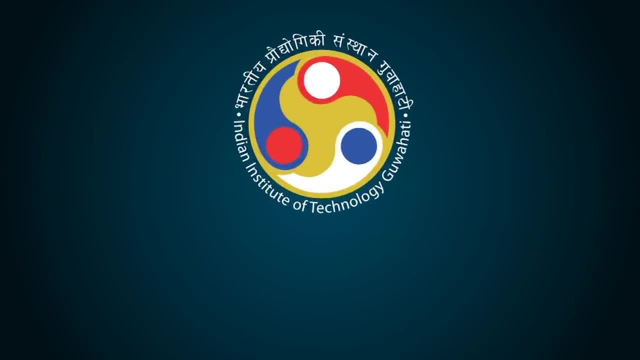 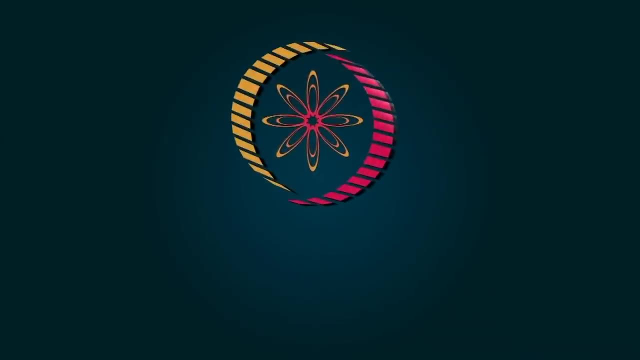 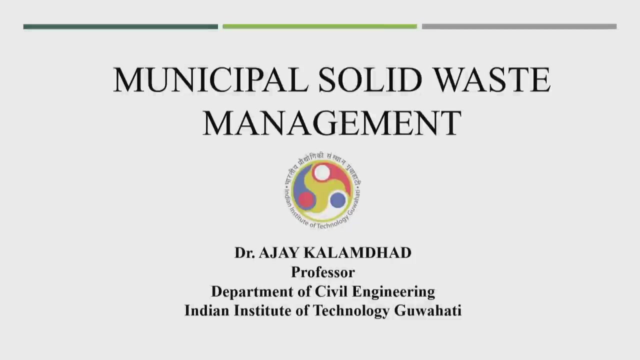 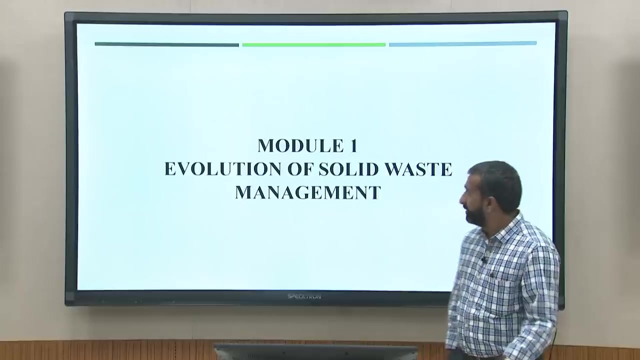 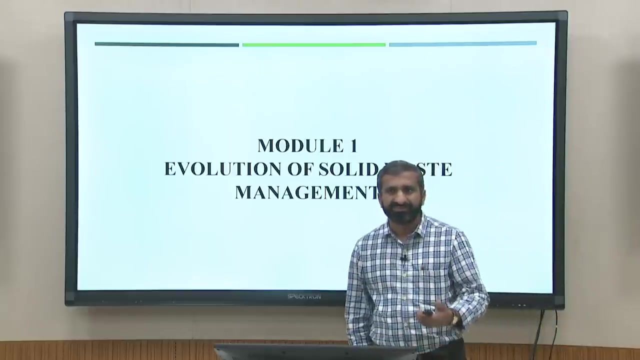 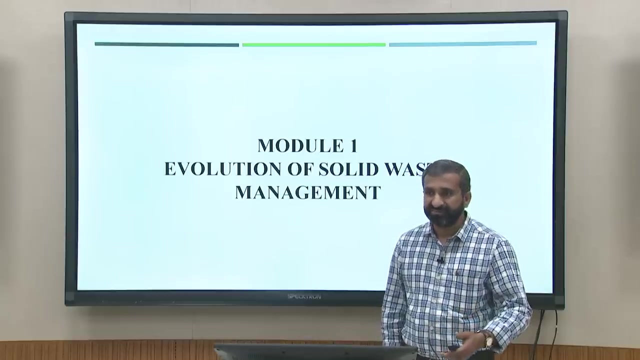 So welcome students for the first lecture that is module 1, evolution of solid waste management. So need to first understand in the in this module or the first lecture, we will talk about the- what do you mean by solid waste? that is one of the very important to understand when you 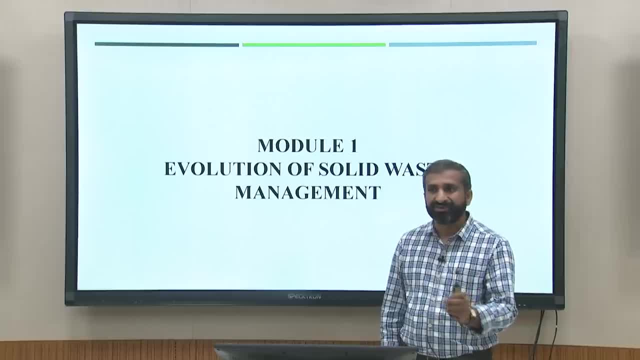 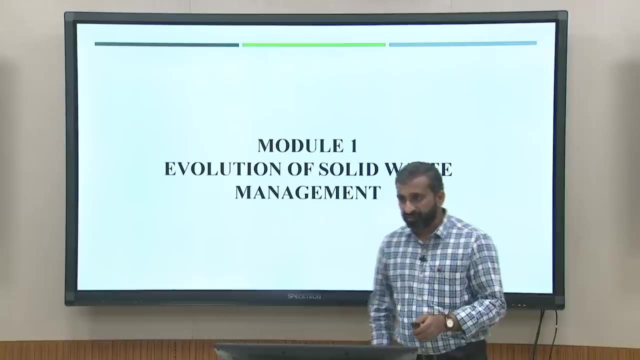 say, the waste is very difficult to understand when you talk about the treatment issue or any kind of disposal issue. Also need to understand how it is very important issue to the residential areas or municipal areas or ULBs areas. So first we will talk about the, the proper definition about solid. 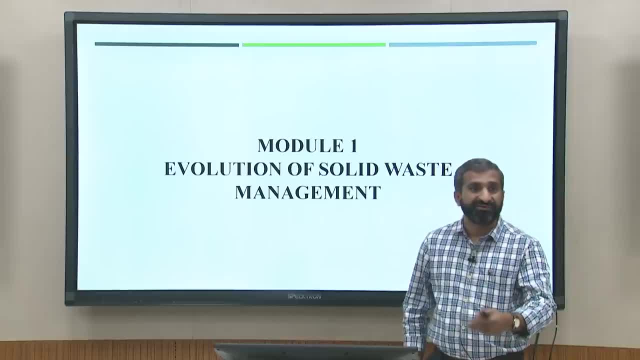 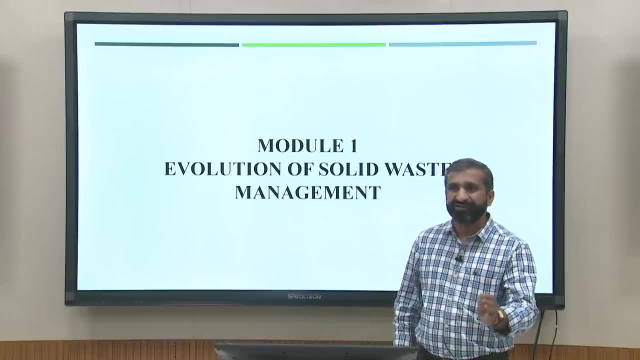 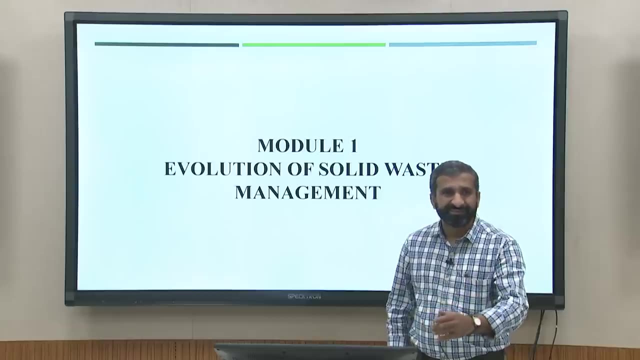 waste, because the problem is that the meaning itself is very difficult to understand when you say any material is a waste and other way we are saying that the waste could be as in waste, or again I think you heard of waste to energy, Or also understood that the waste could be converted, for the compost is very difficult. 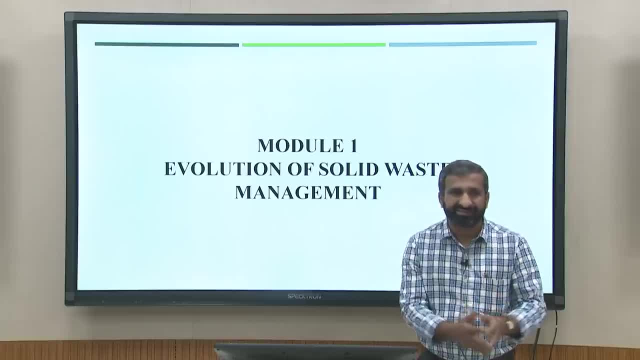 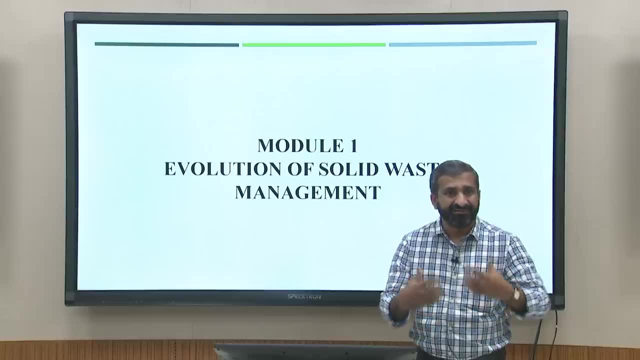 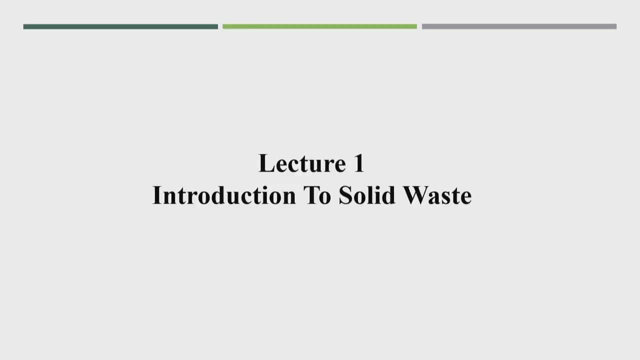 to understand when you say any material is waste is a waste, how you can get benefited of the waste. So name itself is a very difficult to understand giving the proper information. So I will start with the. what do you mean by when you say the solid waste management? So this is: 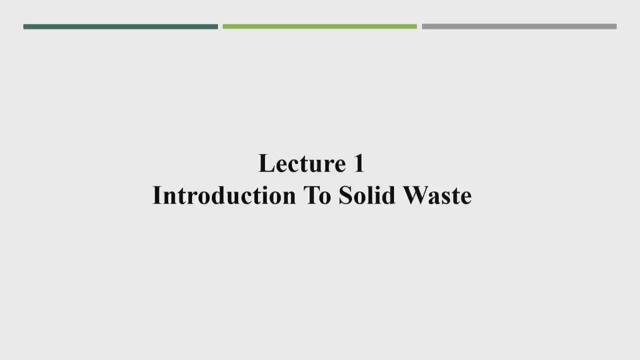 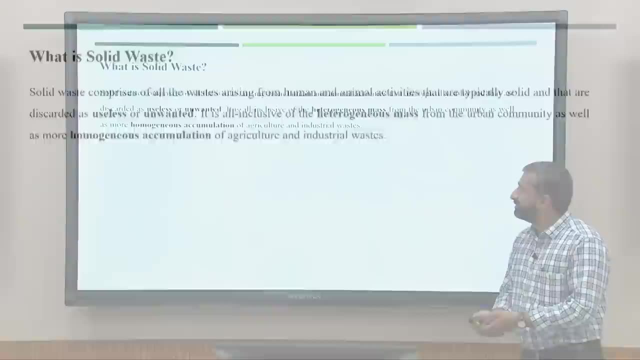 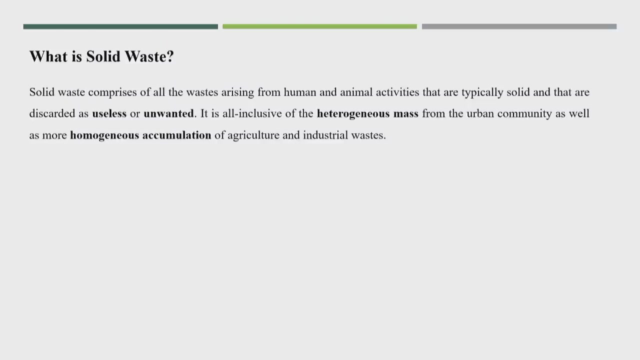 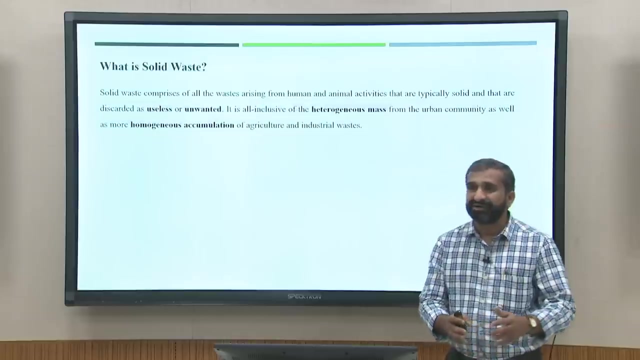 our first lecture on introduction to solid waste. So this is the proper explanation or definition of the solid waste management. So these are: solid waste comprise all the waste arising from the human, animal activities that typically useless and unwanted. So this is the proper explanation of solid waste. See, any material could be. 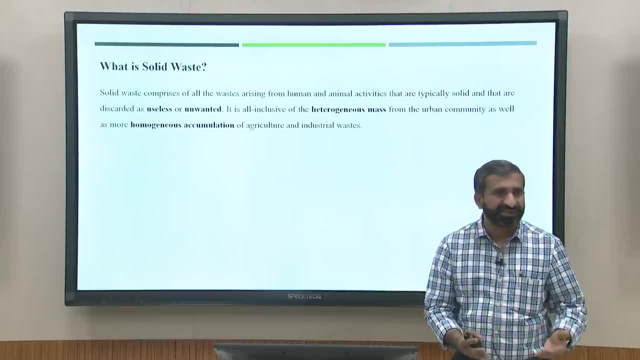 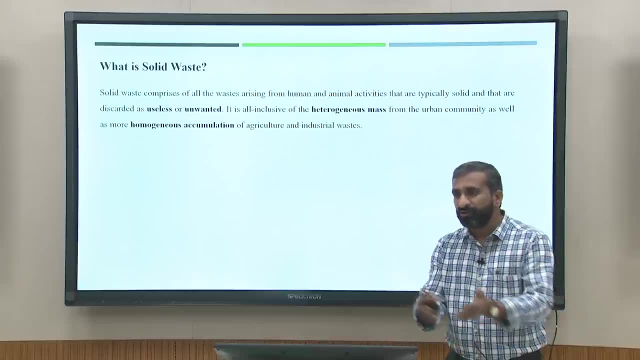 useless or unwanted, that could be a waste material. But when you, when you say that is a useless or unwanted, That for my purpose could be useful or could be helpful or could be produced, some kind of wealth from that same material could be for the another person. So this is the proper. 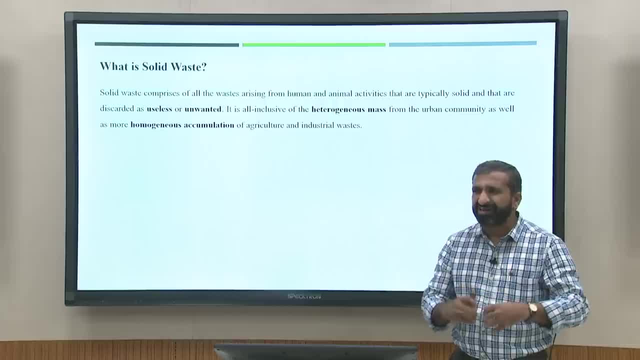 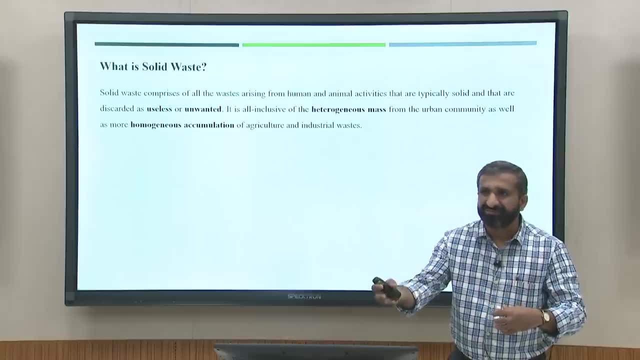 explanation of the waste. But when you say the waste again is very difficult to say that it is unwanted for me. but the same waste is getting wealth for the, some other persons or for other beneficial purposes. So the proper explanation of the waste, So the proper. 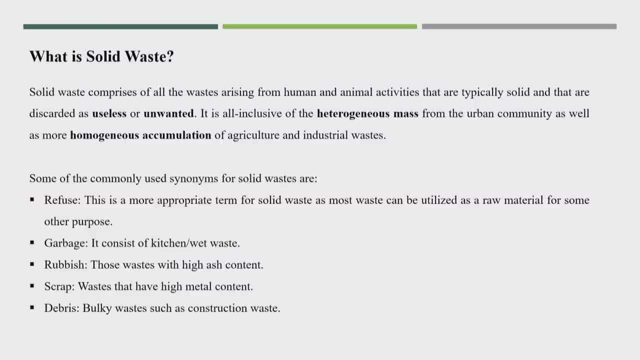 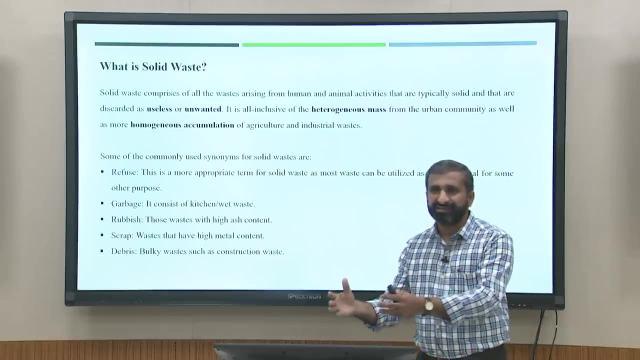 wording. So here this is the word called refuse. This is the proper wording of the solid waste, the refuse, because this refuse can be useless or unwanted for somebody, but the same can be used, as in some of the wealthy material can be produced either as a energy. 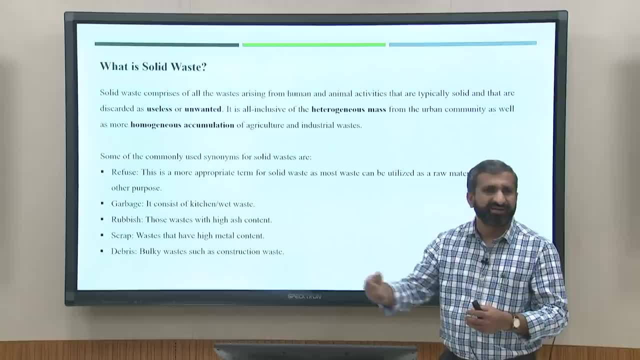 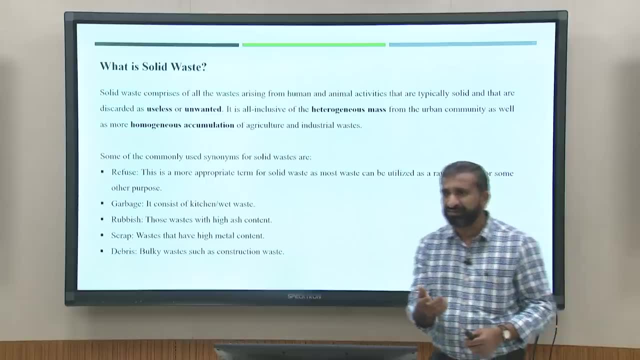 or as a compost or whatever could be or any kind of recycled matter that could be possible. So is a Normally we called as a refuse management. So when you say in the US and European countries mostly they will not talk about the solid waste management, they will talk about refuse. 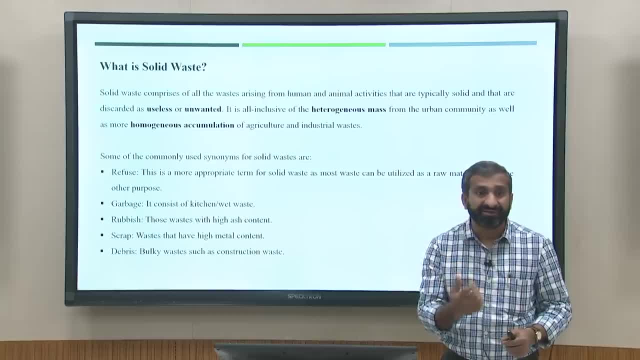 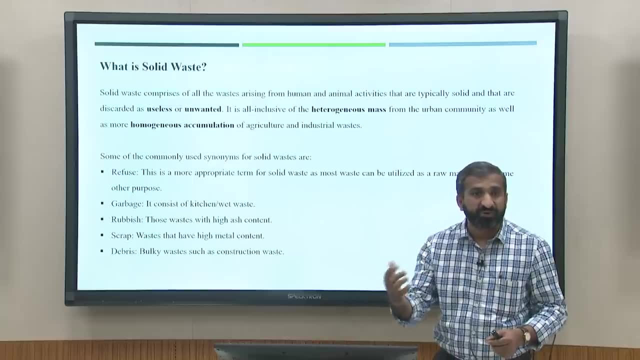 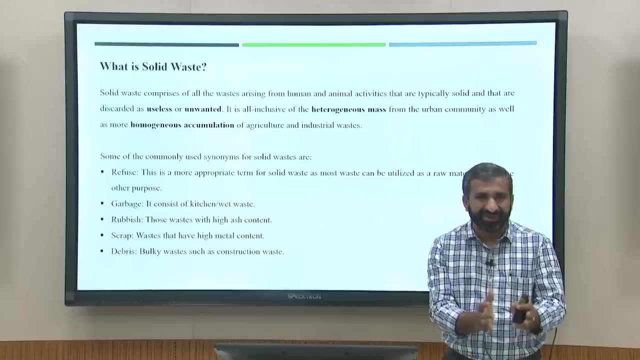 management. That is why they, in their country, they are allowing to use the proper recycling matter to produce the wealthy products like energy, like compost or biogas production, because in India we talked about is a waste, very difficult to accept. this waste could convert as in very 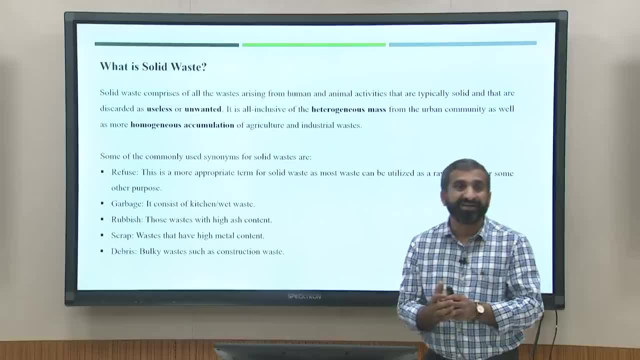 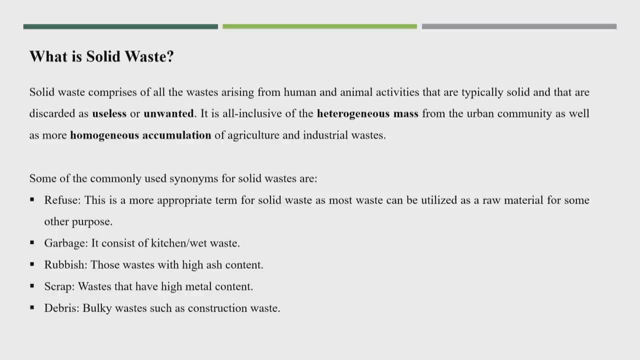 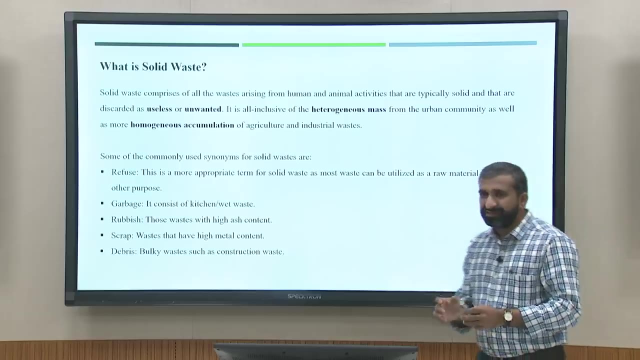 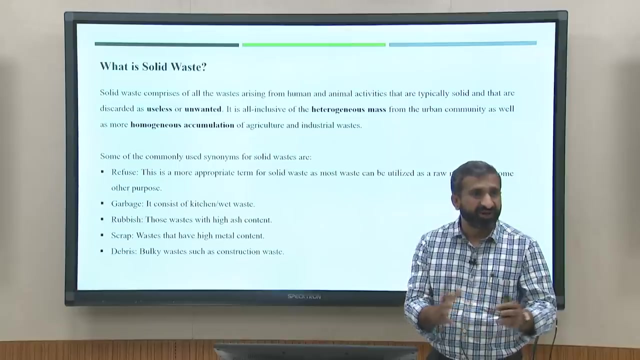 good recycling matter Or could get some well the material out of that. So another word, I think might you know about some few different wordings about solid waste management like garbage. garbage, rubbish, crap and debris is normally the garbage normally we called, as in kitchen waste or wet waste. 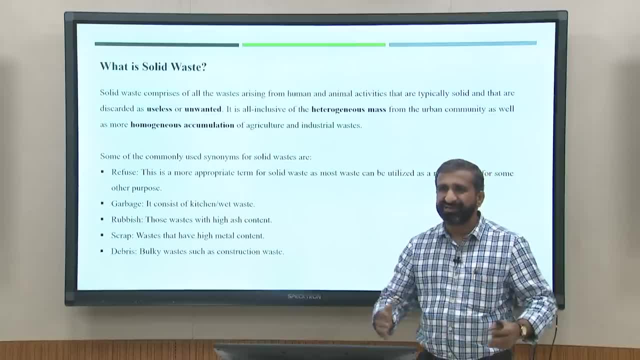 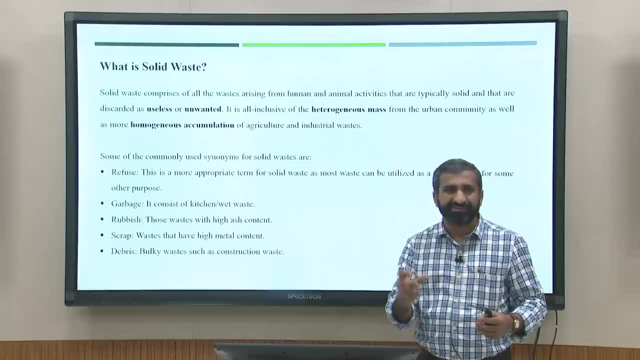 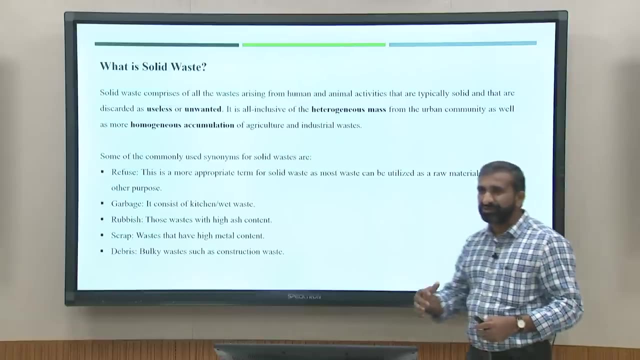 that is normally called as in garbage. So normally in India we talked about the garbage. So this is not the proper wording about this. garbage management is specially targeted to the wet waste or kitchen waste and rubbish- I think rubbish also. rubbish is another management. 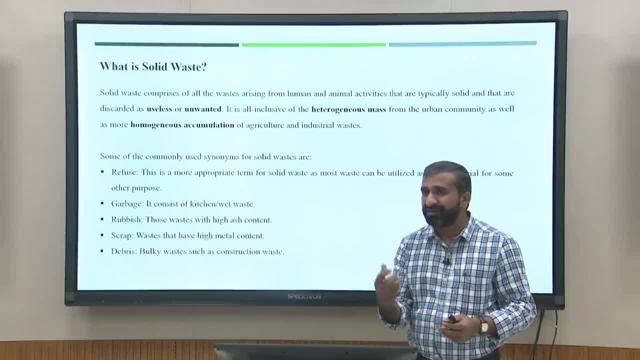 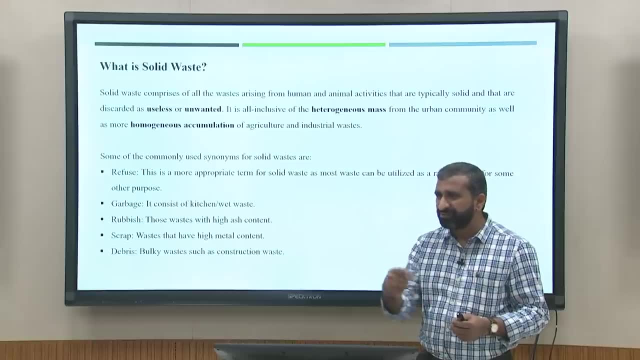 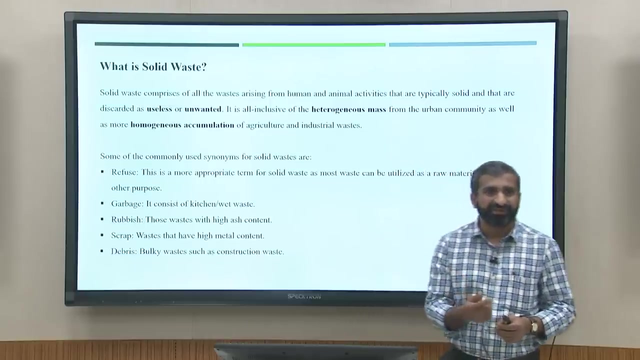 issue where rubbish management, but this rubbish mostly targeted to the waste ash content into the waste material. mostly these kind of rubbish material are producing from the slum area or poor areas where still the cooking is under the simple cooking materials the wood or other materials are. that is producing the lot of ash. 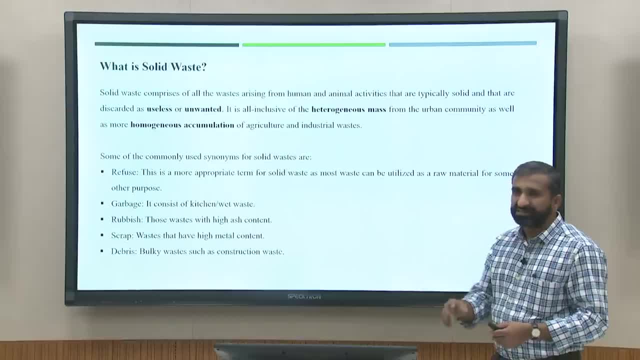 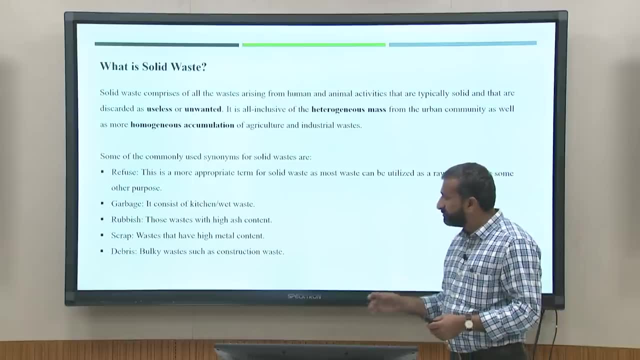 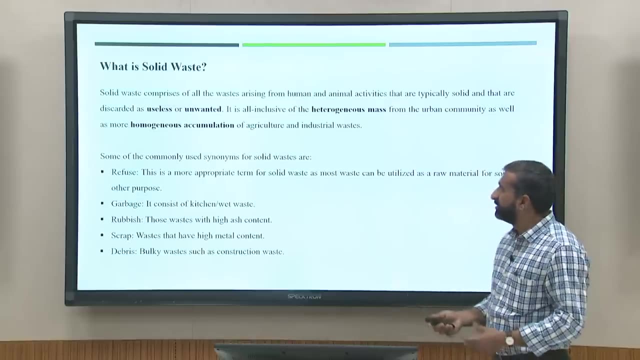 The scrap. this is another word. scrap. that is mostly the scrap is recyclable matter. mostly is a metal is included into that and debris. debris is mostly where the large size materials are including, like construction or demolition waste. So this is proper definition of solid waste. 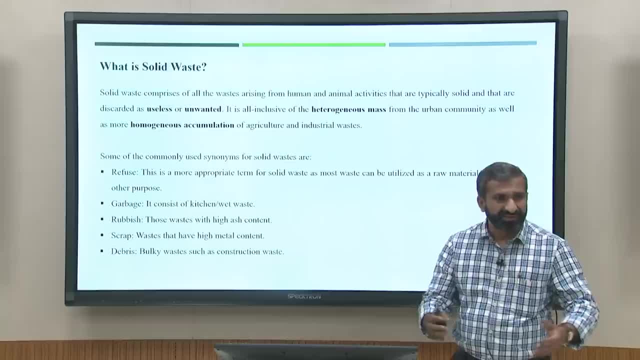 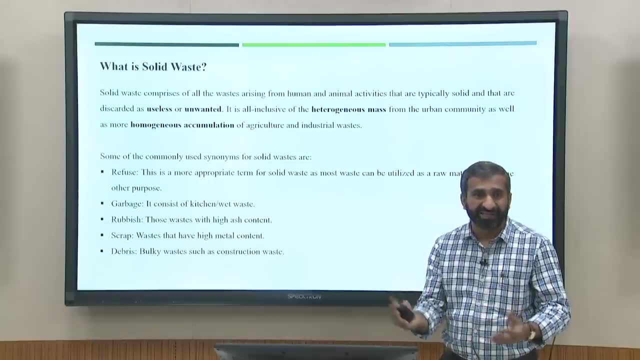 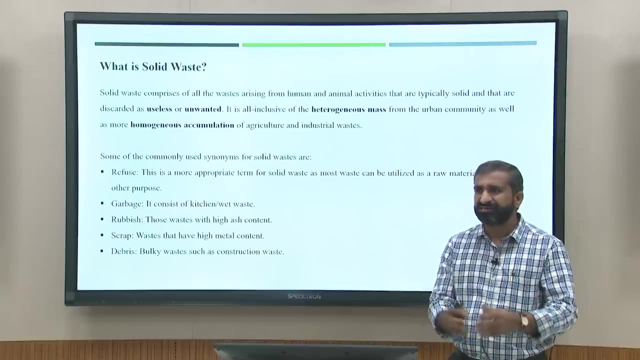 So do not get confused about wherever I think you will study that is a solid waste management or garbage management, rubbish management or scrap management or refuse management. So almost is a similar, just based on the different sources or based on the different characteristics name. we can give it to the waste. 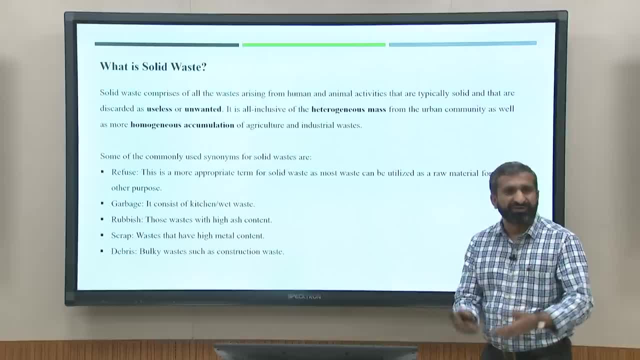 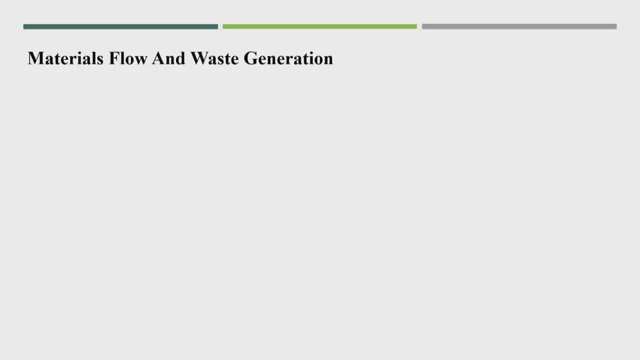 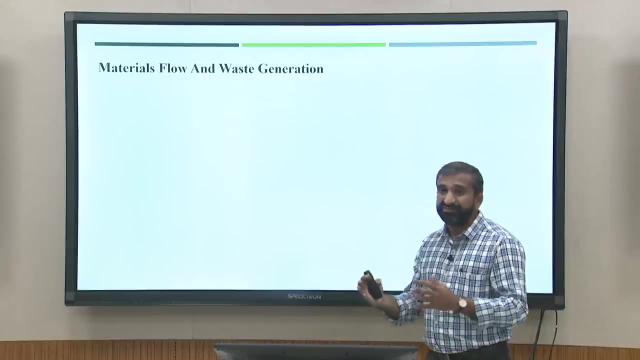 But normally we call it as a solid waste management for all kind of different characteristics of the waste material. So now the very important one, the while producing the different material, or specially for the manufacturing of any material, how this is related to the waste generation. that 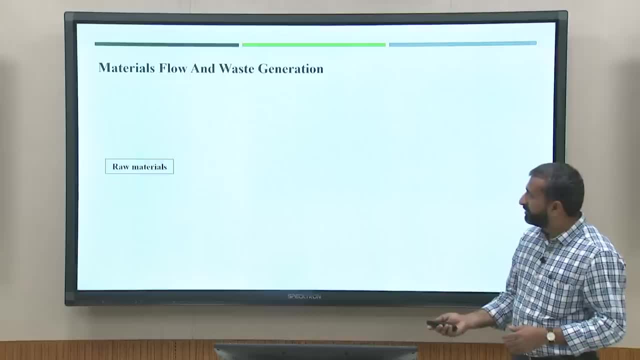 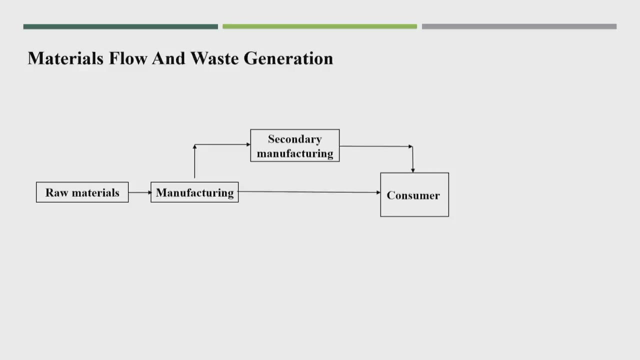 we can find. we will see with the one flowchart, like, suppose some raw material we will take for the any manufacturing of new product. So manufacturing will go. maybe is a primary manufacturing, secondary manufacturing and we will get some kind of product that will go to the consumer. 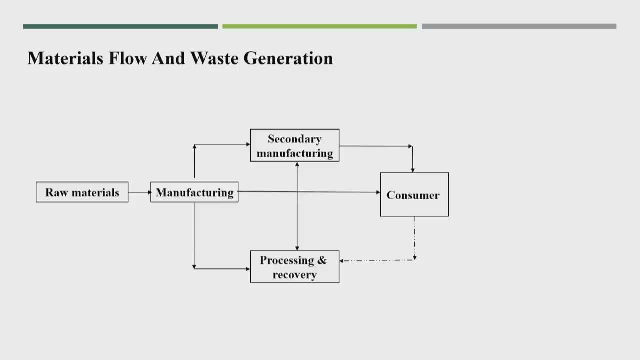 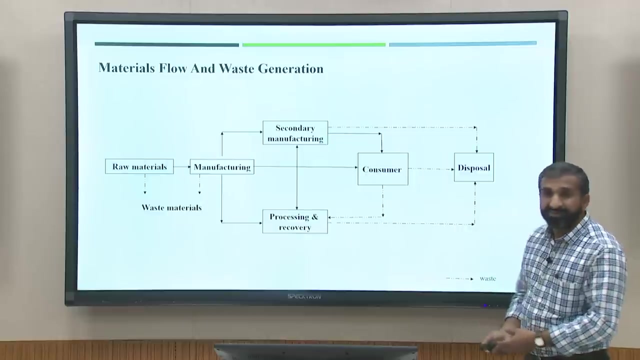 And from consumer again. suppose we plan for recycling facility or recycling of the same material. it will again go for processing and recovery and go to the manufacturing process. But entire these material flow, you will see the lot of waste production. So is under the raw material. you see the lot of waste production. 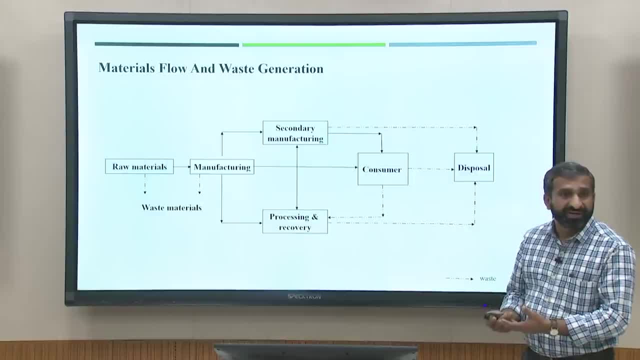 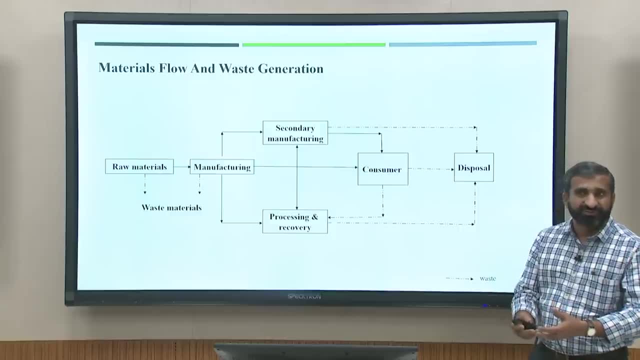 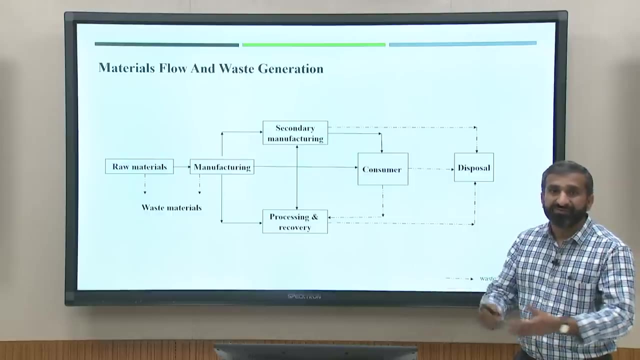 So it is clearly explained that. and again, once the consumer will use that particular material, again after entire utilization of the material, it will go for the disposal site. So it became waste. So the entire flowchart is showing that if any raw material is getting manufactured and 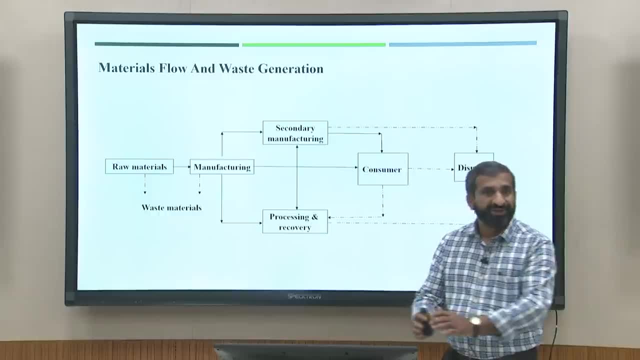 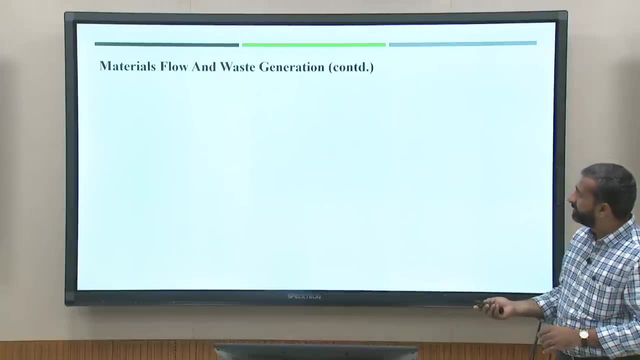 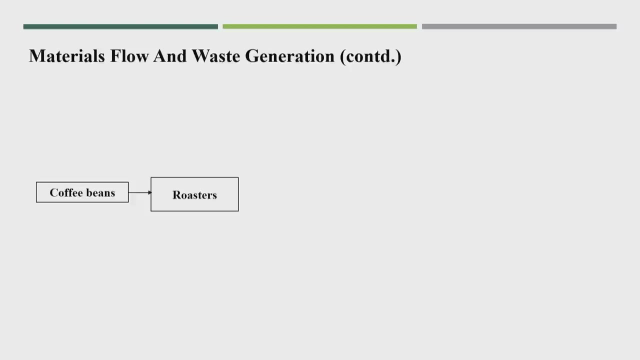 to manufacture to the consumers Also is related to the waste generation. So, similarly, one example: this we can understand by one example, by: if you take the coffee beans and these coffee beans, normally when you prepare the coffee, that powder it need to be go to. 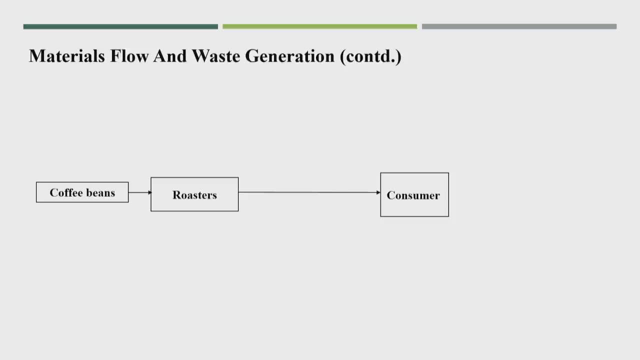 the roaster and finally, after getting roaster, that goes to the consumer. but sometime the roaster beans also become a coffee powder. So these coffee beans become a coffee powder and will goes to the consumer. This is the entire use of the coffee beans to become a coffee powder or direct roaster. 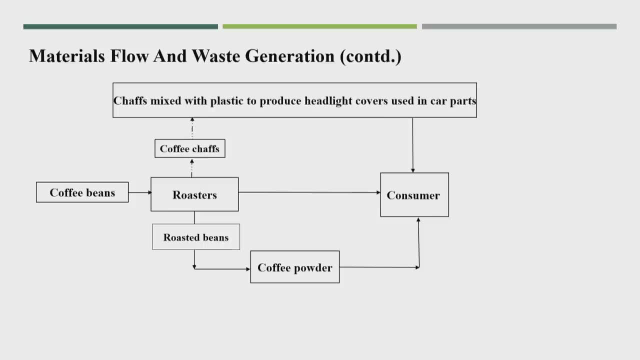 to the consumers. But now again from the roaster. there are lots, of, lot of coffee chops is getting produced as a waste material. These waste material also can be utilize. can be these waste chops? mixed with the plastic to produce covers used in the car parts is again getting utilized. 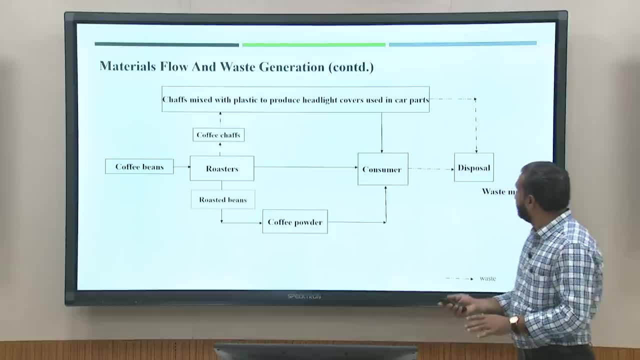 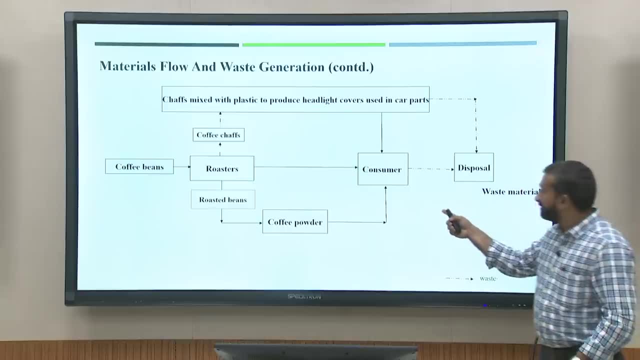 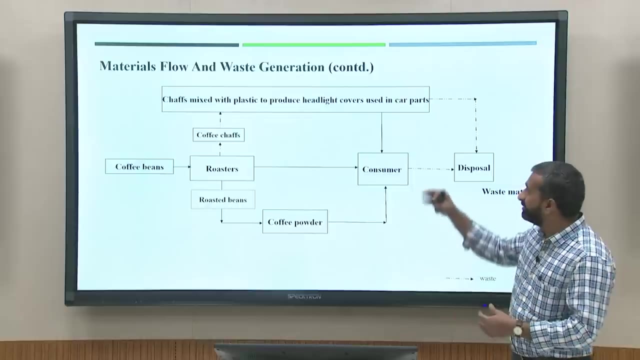 So there will not be any waste material production. But again this material is again getting disposal because once you prepare the coffee to that coffee powder also is became a waste material and whatever the remained material while in the roaster, that also will go to the disposal area. 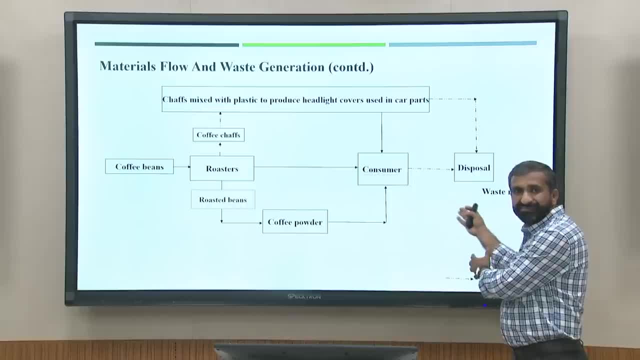 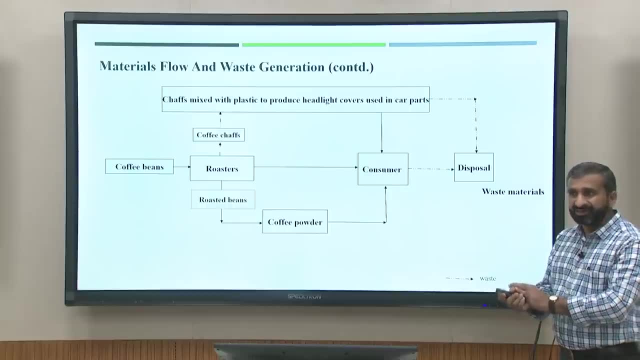 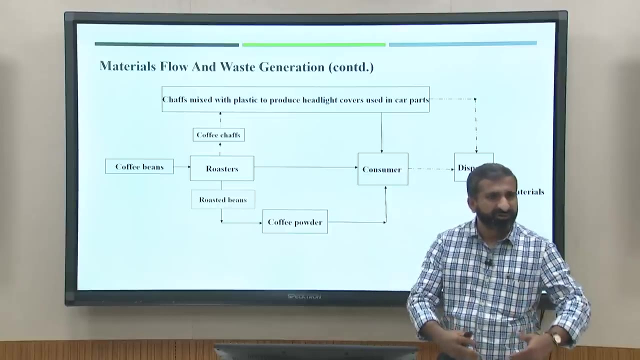 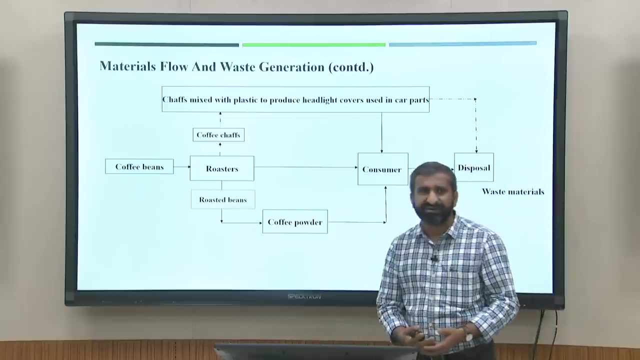 And ultimately entire coffee beans or whatever the after utilization it became the waste material finally. So it is clearly related that for any manufacturing or for any, whatever products we are using for our daily activities, So these all products is including the waste generation. okay, So is very easily understandable. now, waste generation is very important because, whatever 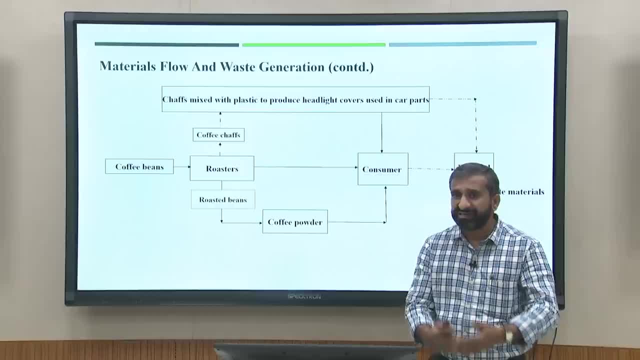 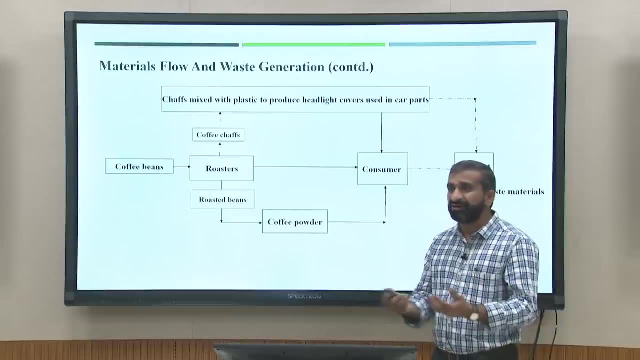 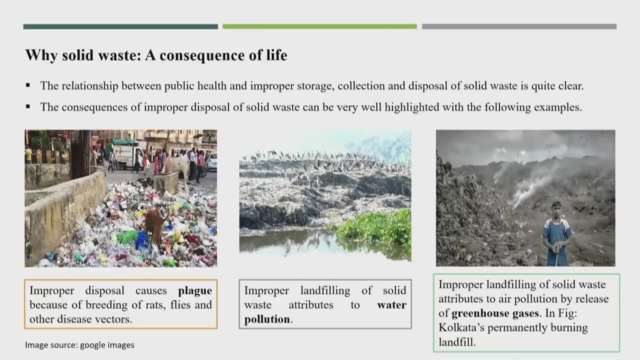 materials, your daily activity, you are using the same material will get finally getting disposed as an waste material after the entire utilization of the that particular material. So we will see that how the solid waste is related to the, to the or consequences of the life. You will see that there is a proper disposal of causes. the plague is a. you know the Surat. 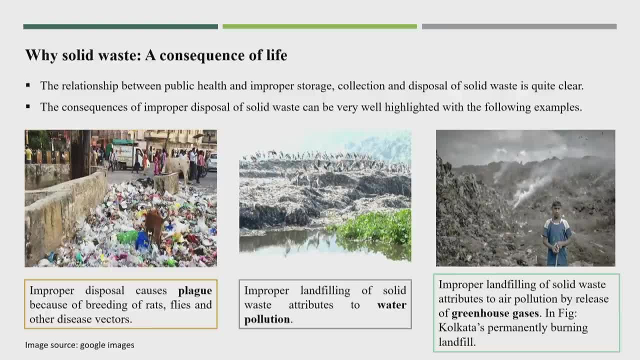 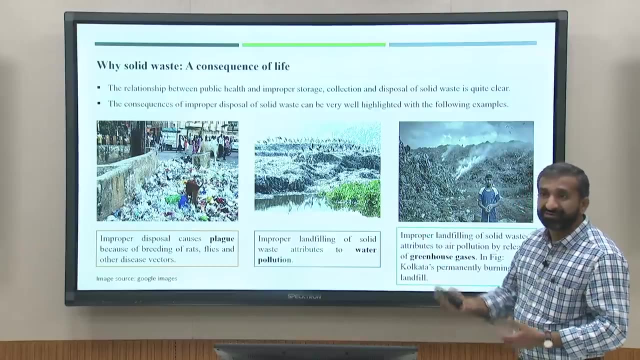 plague is very well known in 1983, where a lot of people have died because of plague issue. So that is clearly shows that if you are not able to dispose the proper solid waste, how is is your life is getting affected. You see this. 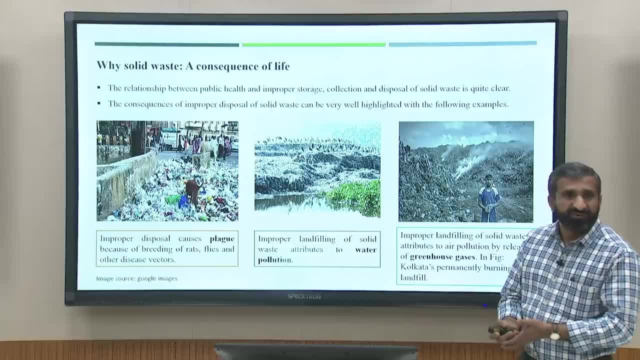 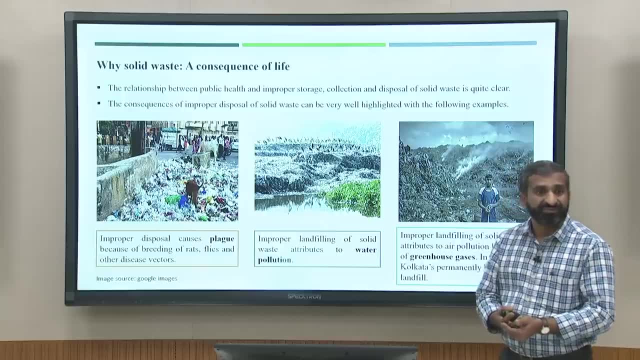 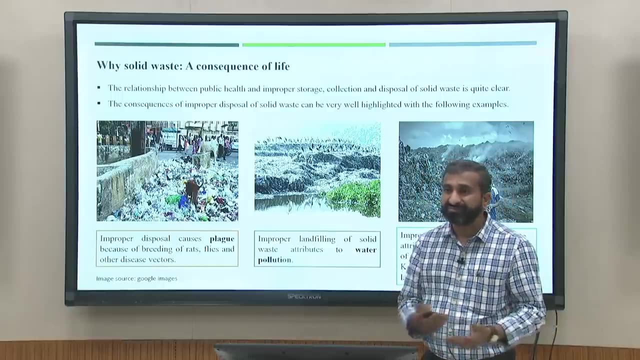 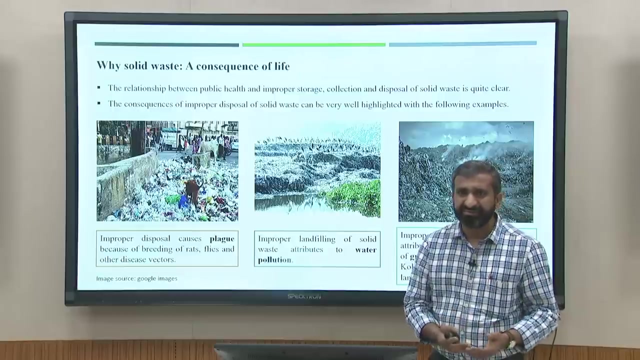 The, Yeah, The land filling, the way we are disposing the, the solid waste, is become a very important issue for the water pollution. So because of that, not only the surface water but also the ground water is getting polluted because of improper disposal sites, and in India mostly the waste is getting collected. 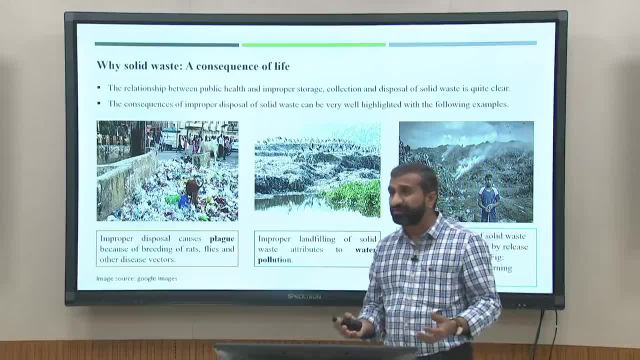 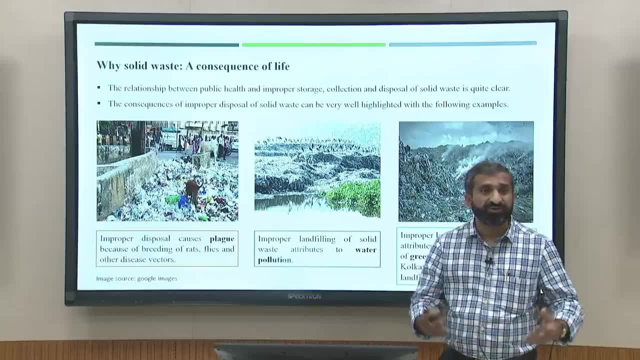 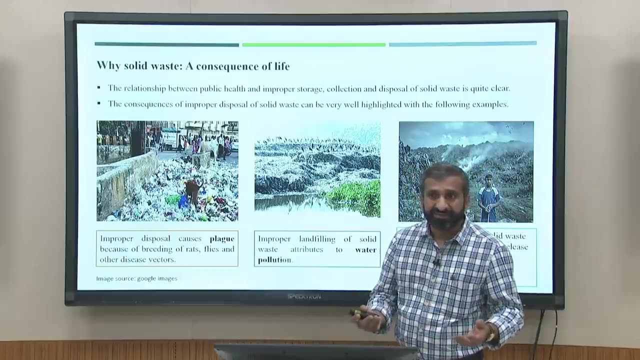 even under Swachh Bharat Mission, The major target was to clean the city. Okay, And from 2014 onward, most of our city is getting cleaned and where number of cities are getting awarded also because of cleaning, But I think we never talked about once the any way any city is getting clean means entire. 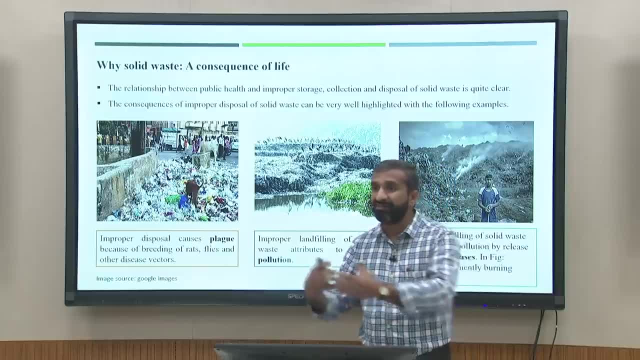 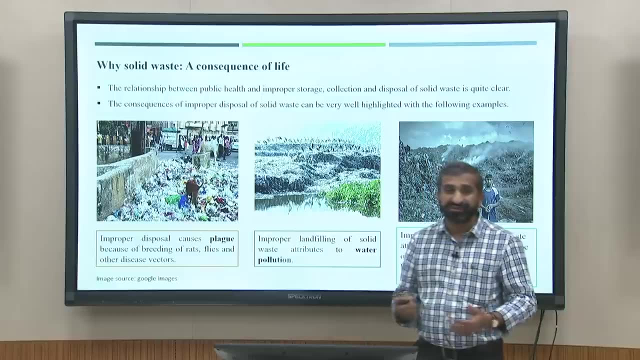 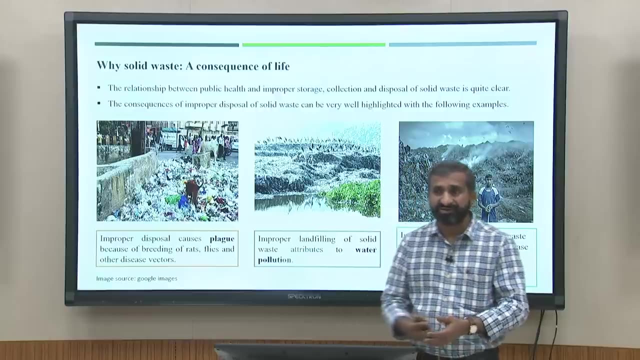 waste is getting collected, but how best they are able to dispose of and the way the waste is getting disposed of in low lying area in most of the cities. are these kind of issues Okay? The water pollution issue? similarly, if you, and especially the cities, like the cities, 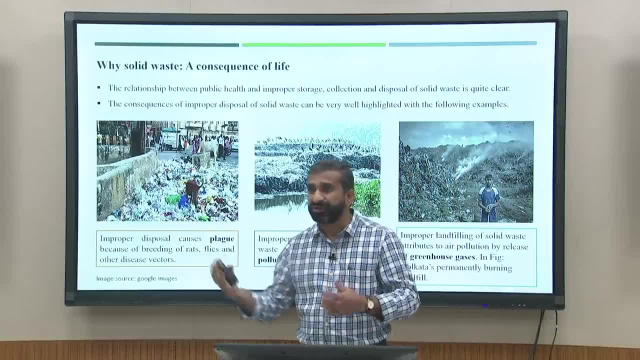 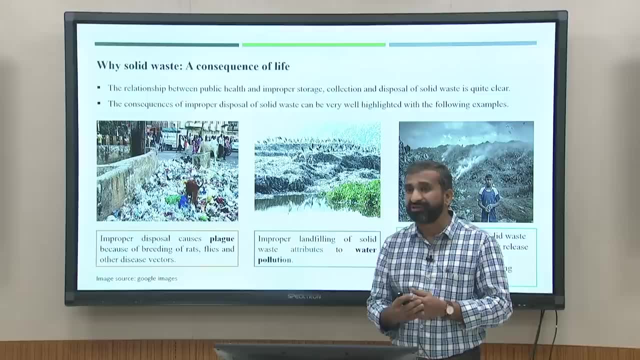 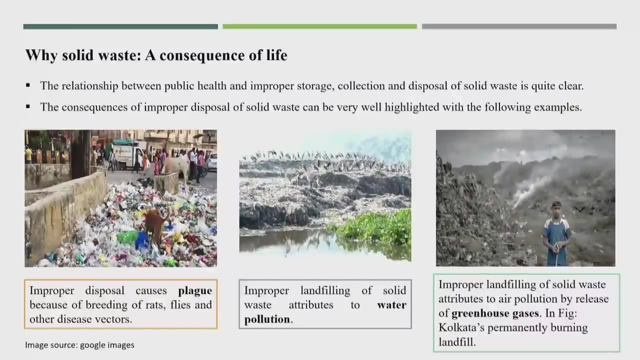 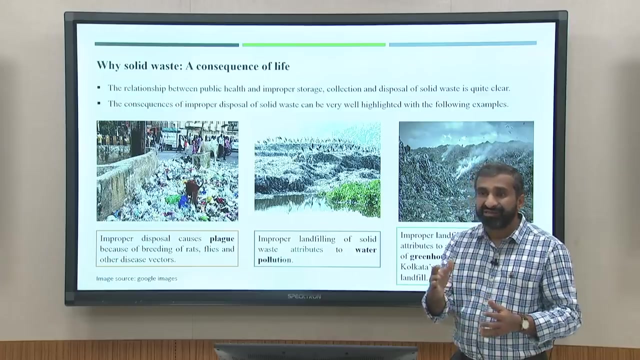 very close to the any water storage area or somewhere near to the wetland areas are very difficult to have the proper disposal system. See somewhere here also the greenhouse gases, because once is once the entire mixed mixed waste is getting disposed of, So one location there is not only the leachate is getting produced, while degradation of biological 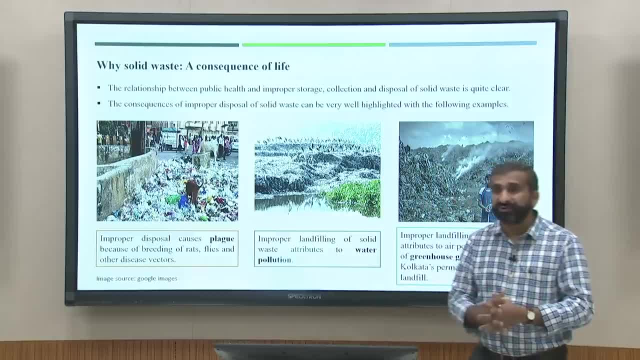 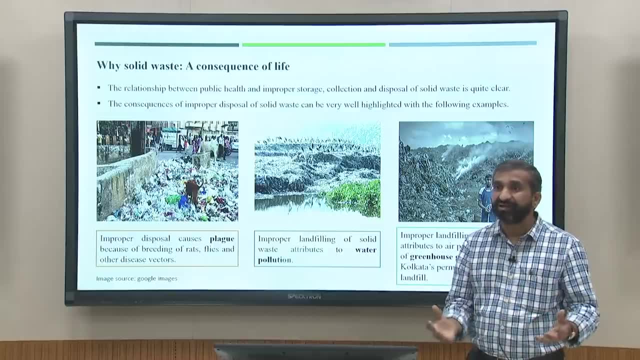 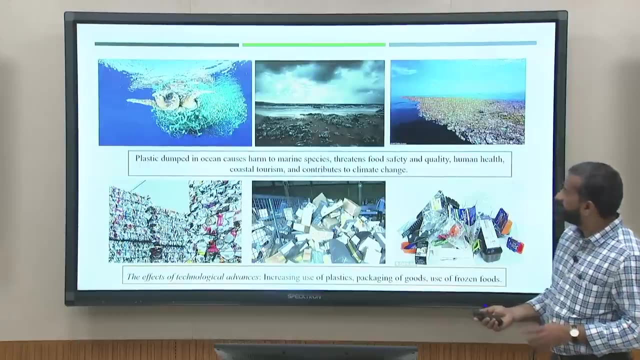 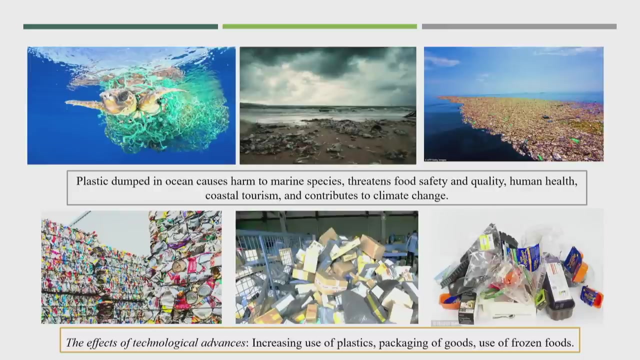 waste also, the greenhouse gases also will get produced. these greenhouse gases, including carbon dioxide, methane, these gases will get produced and this is polluted the local, local area- See some of the photographs are here: Might. This is the one photograph, like the the way we are disposing the plastic into the sea. 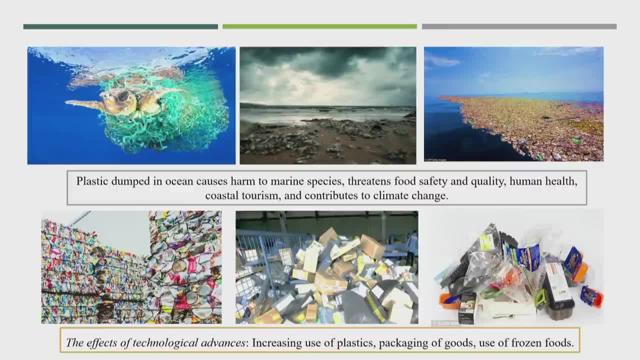 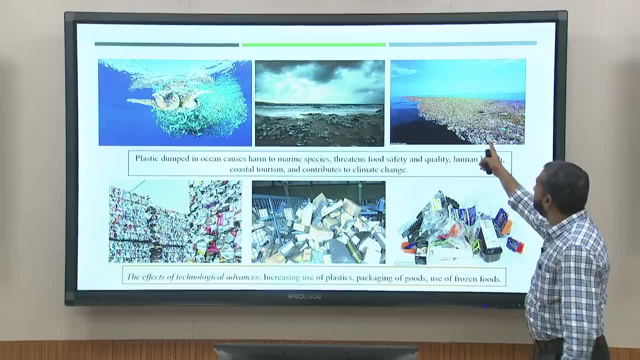 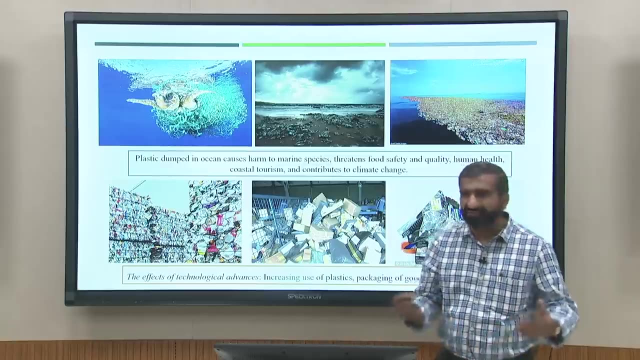 how these marine species are getting affected by the these plastic disposal into the sea. See the. this is the one photograph you can see, because the plastic is not getting degraded and is getting floated onto the water and somewhere is getting stored in a very large quantity. 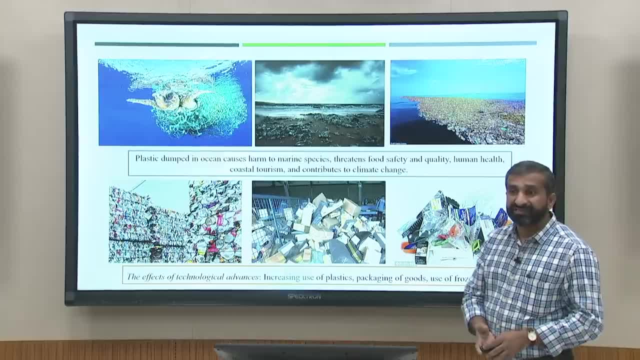 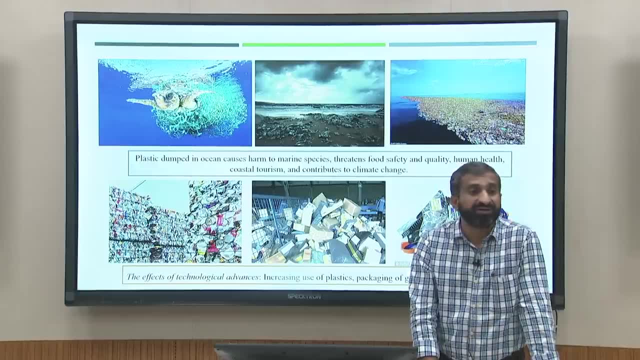 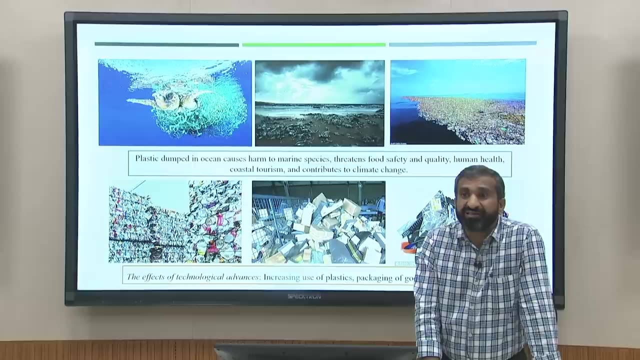 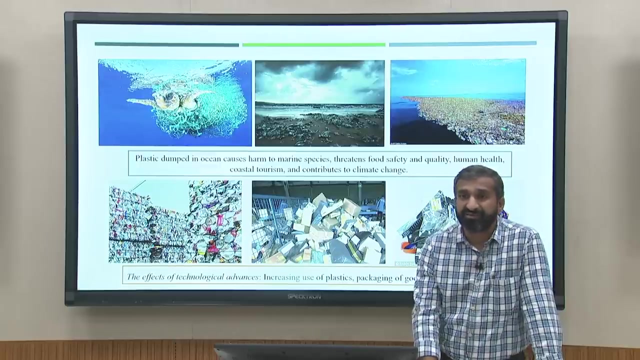 And also the because of technology, urbanization. Now see the. before 20 years or 15 to 20 years, India never talked about the packaging material. Now, because of this online purchase, had increased lot of waste production. that, especially the packaging waste, see, I still remember in our older days when you go to somewhere into the. 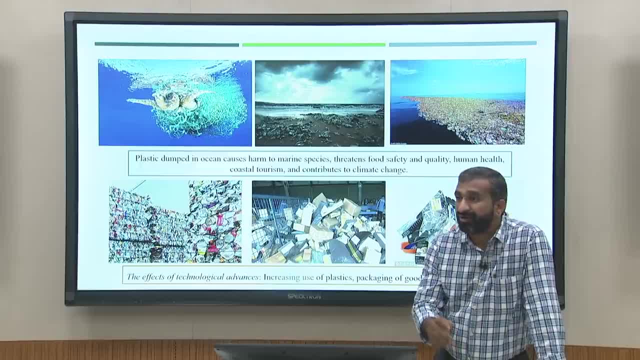 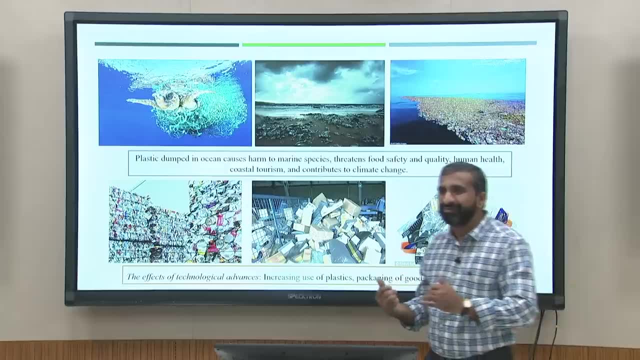 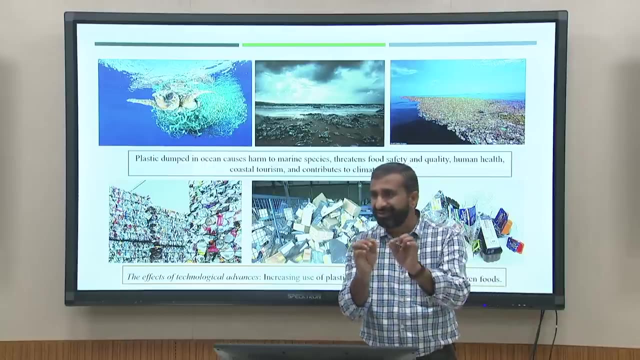 shop. See, We never used to get lot of packaging material. most of the material is getting packed into the newspaper and easily. we used to collect with the bags, But now I think the way our product is getting sold off, that is based on the package. 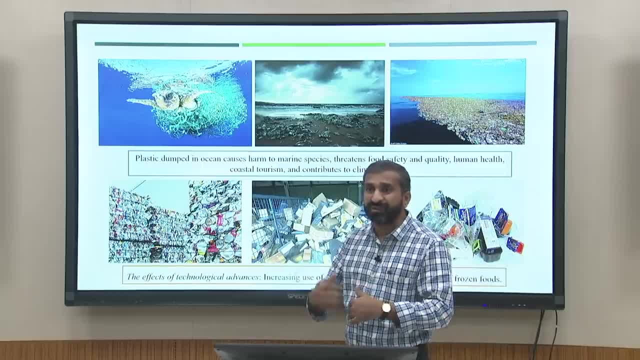 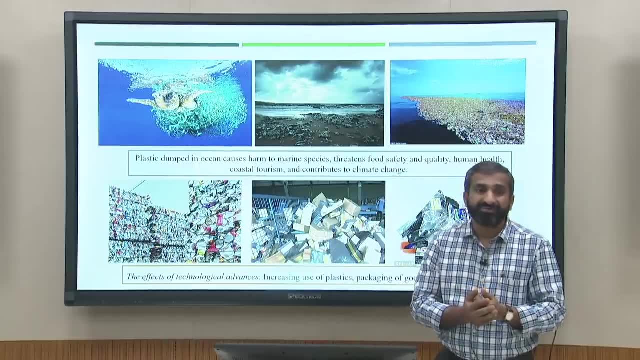 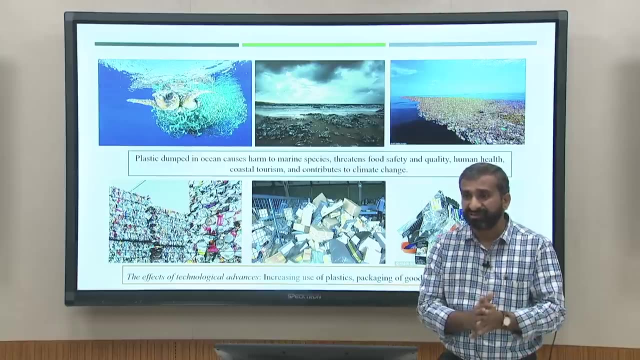 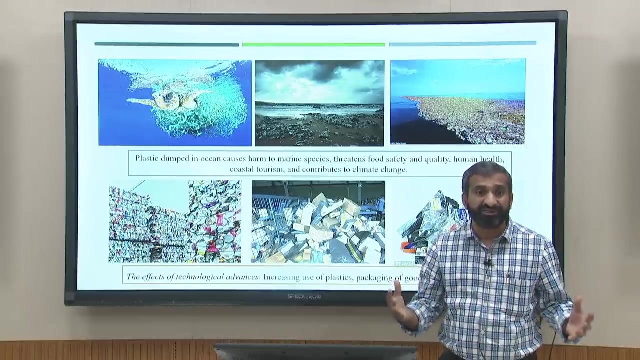 And because of this online production, large amount of paper, large amount of plastic is getting included into the waste management. Okay, Okay, the important issue now: see earlier, India always used to talk about the vegetable waste or biological waste is producing more, But now, if you see the entire waste compositions, now we are getting large amount of paper and 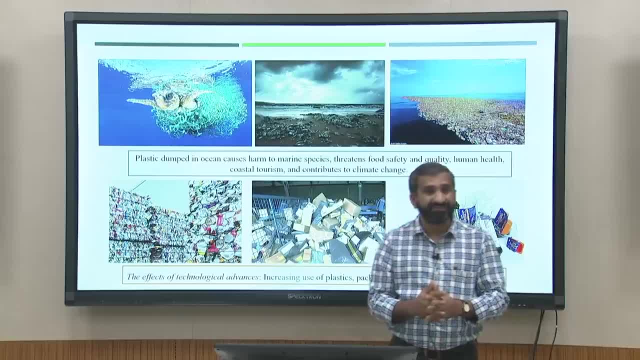 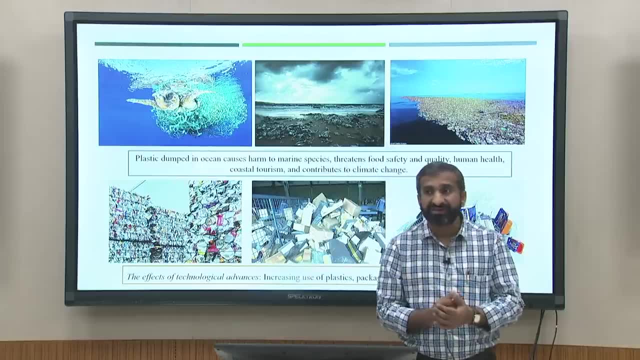 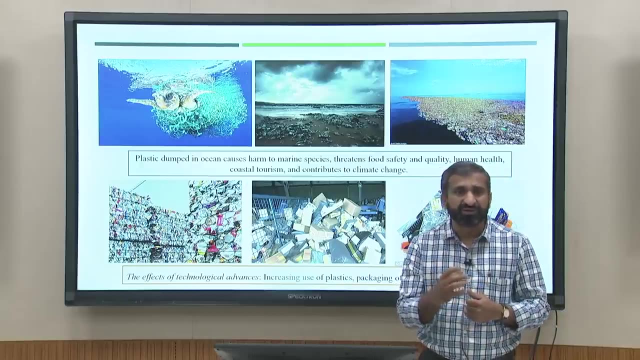 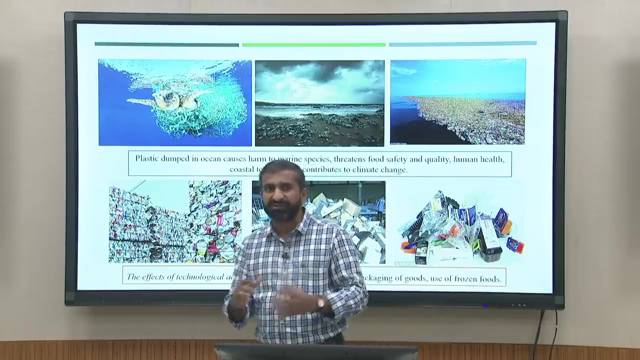 plastic that is not degradable but is more recyclable. matters are coming up. So you see that the solid waste management, the very another very important one, this waste is a heterogeneous in nature, highly heterogeneous. Now see, you understand this heterogeneity, like if you just compare with the water treatment. 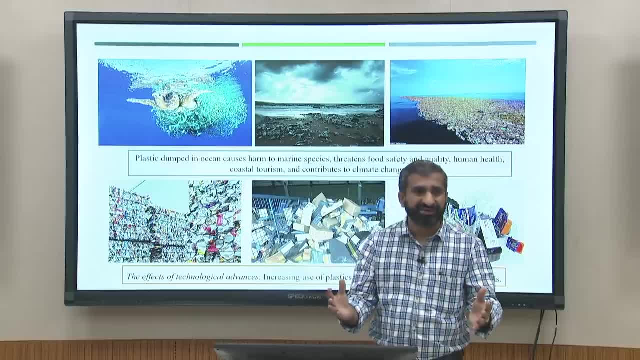 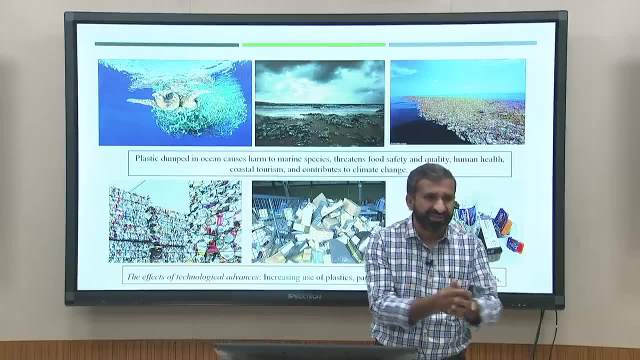 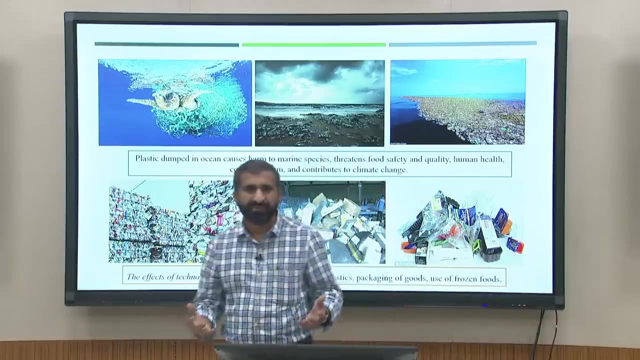 or wastewater treatment. So water is a homogeneous material. you take the water from, whether India or European countries or American country, water quality is same, Except maybe some pollutants will get changed. So your treatment also will be almost same. these all treatment facility, your sewage also. 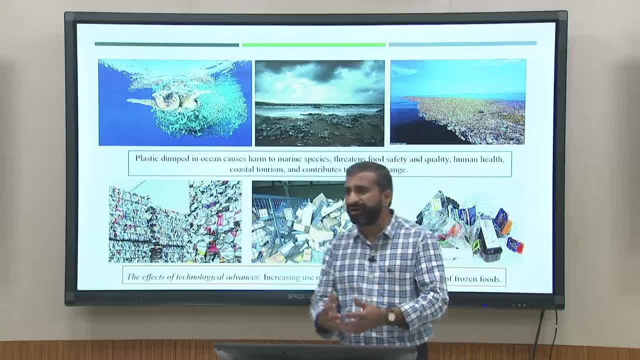 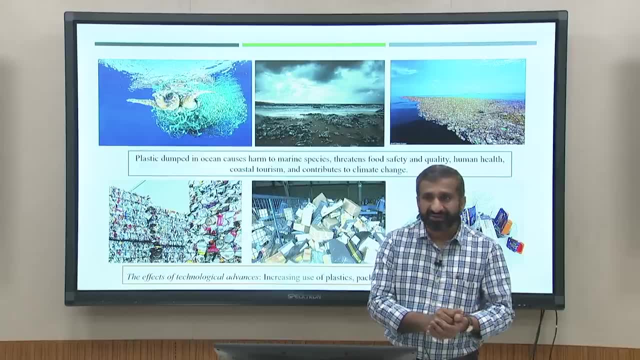 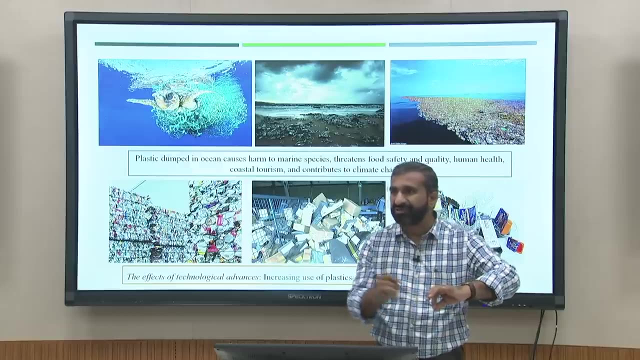 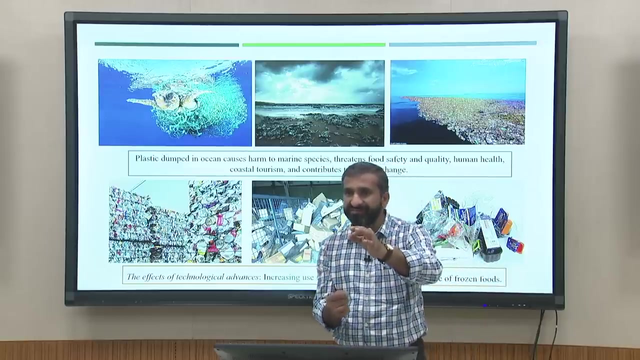 characterization will be the same. So your sewage treatment plant also will be the similar kind of sewage treatment plant will design, But for solid waste. now, the, it is a entire heterogeneous mass, even in the every day, also, the, your entire composition will change. So, like you see, the, your daily activity on Monday and daily activity on Sunday. both are 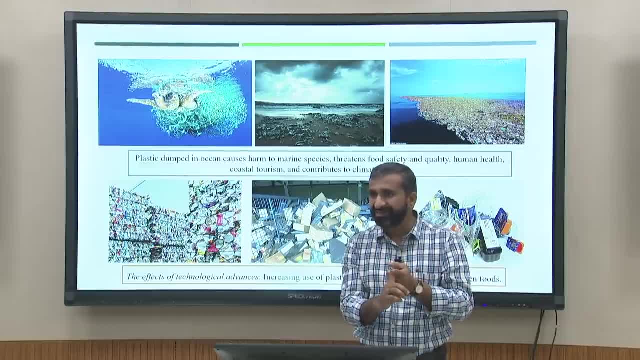 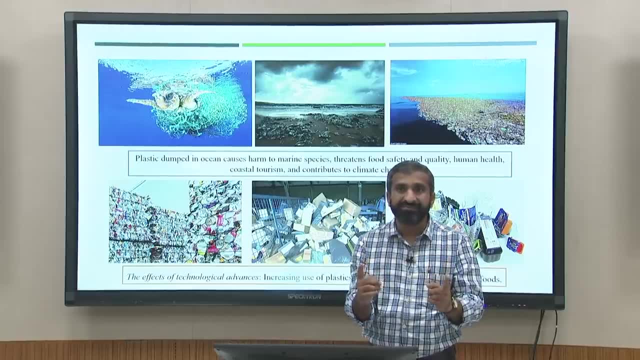 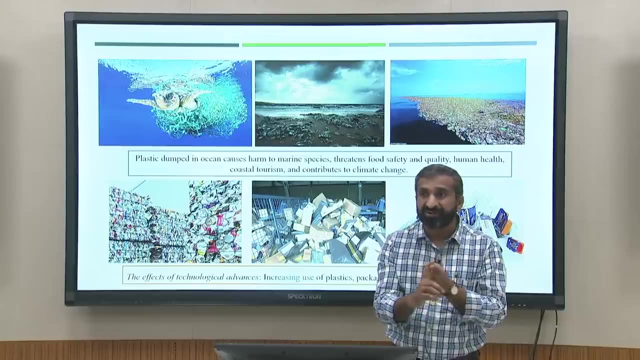 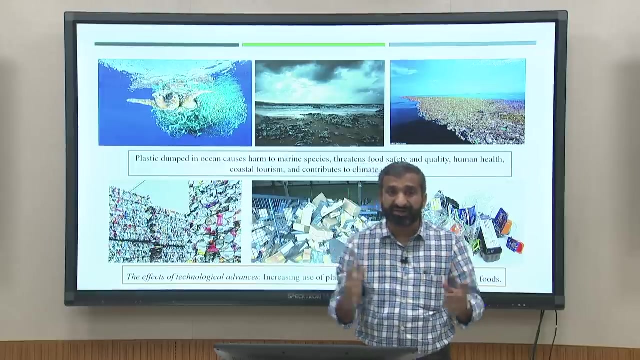 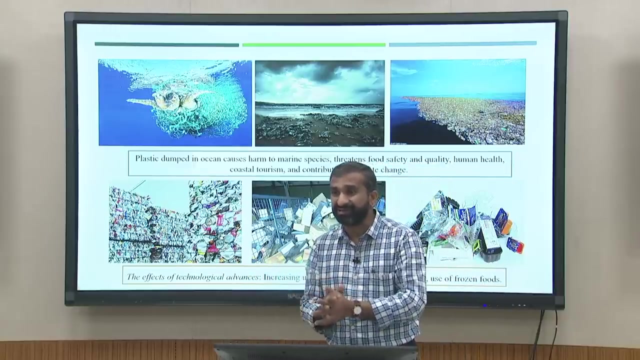 different. So activities are changing. your waste generation also will change. waste generation not only the quantity will change, but also your characteristics will change. So someday you will produce large amount of biological matter, someday you will produce large amount of recyclable matter. So So it is very difficult to have the one kind of proper technique or any treatment facility. 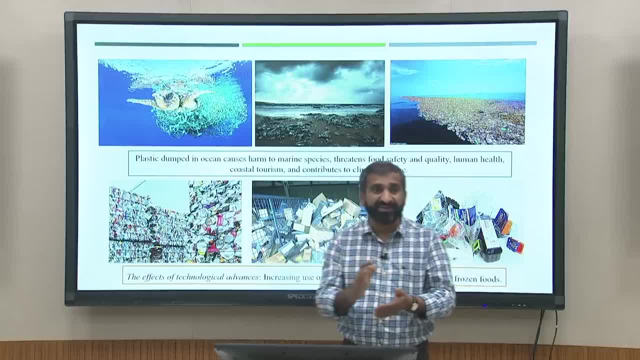 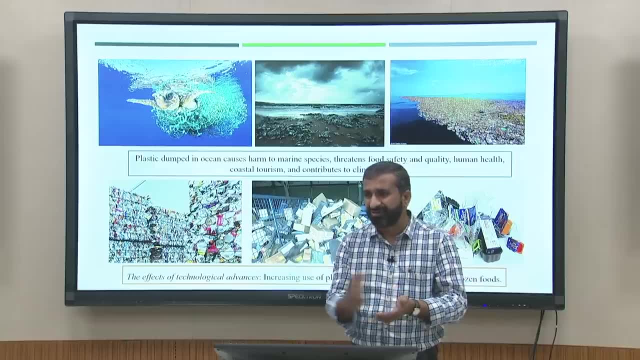 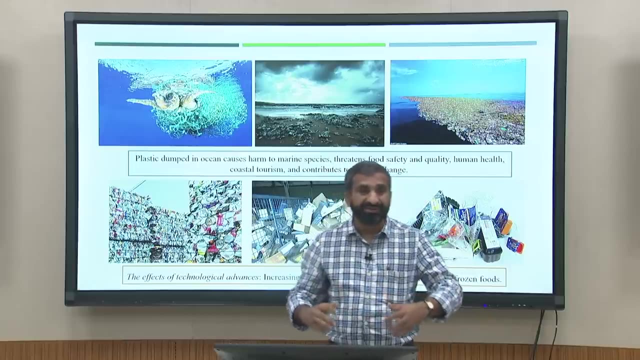 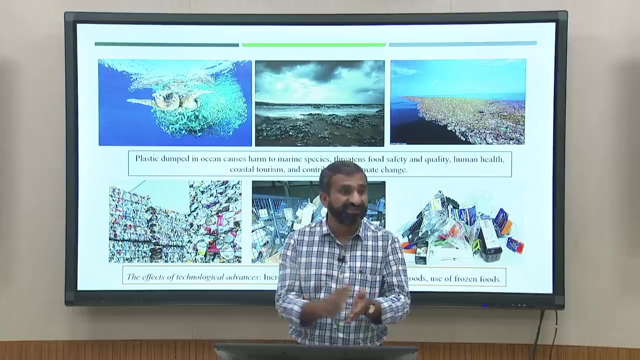 And also these characteristics also is changing with the area to area and season to season. that is another very important issue. like when you take the, in India we have three different seasons, So obviously your, even your food habits also change with the, So change with the season. like in the summer you will not get a lot of vegetables, but in 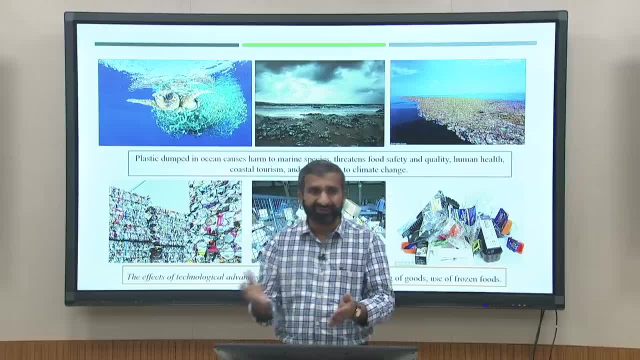 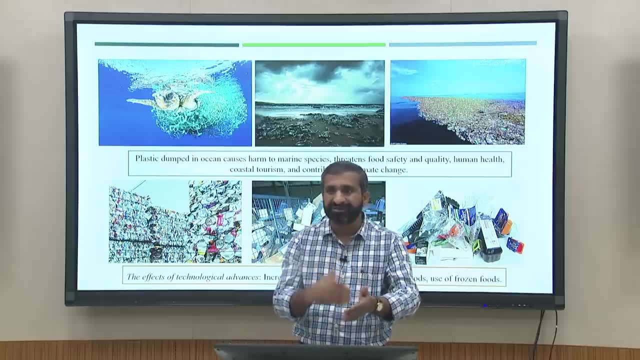 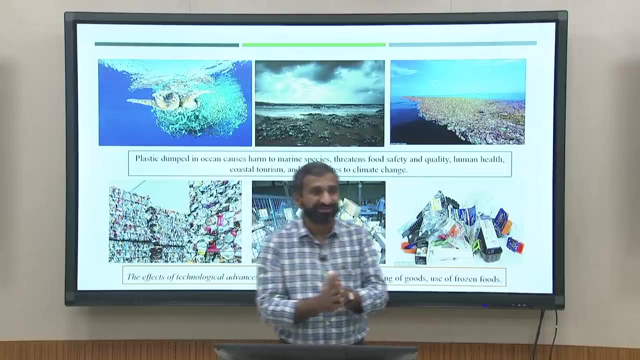 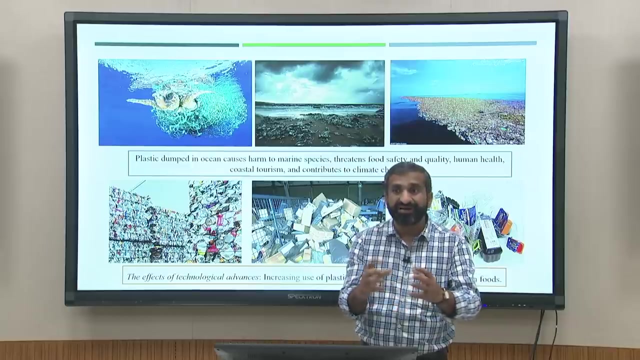 winter we will get a lot of vegetables. So obviously your vegetable waste will be more into the winter season and your dry waste will be more on to the summer summer season. and again you see the monsoon. again we have 3 months monsoon, So the technology should be such a way that it will. is very difficult to find a simple. 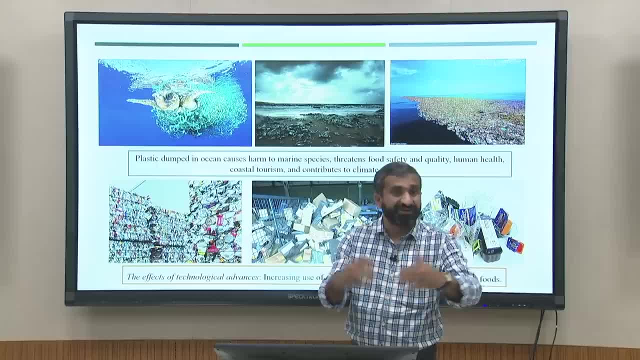 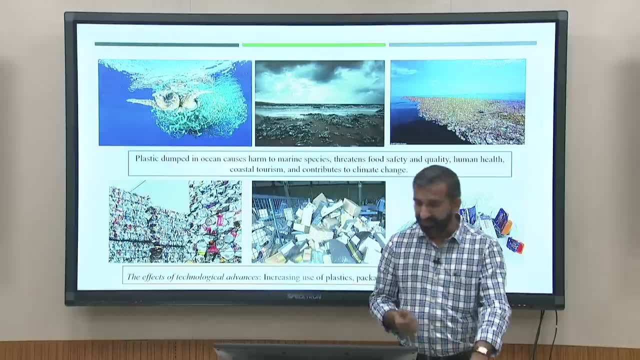 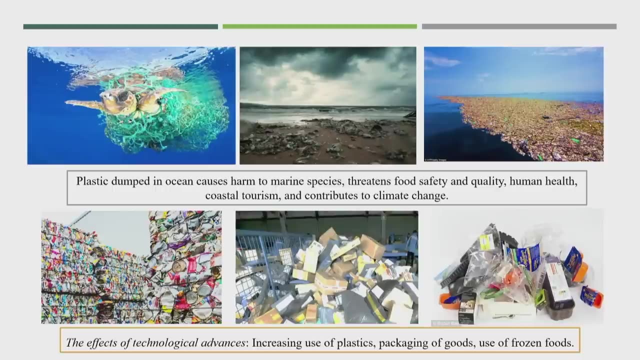 one technology where the dry waste, wet waste, different compositions, can be treated at one location within the different season. that is one of the very important issue in the solid waste management. But now the way our commercial or urbanization is increasing your waste generation is also. 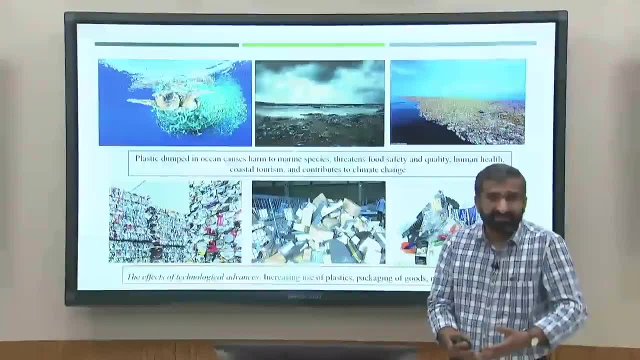 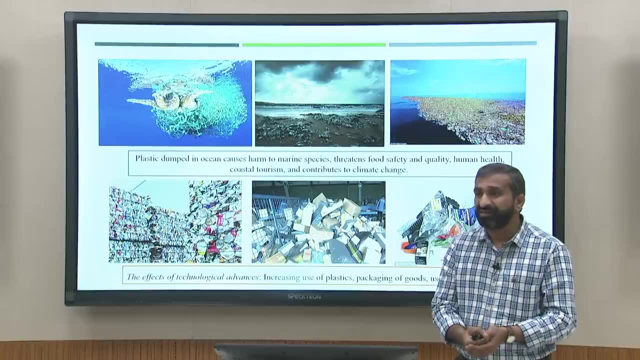 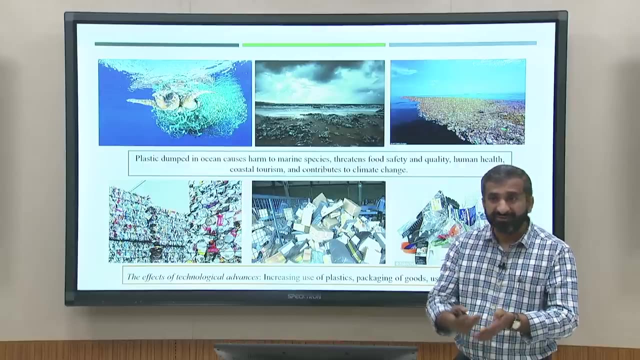 changing And whatever technology we will propose, That may be after 15 years, 20 years, that technology would not be beneficial And the way our waste generation is increasing, especially from last 5 year to 7 year, is very difficult to believe that the way our waste generation generation is increasing. 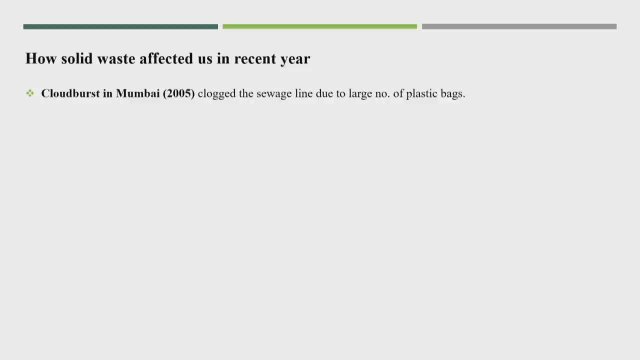 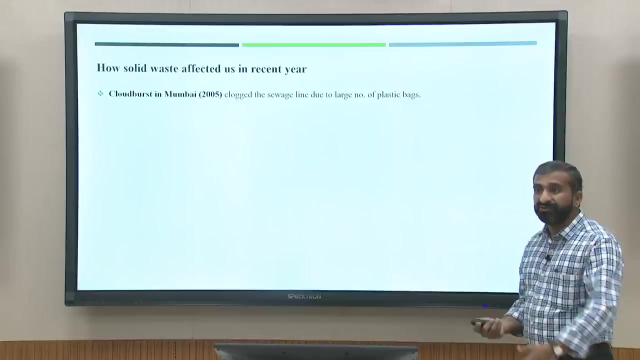 You see that I have some of the data about the cloud burst in the Mumbai 2005 and mostly we see that in Mumbai Ah, The power sever network, specially in the monsoon season, is getting clogged off and every year in Mumbai we will see the the flood issue and why the flood issue is not because of 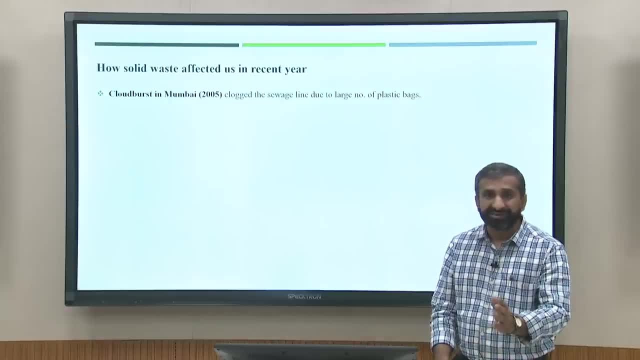 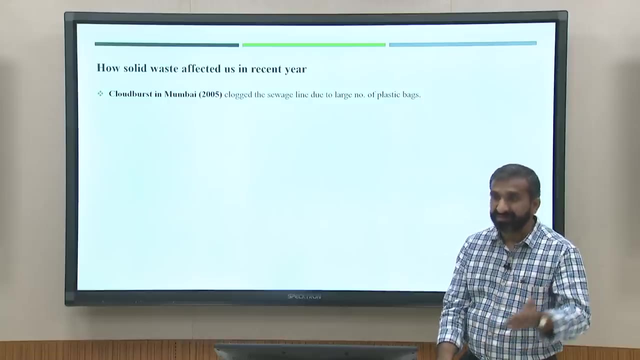 they do not have power sever networks. but because this plastic, the way we are getting disposed off that plastic, is adding into the sever network and these became a, these plastic be is getting clogged into the sever network And is the Mumbai always getting the flooded in every year? 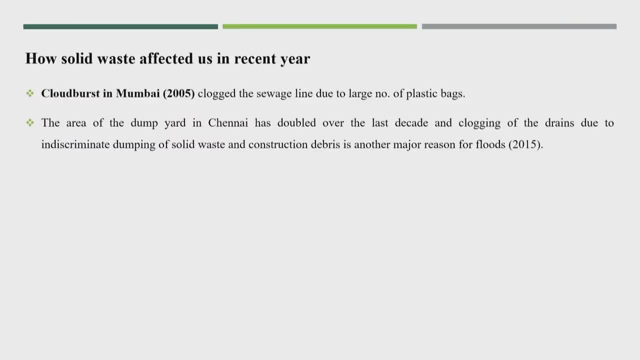 Like I got surprised when you say that Chennai had a flood in 2015.. So was very difficult to believe that Chennai could have the flooding, And I believe that these flooding is because of because most of sewer networks or the- wherever the water is going out from the city, that has been clogged by the solid waste as city. 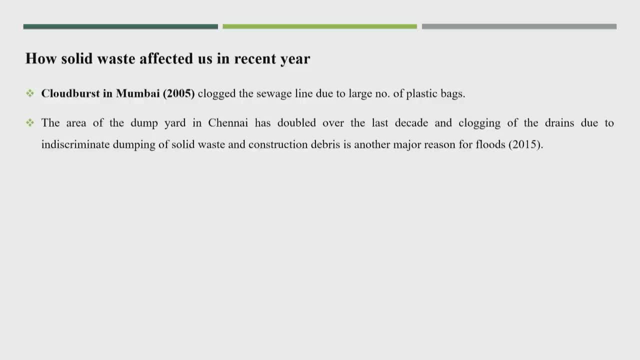 become flooded completely And we normally in the urban centers also. we never thought about the how benefits of the wetland and the better proper space. space is very costly in India now. land is very costly in India. The people would not think much about the benefits of the wetlands where water is getting. 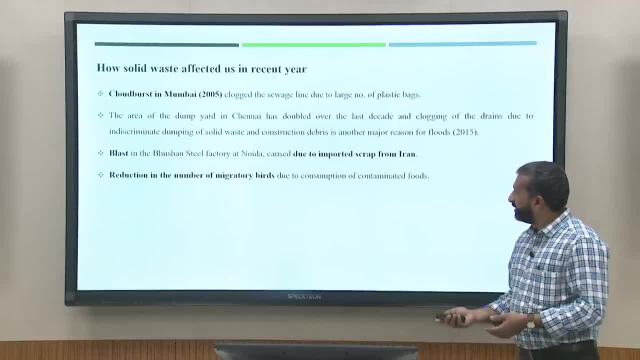 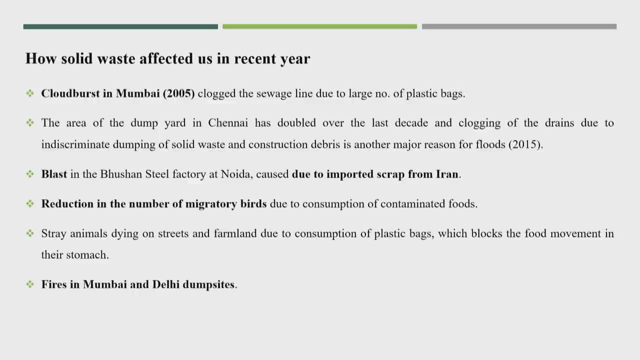 stored off. So there are few more like the fire. one more, the fire in landfill area, I think might you remember about the fire- work was found, I think that extended for the more than 15 to 20 days where Mumbai landfill got fired off. 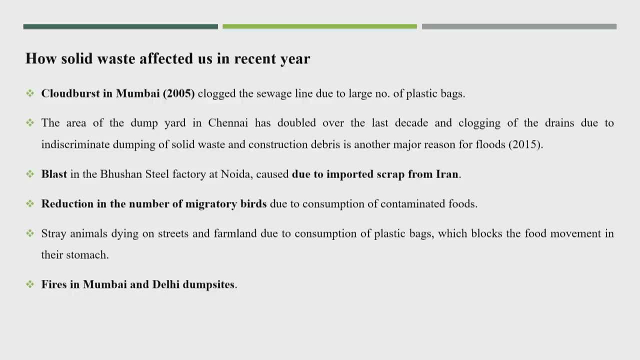 These firing people were talked about. this firing is because of methane production from the dumping area, But also, along with that, not only this fire is because of methane production, but also if you see that in the dump site, the lighter material, that paper and plastic will be always. 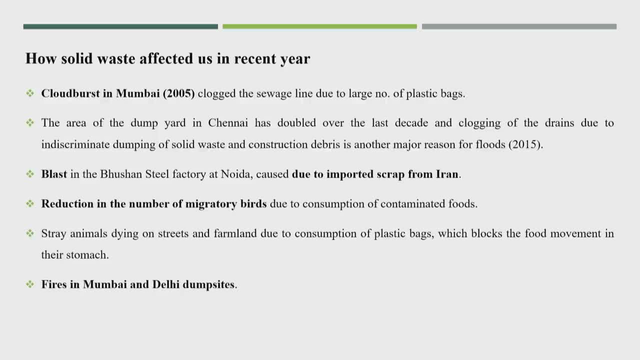 on to the top and always because the entire the dump site under the anaerobic condition. So obviously some kind of methane will get produced and this methane- methane- maybe that quantity is not very large But in the dump site But is able to get fired off or purposefully. also many corporation is firing the landfill. 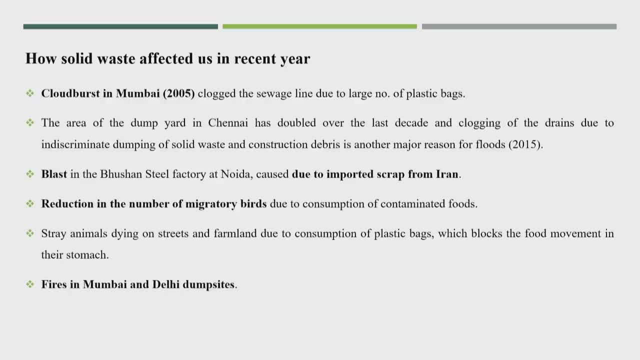 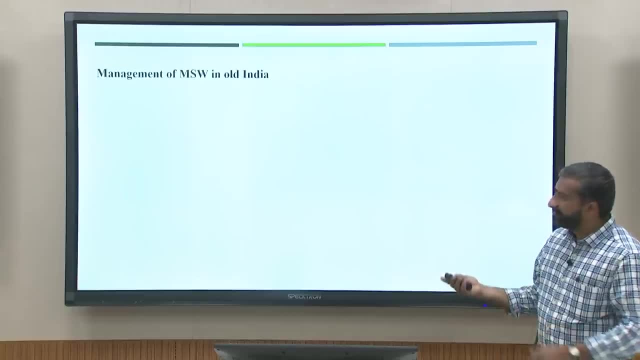 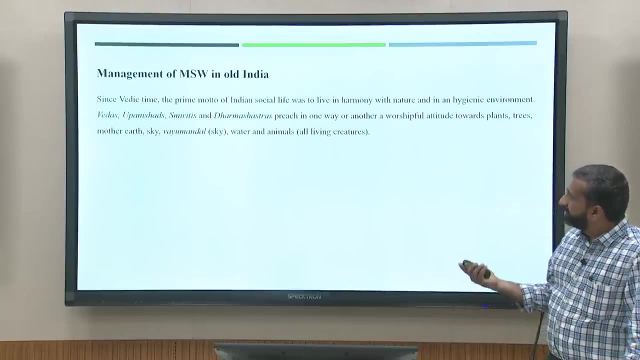 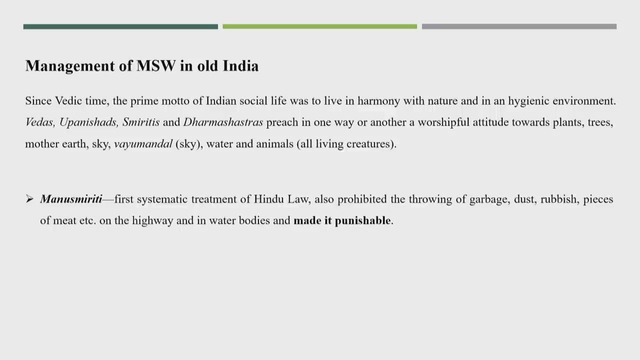 to show that the entire dustbin do not have the paper and plastic waste into the waste material. Now you see that some the past literature in old India, since Vedic time also, we used to talk about this waste, Waste management. So I have some some information about the one very important document like systematic 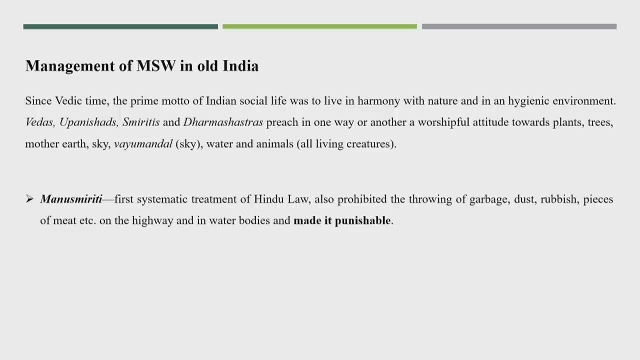 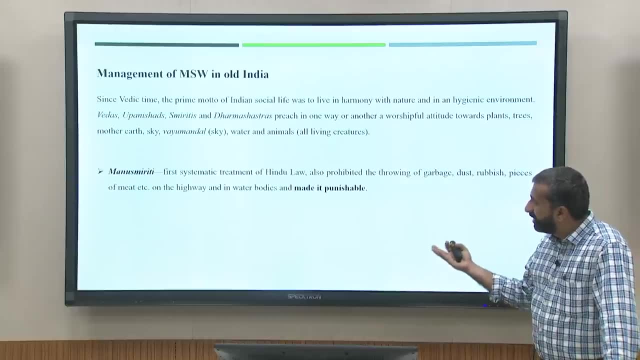 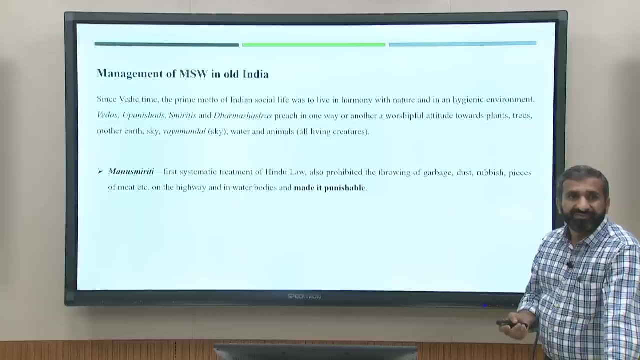 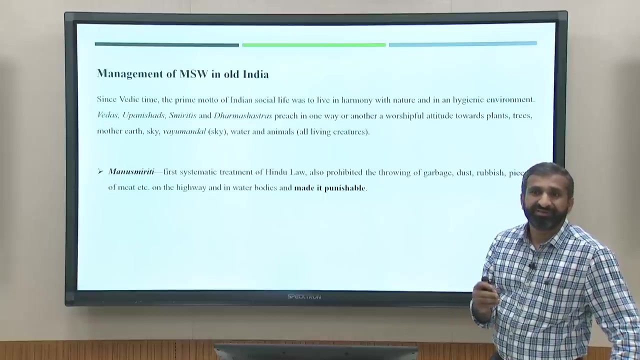 treatment of Hindu law, Manusmriti, that says that it prohibited the throwing of garbage, dust, rubbish, piece of meat on on the highway, on in water body and made it punishable. See, that was wrote it Hundreds of years before this thought was being proposed. 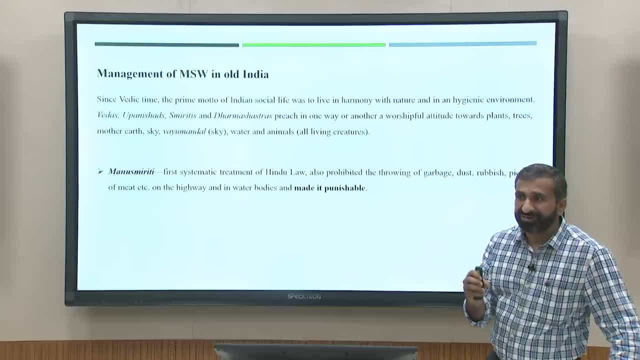 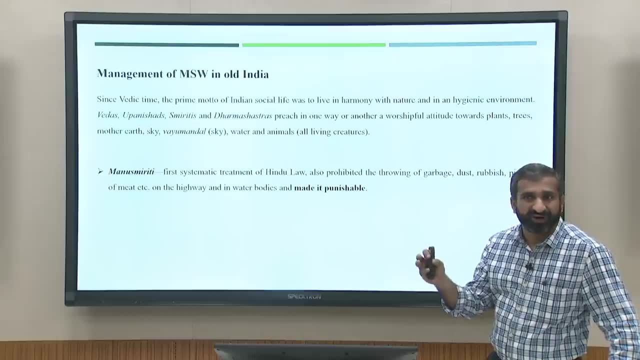 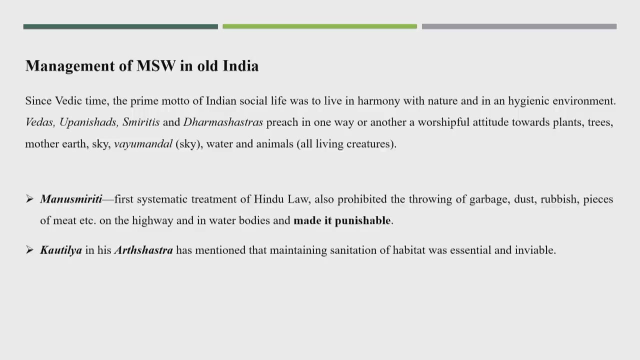 This waste should not be disposed into the water body, should not be thrown onto the highway, And if anyone will found to get disposed of need to be punished. Another document like Kautilya's, Atharveda, also talked about the sanitation of habitats. 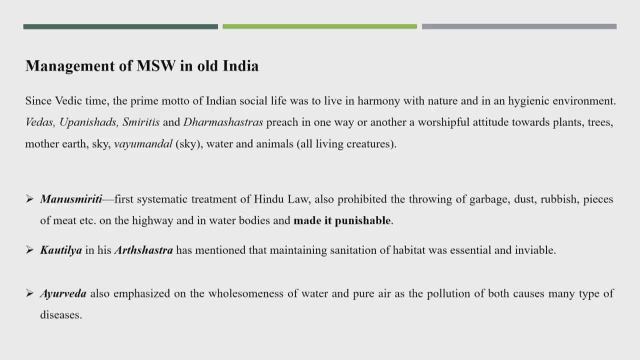 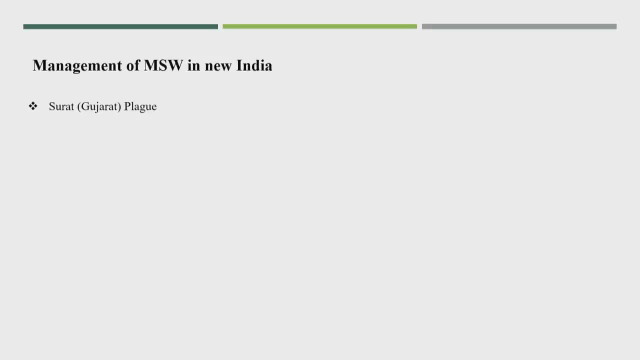 made it very essential, And also another document called Ayurveda also talk about wholesomeness of the water and pure air. But now in the management of MSW we will see the management in the New India management of solid waste in New India. 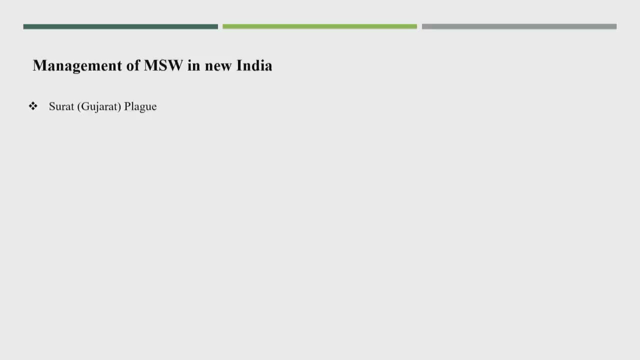 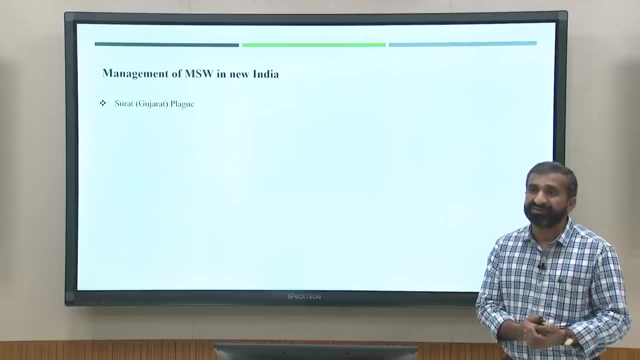 So I was talking about. the Surat plague was the first event where we thought about, or we came to know that, That the importance of solid waste management, where a lot of people have died because of the Surat plague. maybe hundreds of people have died because of that. 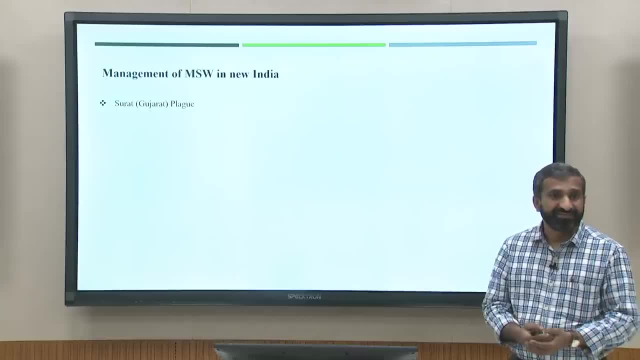 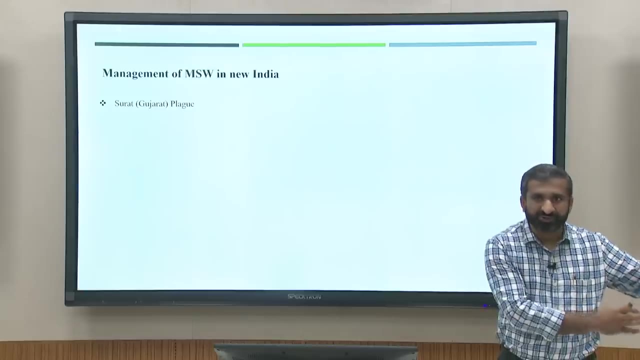 Surat known to be a textile city, and the waste used to be produced by this textile industries are mostly a biological matter and that never used to get disposed of out of the city used to be disposed. So it is a very close to the industrial area and these industrial. because of that, 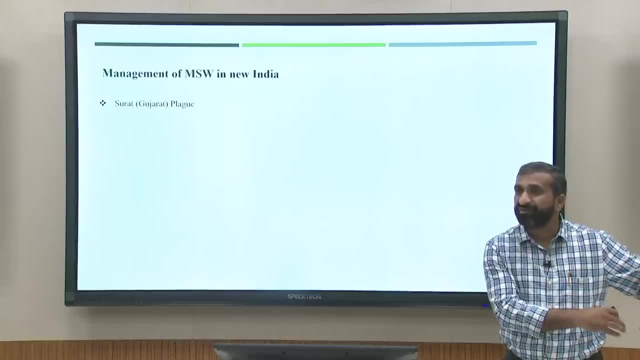 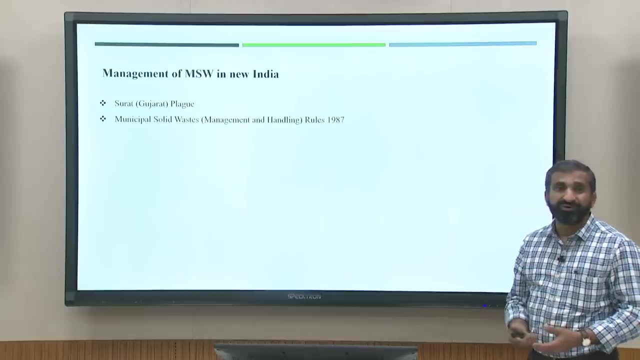 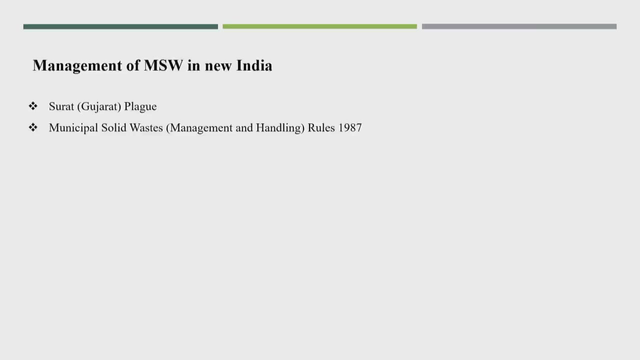 lot of rats had been attracted to such waste because that was very biological waste and because of that the India thought about to propose a special rule that was municipal solid waste management handling rule 1987.. So first time in 1987 the government of India proposed a special rule that it is a part. 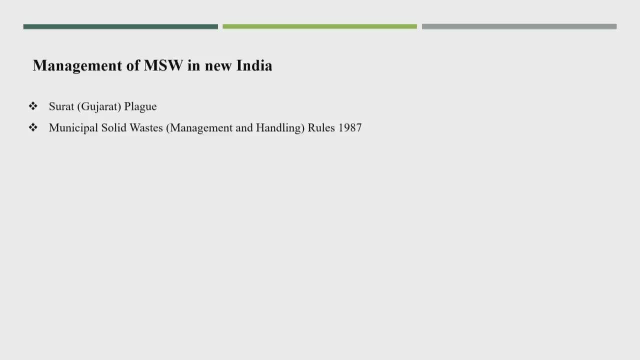 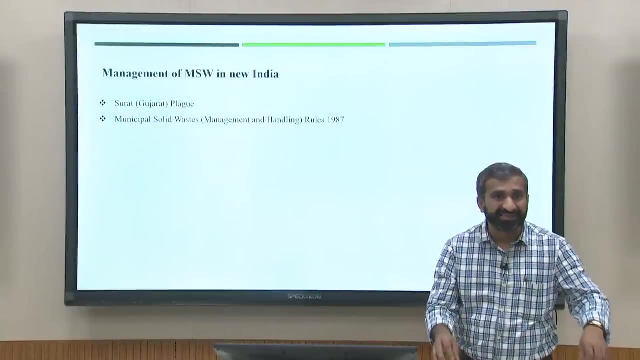 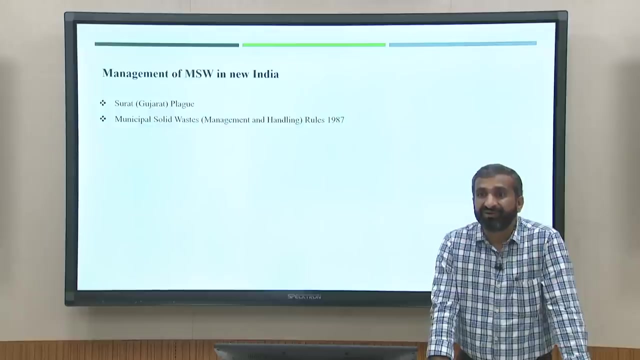 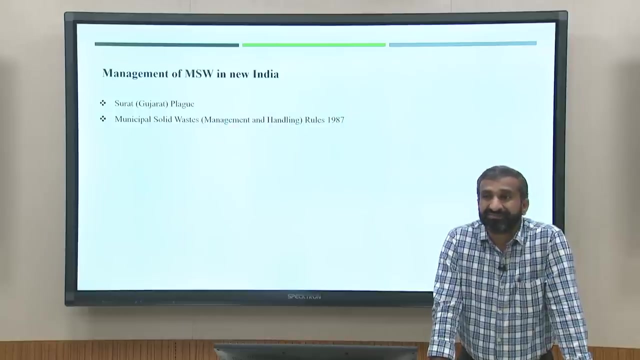 gave one of the important thought to the local bodies or corporation area or urban local bodies: apart from water supply, sewage collection also. they need to collect the solid waste But was very difficult for the ULBs to understand that they never thought of, sometimes because water supply is very easy. 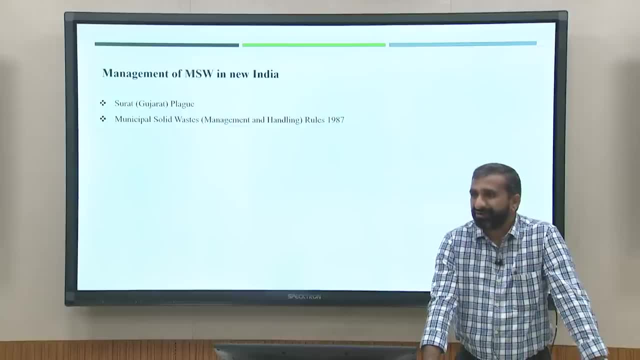 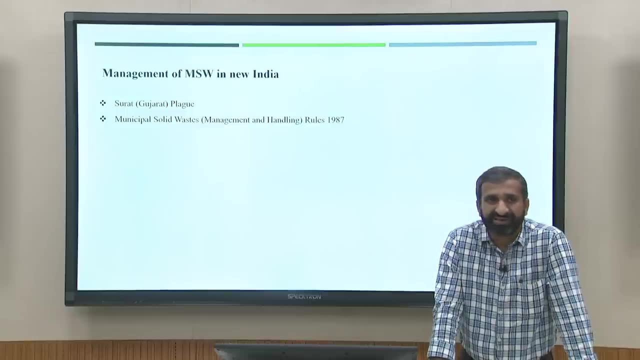 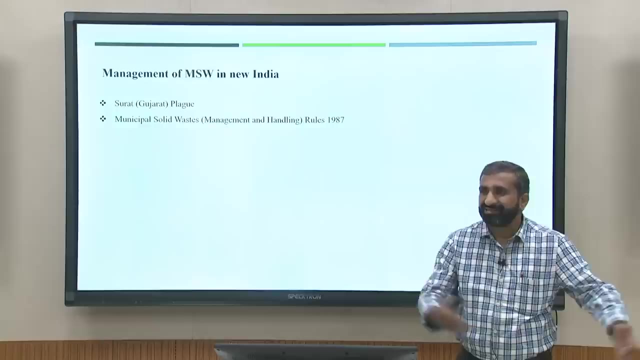 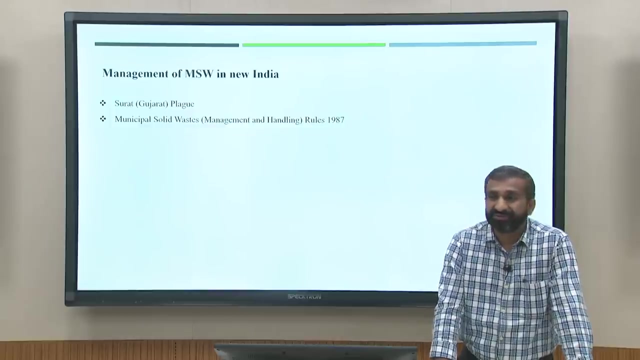 You construct the pipelines and you supply the water and your or you find one particular source, whether is a surface area, surface water, whether is a ground water. find one, one particular source, construct the supply lines and flow the water. was very easy. But now, when this task has come up, to come up to the ULBs to collect the solid waste. 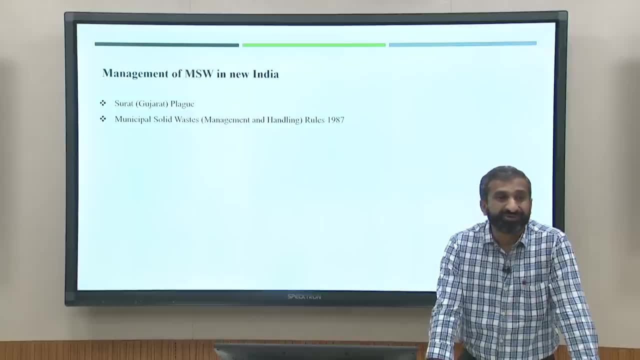 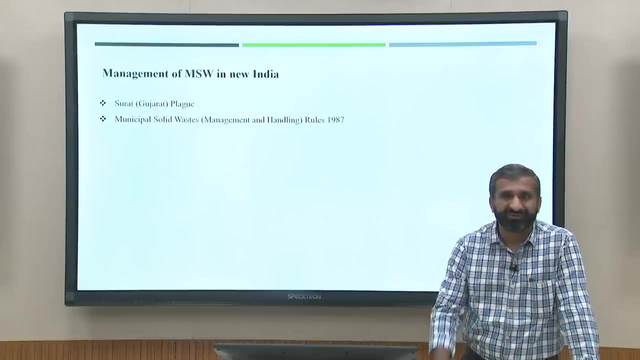 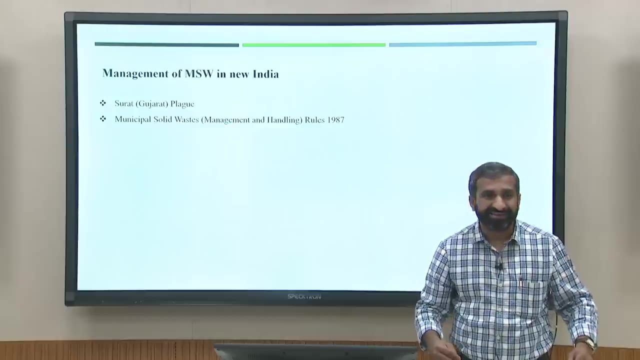 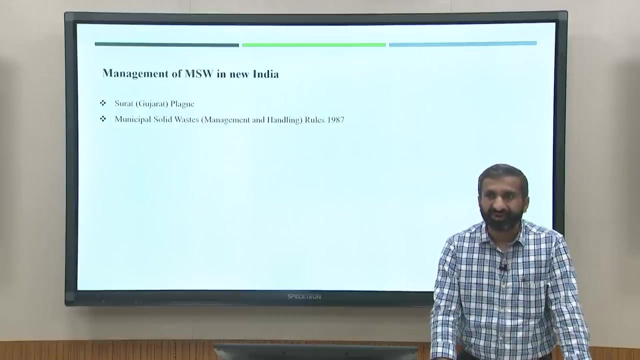 collect the waste. they never thought of because your sources was thousands, lakhs of sources. Each house was producing good amount of waste They never thought of and they they got very surprised that whether now they have to go to the each house and get collect the waste. so how best they can do it. 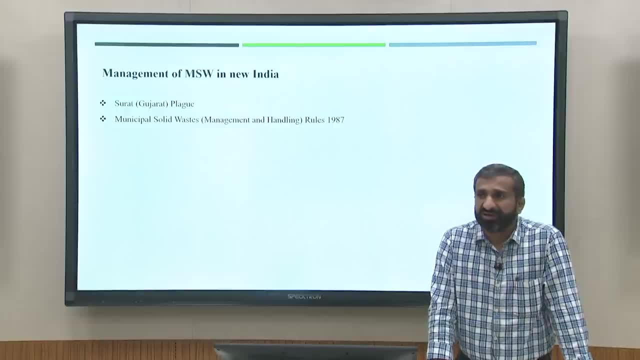 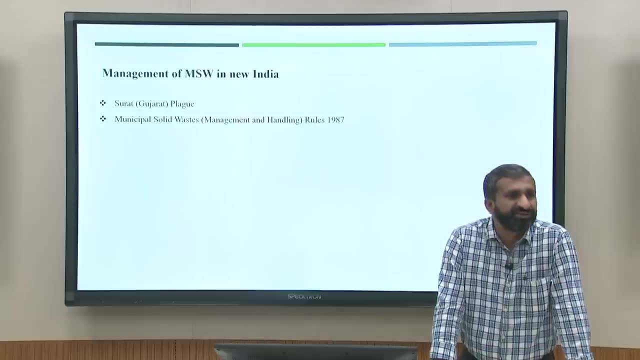 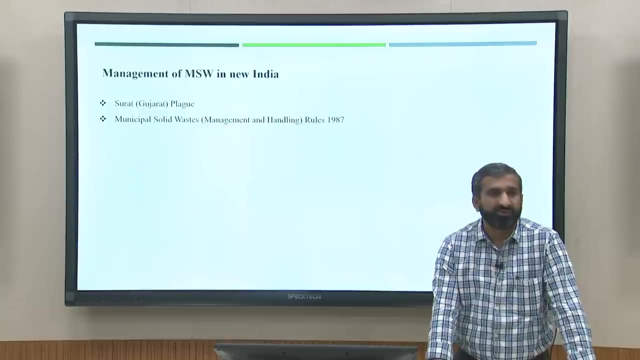 So under this rule, the what corporation did? they? installed number of dustbins into the city and asked the local people to get dispose the waste waste into the those dustbin area. That was a simple collection system. the most of the ULBs have started and had been asked. 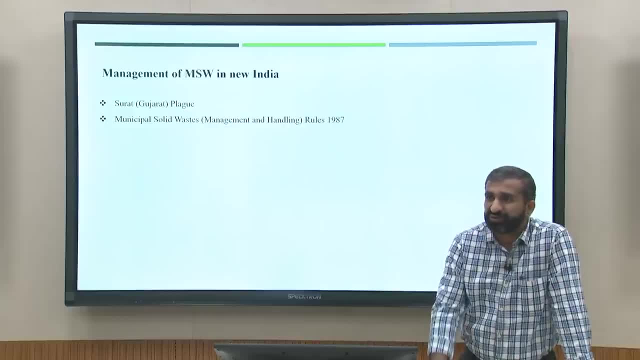 to the local people to dispose the waste into those particular area and what corporation used to do. they used to collect the waste from the those dustbins area but was very difficult. They were finding location into the some low lying area outskirt of the city. was transportation? 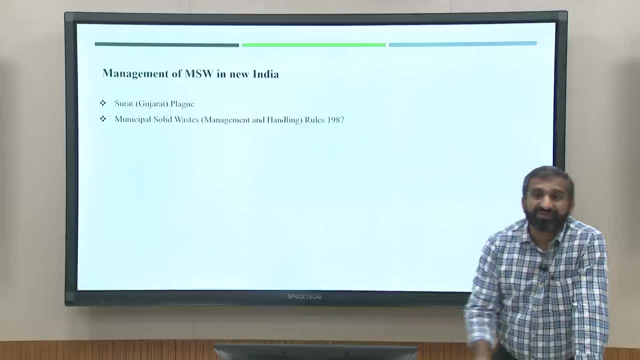 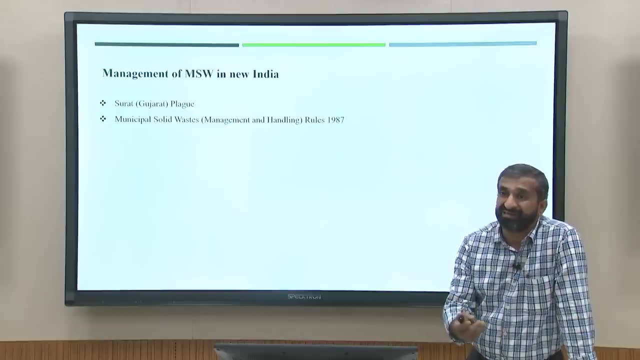 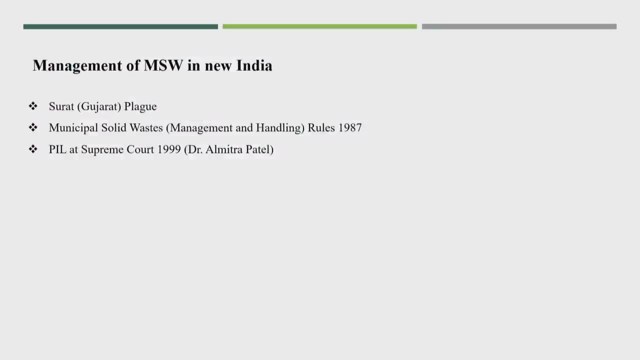 cost very difficult. So most of the city was was was unable to extend the extend this solid waste management or solid waste collection facility. forget about the treatment in those days Then. one PIL has been submitted by Dr Almitra Patel. normally we called as a garbage lady. 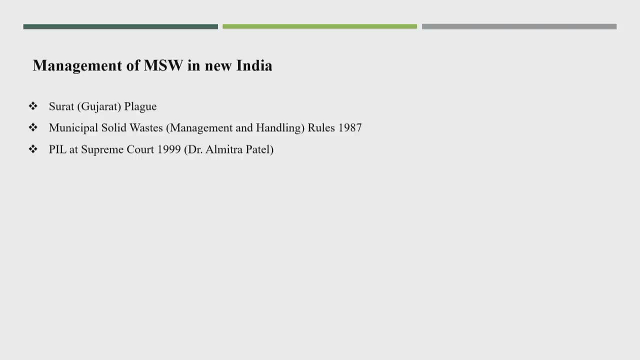 of India. She submitted one PIL in Honorable Supreme Court saying that ULBs or corporation was not able to do the proper solid waste collection and treatment and was not able to dispose into the proper landfill area. Then in 2000, in 1999, Honorable Supreme Court made a one special committee under the Supreme 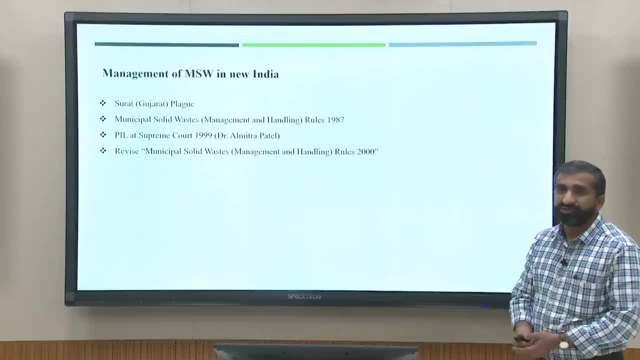 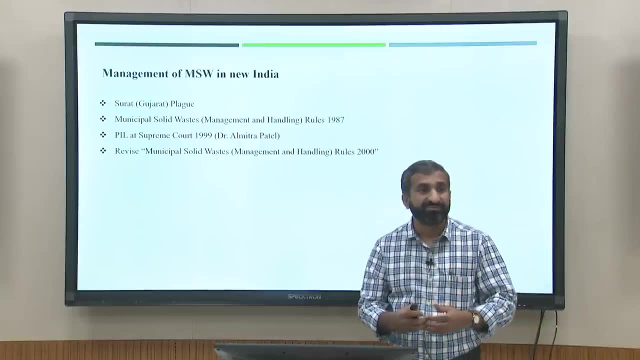 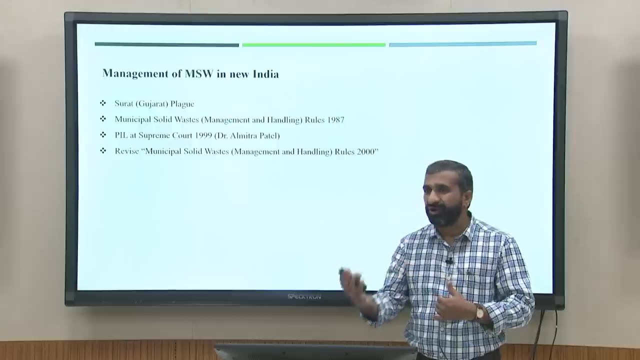 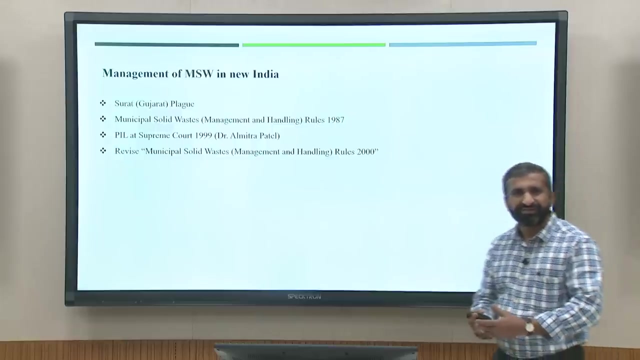 Court the solid waste management rule in 2000 and there I think the first time the solid waste management was related to the public health, So that people will be easily understandable how important is the solid waste management issue. but still I think again the issue was with the always, because when you say the collection, 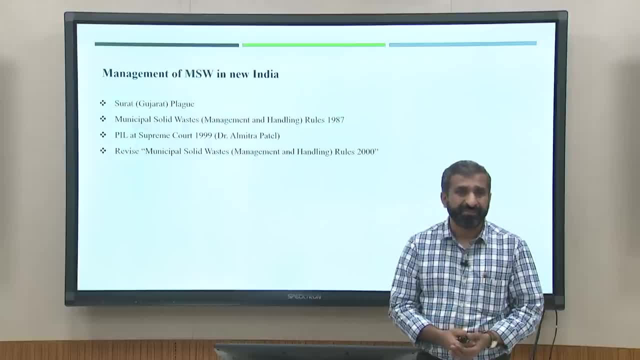 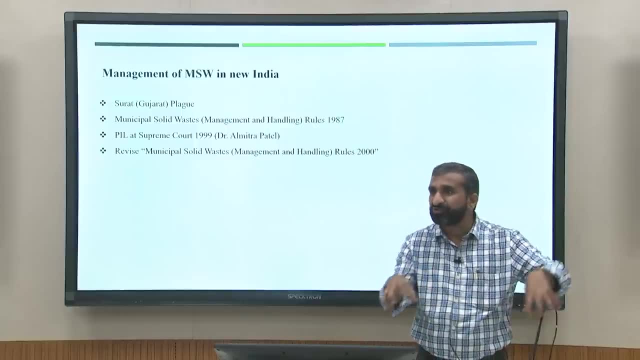 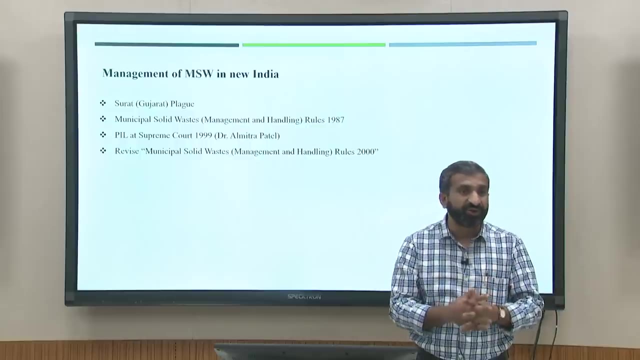 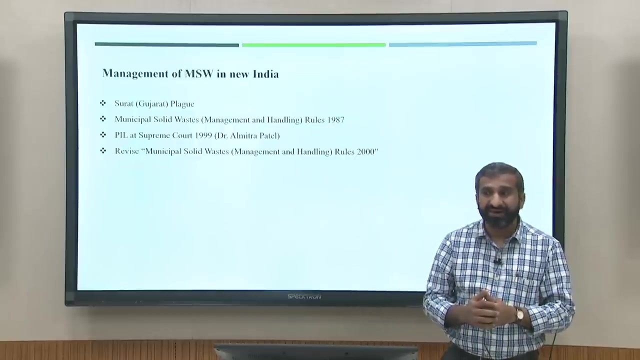 issue in the solid waste management is a very costly process because I think in the initially also when we install the different dustbin. so the collection cost was very high, very large to get collected- 200, 300 number of dustbins located into the city. So collection was very important, very costly process and once you collect also and come 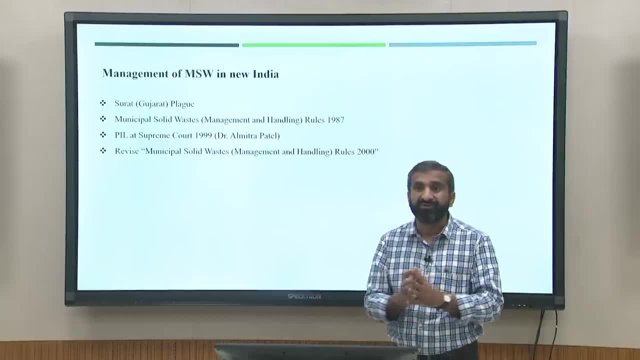 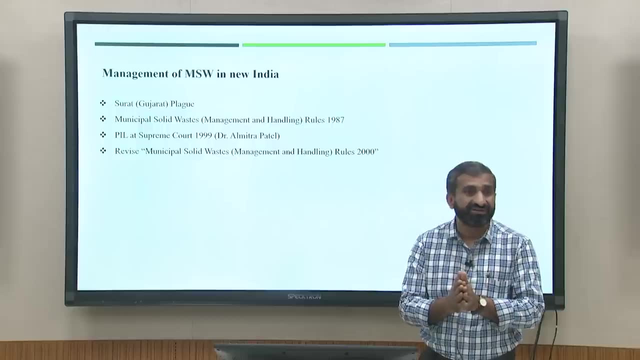 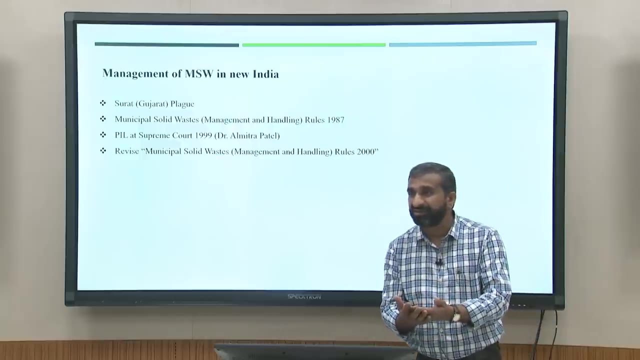 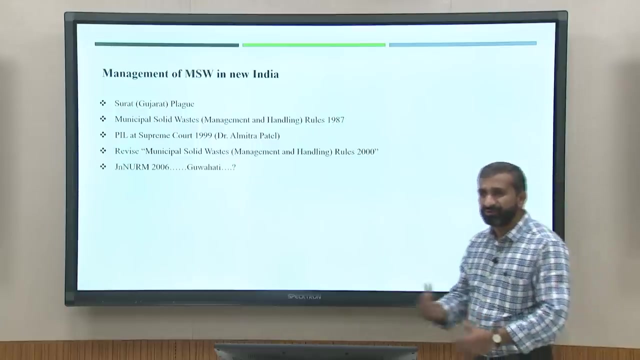 up to the disposal site was very difficult. You have one proper treatment facility So we do not have proper fund fund for the collection, because earlier we never thought about there could be a some kind of collection fee from the producers, from the household area. Then one other scheme has been proposed. I think we know that is a one of the very important. 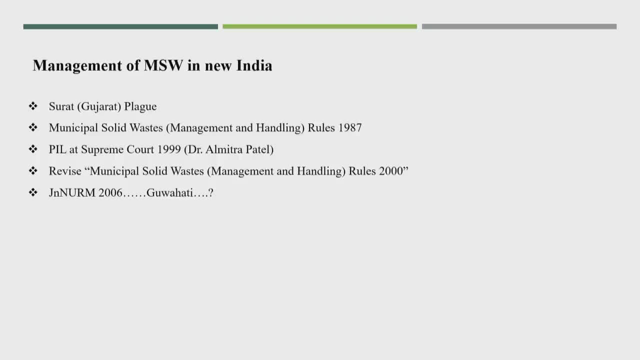 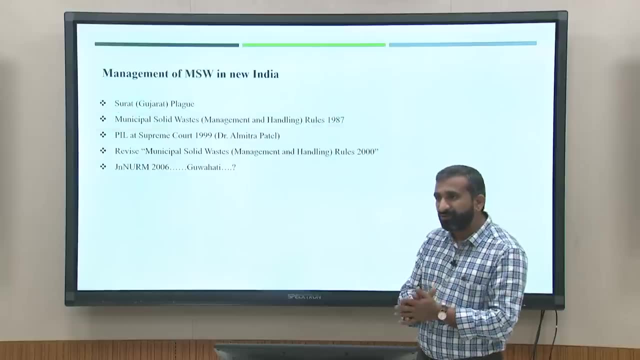 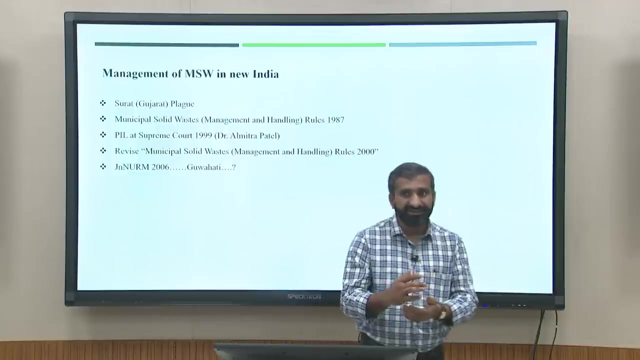 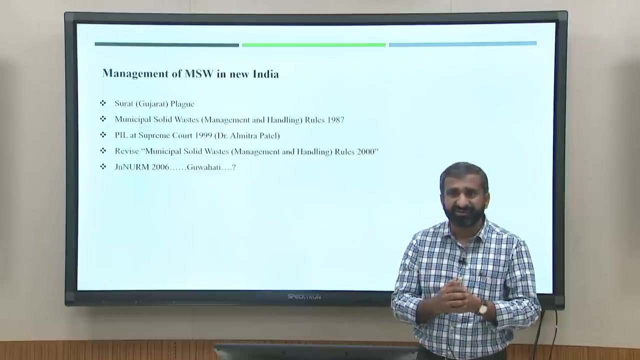 scheme JNRM 2006.. Jawaharlal- Jawaharlal Nehru National Urban Renewable Mission. The target was this mission to help, financial help to the ULBs and in the 2006 in the scheme one, there were 35 cities was been selected for financing for the, for not only for solid. 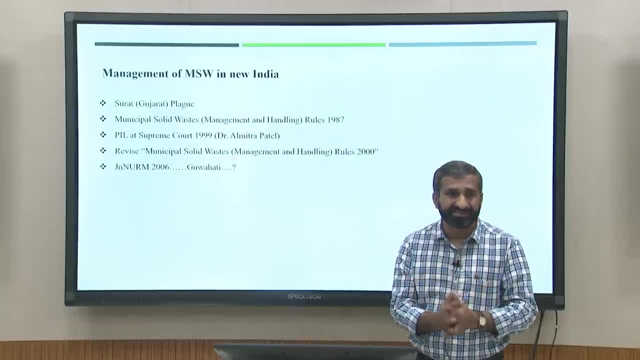 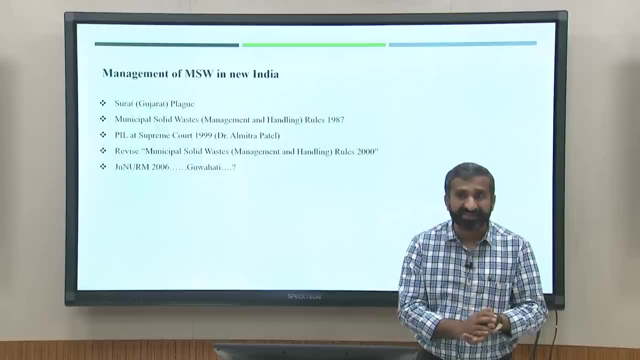 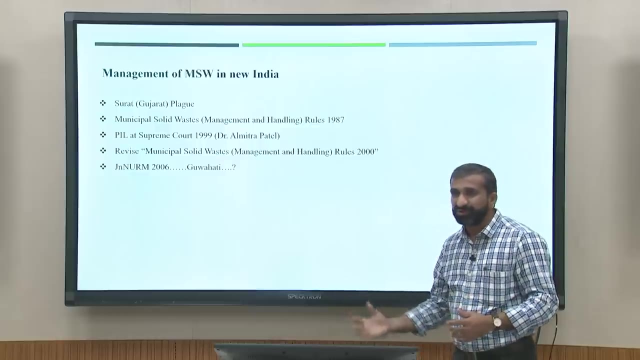 waste management But For the communication purposes. So many cities got water treatment facility. many cities got proper transportation facility- might you have? you have seen the big, big buses under the this JNRM scheme? and also some cities got lot of fund for the collection, solid waste collection and disposal. 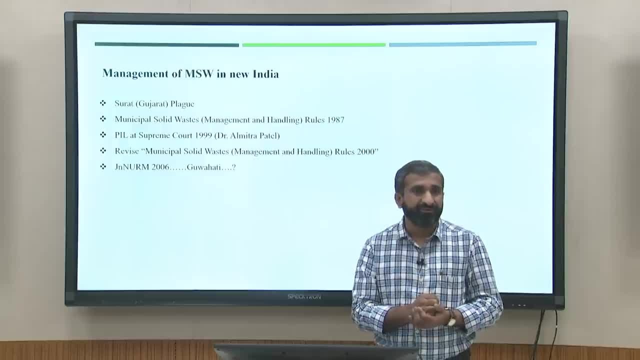 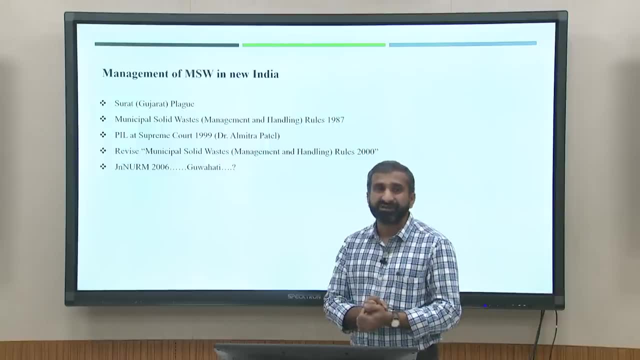 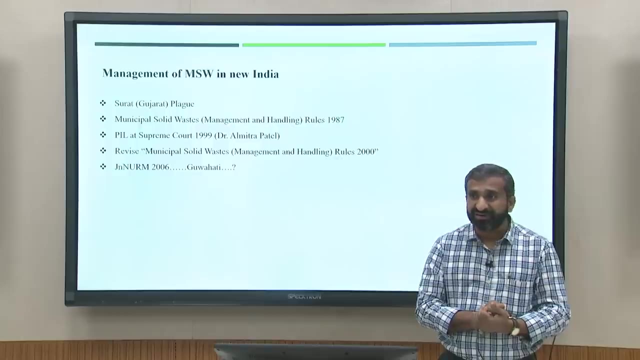 And under this scheme only the first time we thought of the PPP projects, Public private partnership project project- because in solid waste management, because collection was very difficult, very costly process, So corporation was not have enough fund, So the private authority had been asked to the private authority to come forward to help. 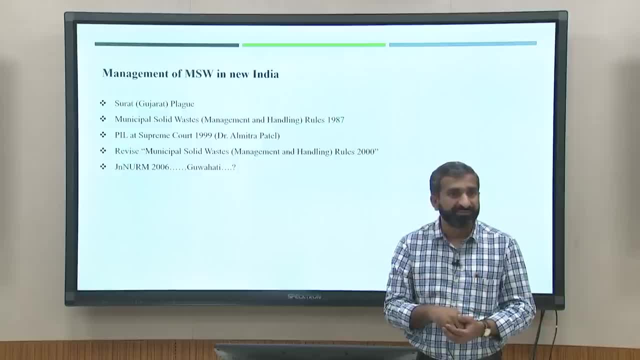 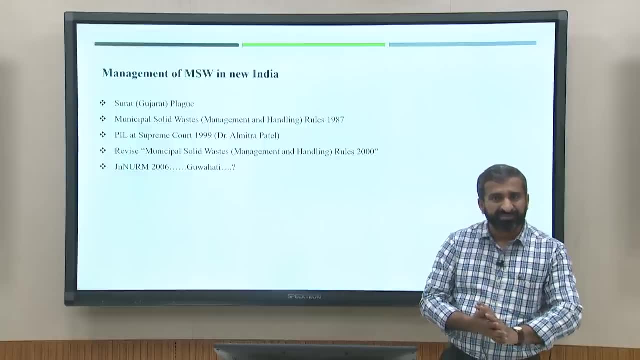 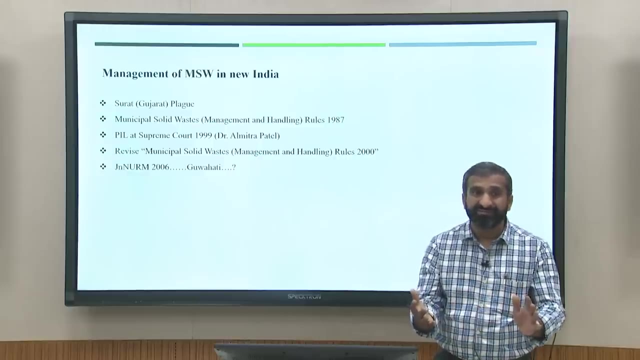 the corporations under the PPP program and to fund the, the current collection and treatment facility. And why private company was very positive about this? Because they thought of, because the waste- this was not the simple waste. Because they thought of there are. there will be a 50 to 60 percent of biological waste. 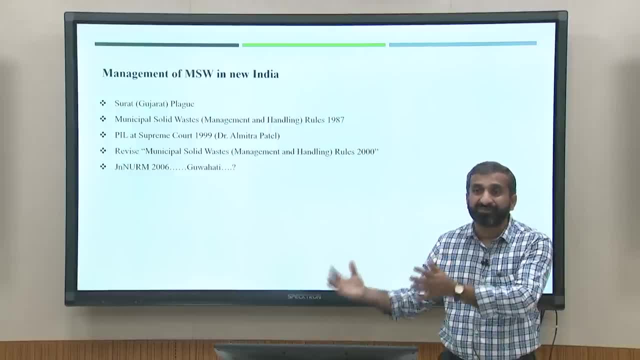 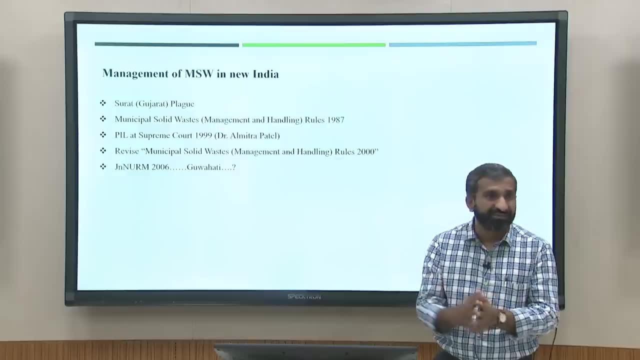 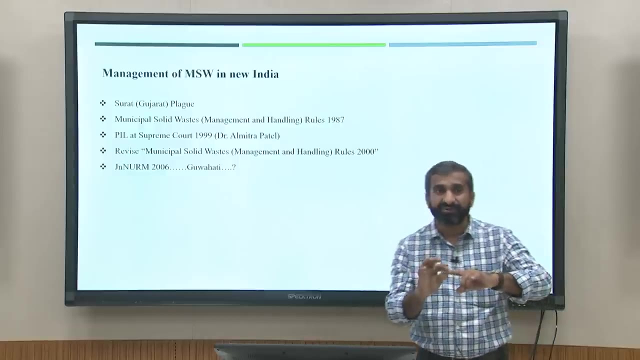 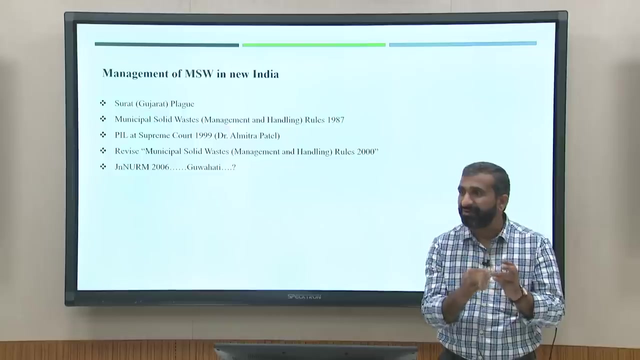 into that So they will be able to produce large amount of compost from that and be remaining. that 20, 30 percent was recyclable matter and mostly the- when you talk about dry matters- was mostly a recyclable matter, Like, For example, of paper, plastic, rubber, leather, metal, glass. everything is recyclable matter. 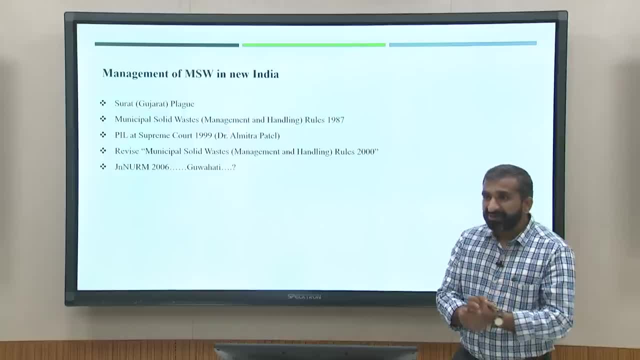 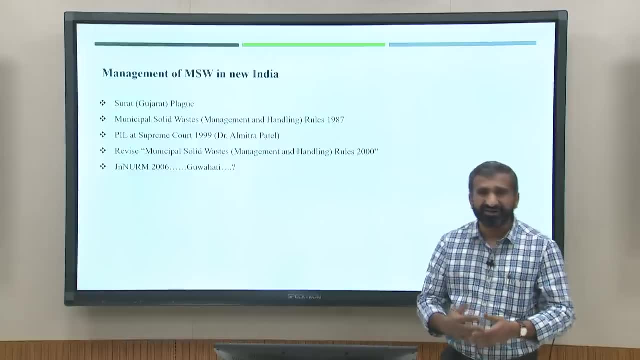 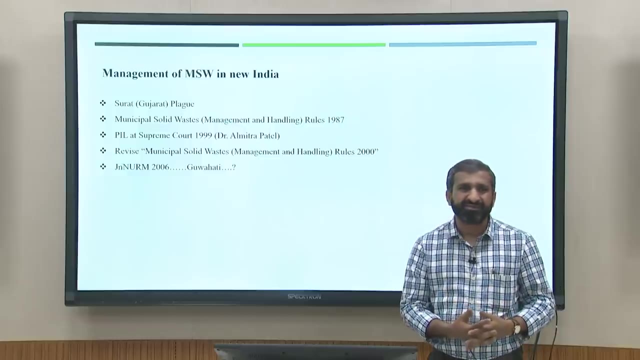 and very costly matters. But I think when the private company has come forward, they they thought of they will get lot of benefits of that. But was very difficult because the way our collection system is, a was a mixed waste collection. There was no segregation. 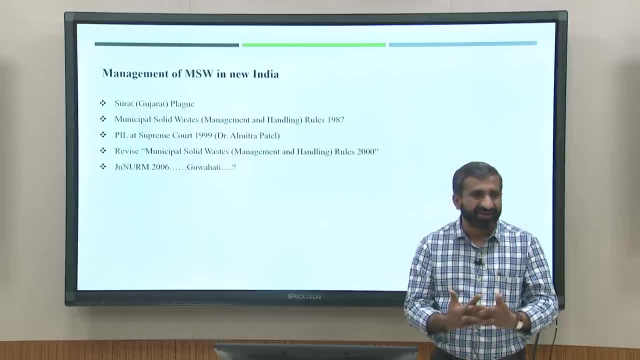 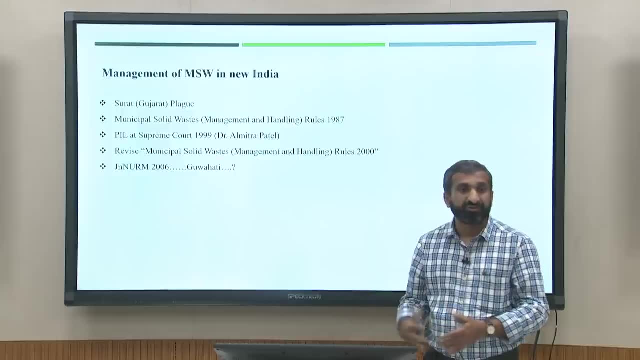 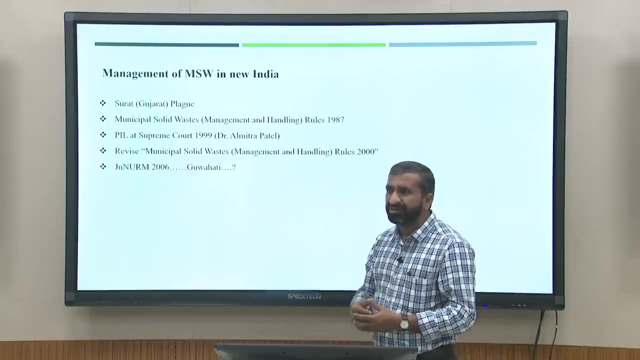 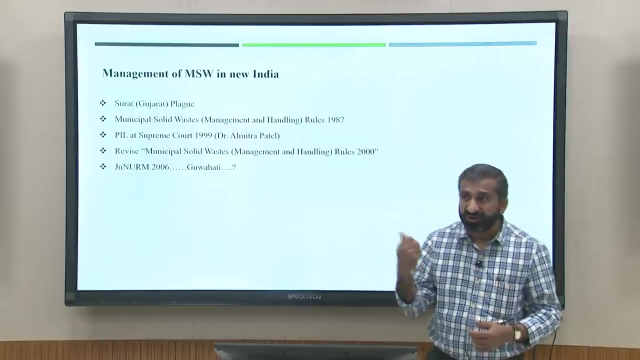 And When, When the private company they tried to collect the waste, So same the collection system get it and and disposed of one location was very difficult to get segregated. So they never, never found the proper compost production, never found the proper recyclable matter which can be easily recyclable or which can be sold off in very good cost. 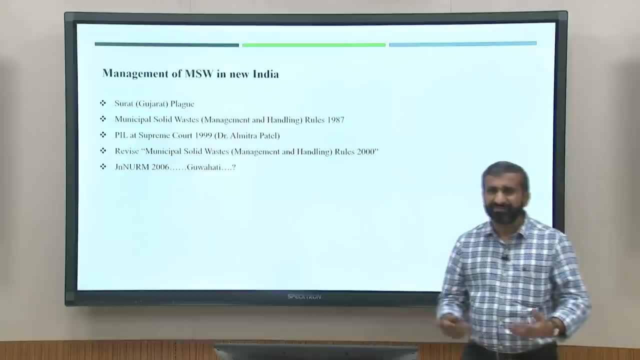 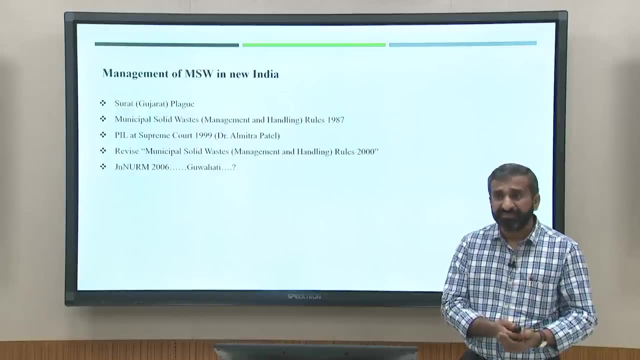 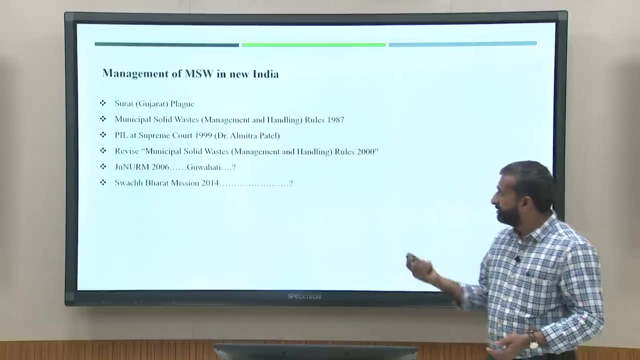 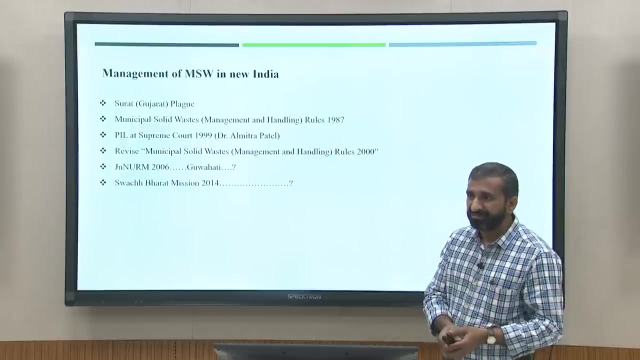 So then I would not say that this scheme has been Failed off, But I think many cities got lot of infrastructure facility, at least infrastructure facility. Many cities got compost plant under the JNRM program. Then, in 2014, the Swachh Bharat mission has been proposed or announced. 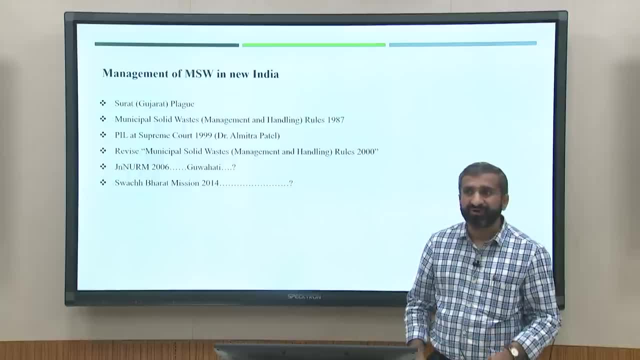 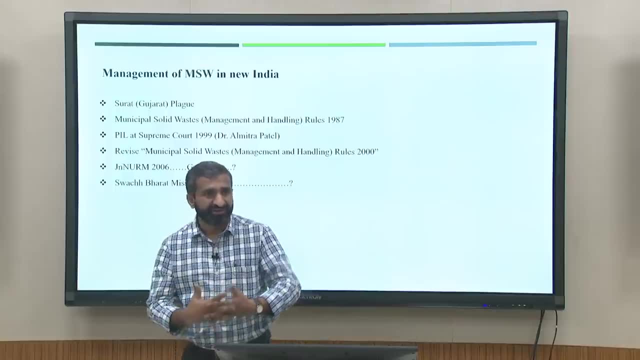 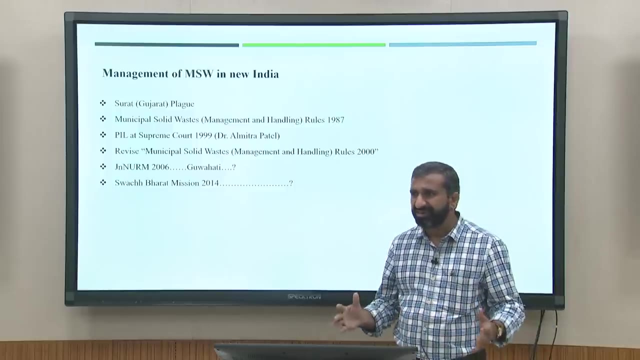 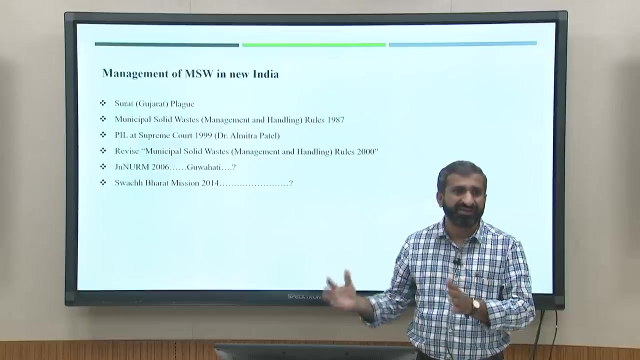 So what was the major, major, important point of Swachh Bharat mission was the waste segregation. And that was a very good initiative in the solid waste management Because from the our we saw that our history of waste collection in India, that mixed waste collection, was never found the beneficial. 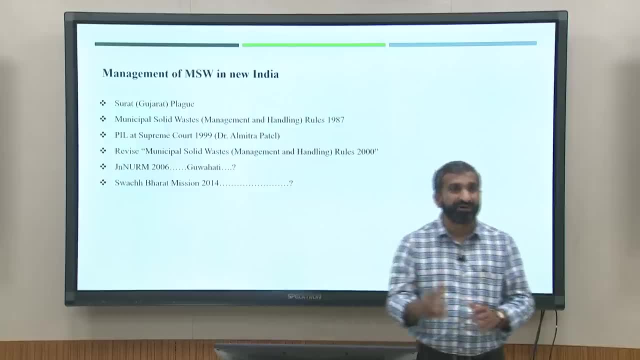 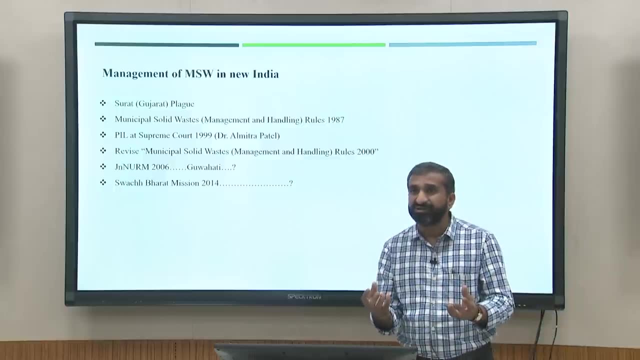 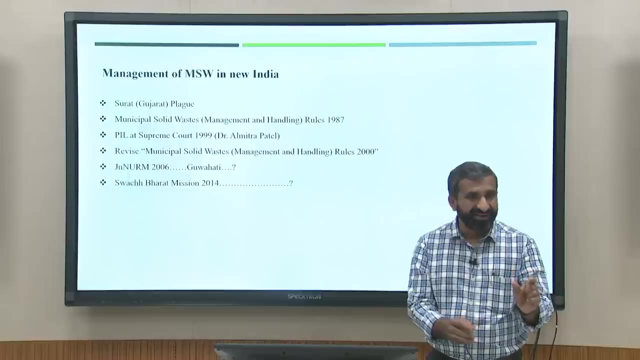 Because we are not able to produce proper compost quality, proper recyclable matter. So the Under Swachh Bharat mission, The segregation was the important issue. So for every household has to be segregated into the three parts: dry waste, wet waste and third part was household hazardous waste. 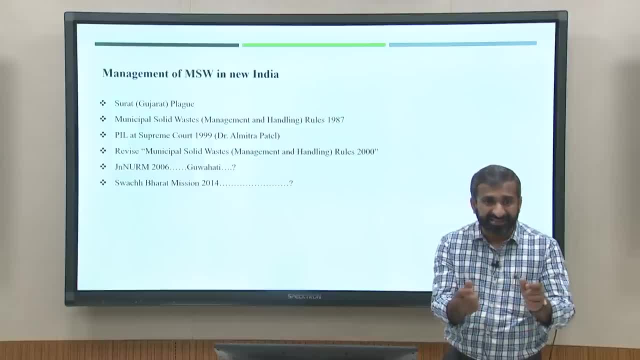 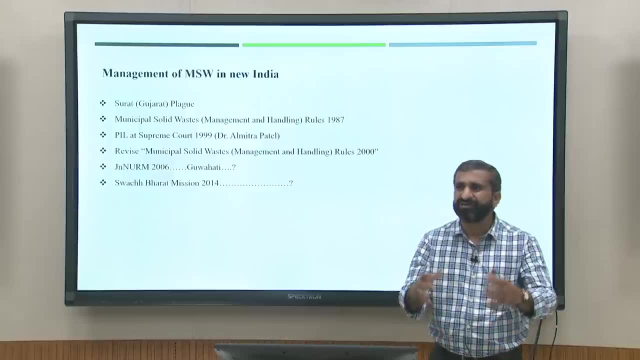 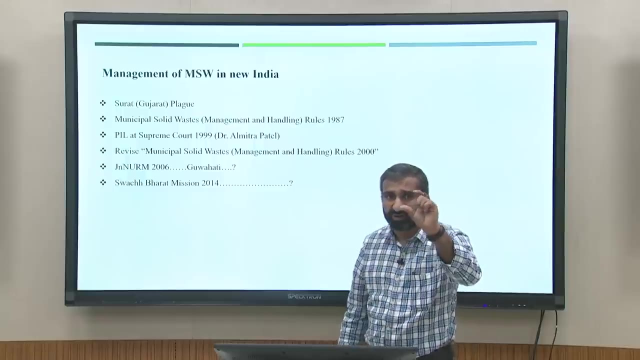 That was a third part and based on the segregation, you finalize the collection system and followed by treatment facility. So that was very simple. thought was been proposed in under the Swachh Bharat mission because once We are going to segregate household level or date source itself, 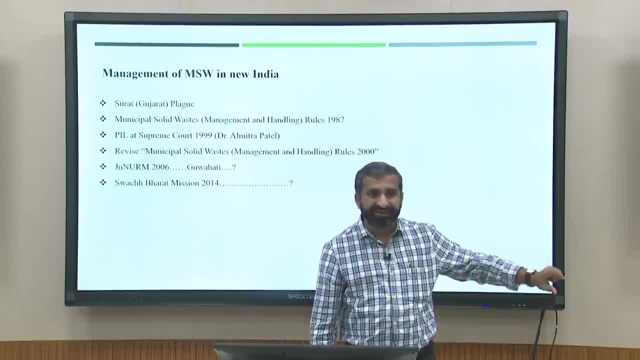 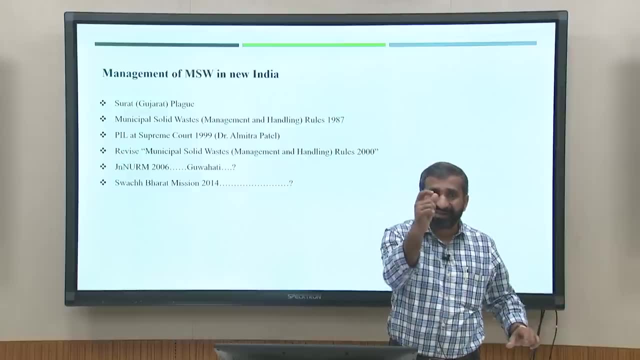 So that biological waste will go to the biological treatment facility that could be a composting facility or biogas generation facility, and this dry waste, because it was a this was not contaminated one and mostly materials was recyclable one. So like paper, plastic, rubber, leather, metal, glass, 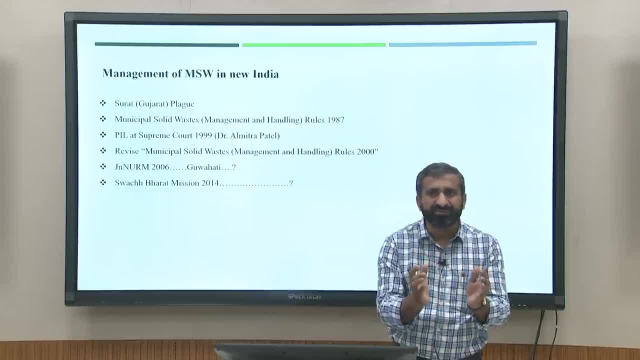 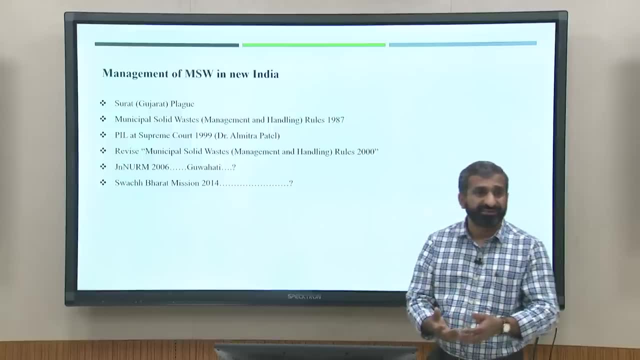 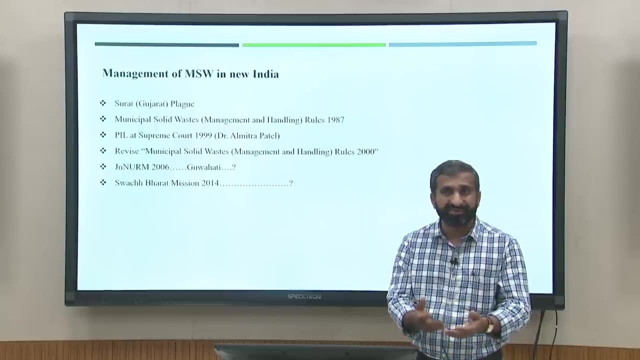 This all goes to the recycling facility. Only the 10 to 20% will be remained for the disposal area. But I think you saw that number of cities has been started the work on to the proper waste collection And we saw that in Madhya Pradesh, Indore, Bhopal, became the one of the cleanest city. 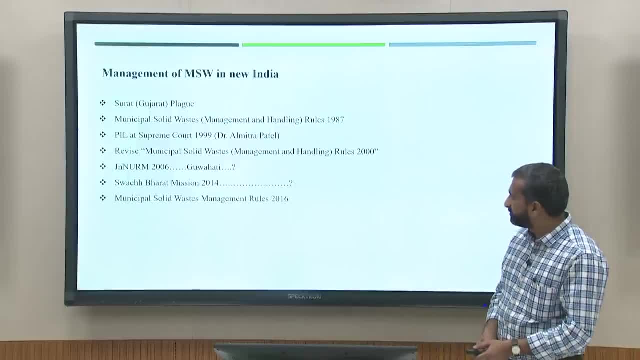 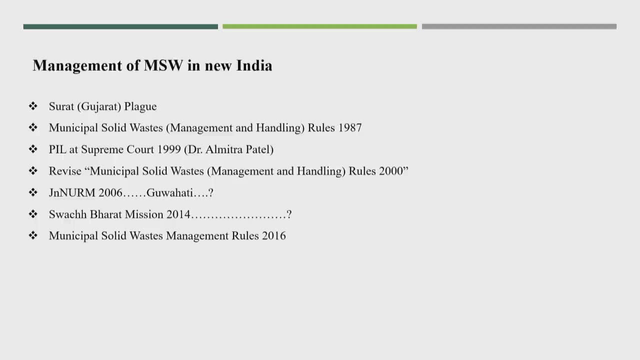 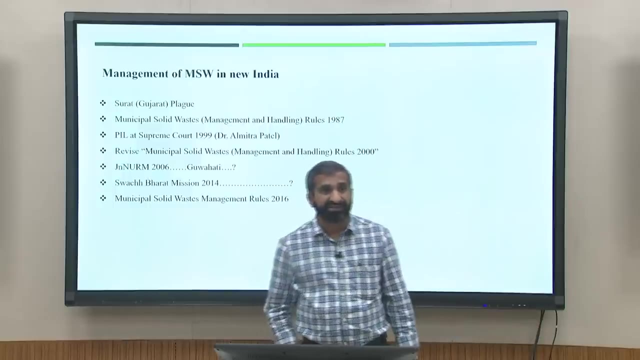 in India for last two to three year And also in 2016.. The rules have been modified. Okay, That is solid waste management rule 2016.. And now this rule rule also suggested that segregation and also propose first time under the rule the, what kind of compost quality has to be produced. 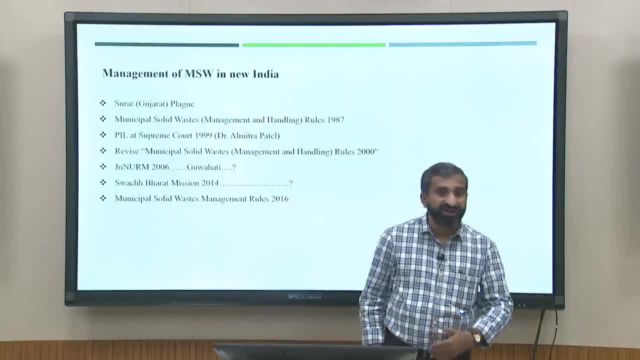 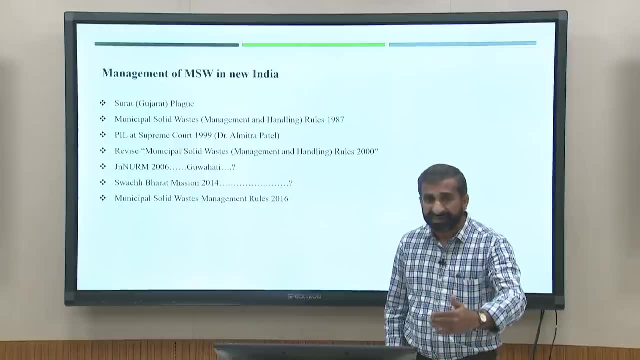 What kind of recycle, recyclable matter has to be produced And when you go for sanitary landfill, what kind of leachate are getting produced off And what kind of treatment, What kind of waste management facility has to be provided for that leachate treatment? 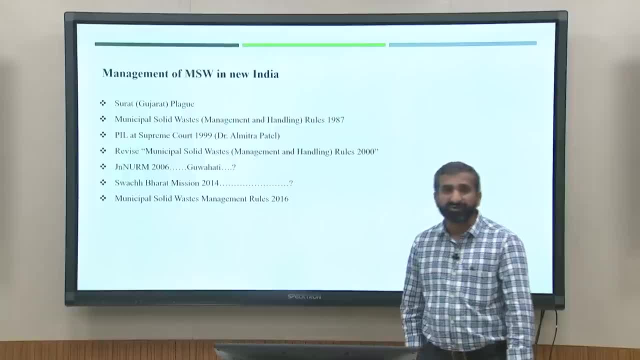 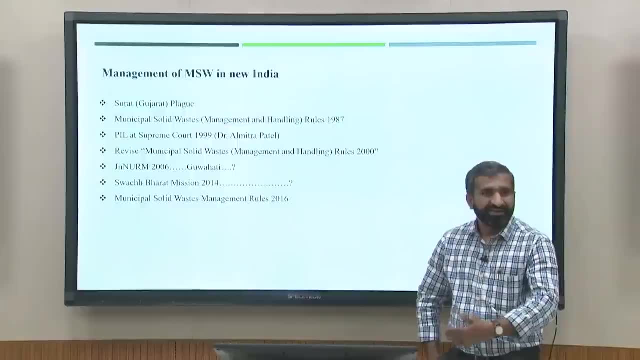 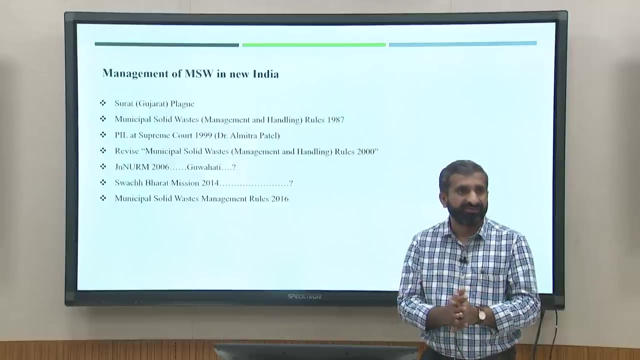 has been proposed into the solid waste management rule 2016.. Okay, So now we see this solid waste management rule 2016.. So under the first lecture now, I think I believe that you people have understood what is solid waste management and how important is solid waste management to study. 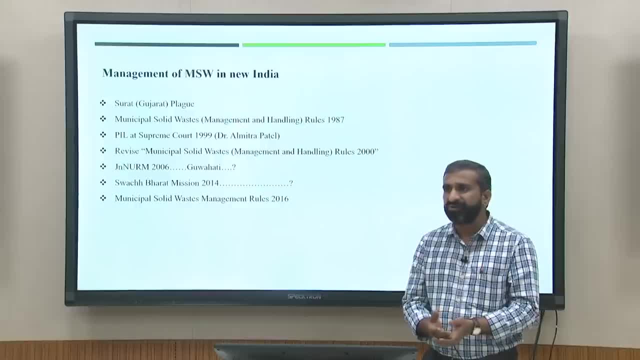 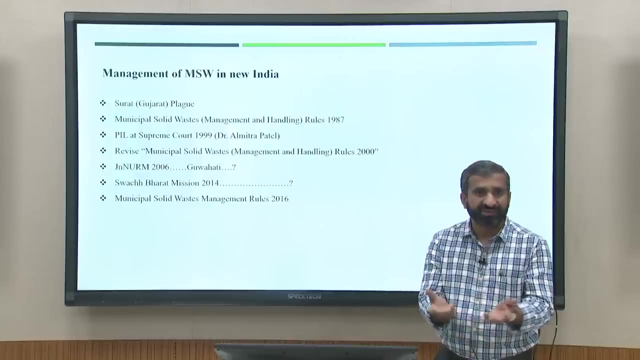 So in the next lecture. I think you will understand. Okay, So next lecture, I think we will talk about the function elements. On that function element we will go one by one function element to the next two next lectures. So if you have some kind of questions you can ask me or some kind of queries you can. 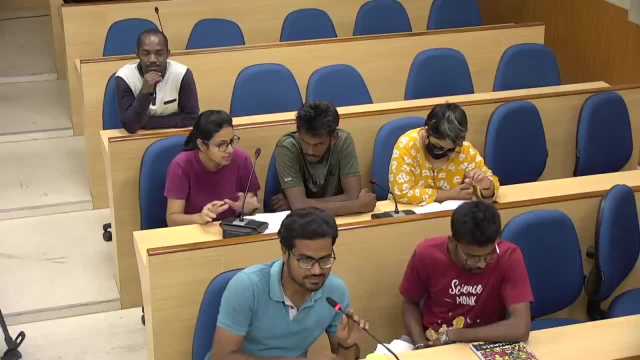 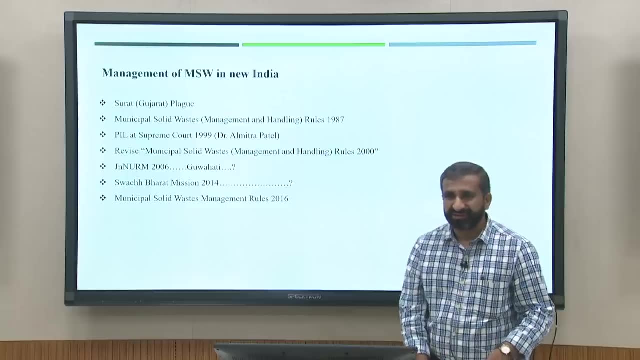 ask me, Sir, when did this hazardous waste got included into municipal solid waste management rules? Yeah, So the now. actually this course is specially for the municipal solid waste management rules. Yeah, So the now. actually this course is specially for the municipal solid waste management rules. 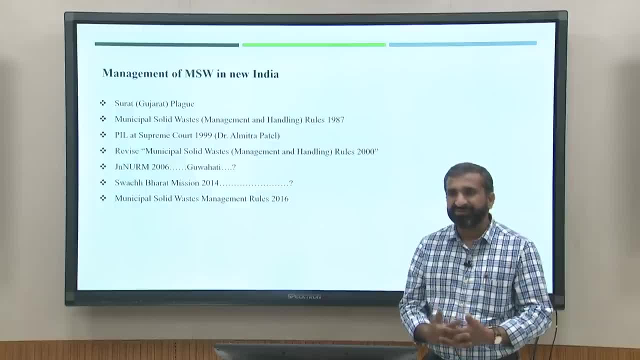 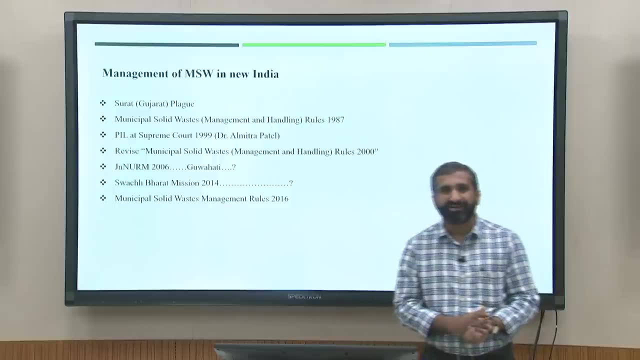 Okay, So this course is specially for the municipal solid waste management rules. Apart from municipal solid waste management, there are number of different waste And in India there are number of rules for that. So hazardous waste also is another, very different course. 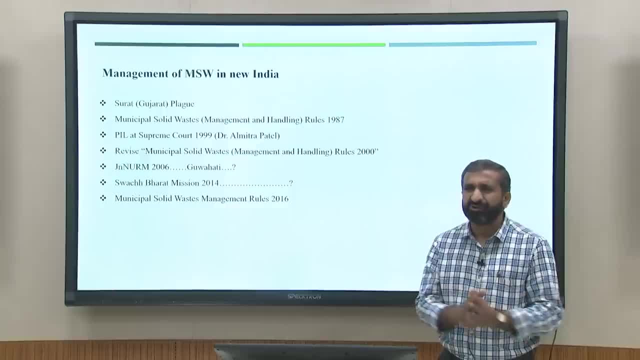 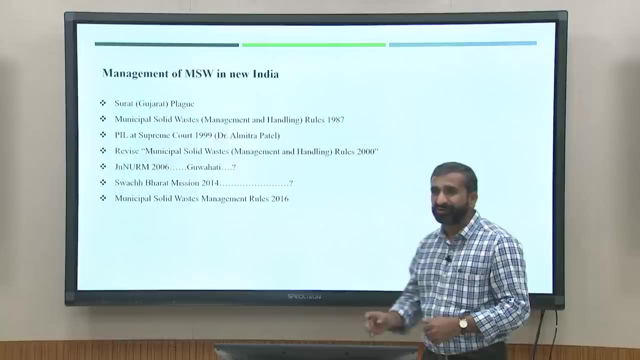 That normally in our municipal area we do not produce hazardous waste management, Although we talked about one source is a household hazardous waste, but that is not that kind of hazardous where normally we include it into the hazardous waste. Okay, So this hazardous waste management rule also has been modified in 2016.. 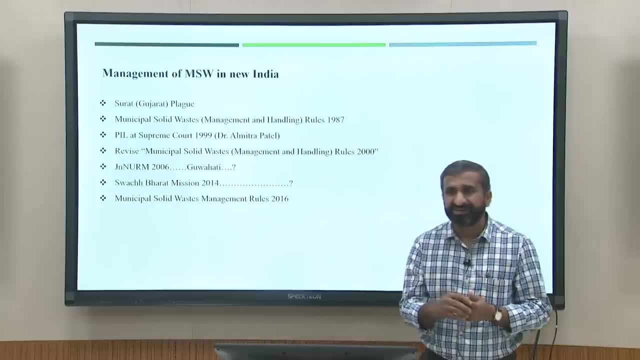 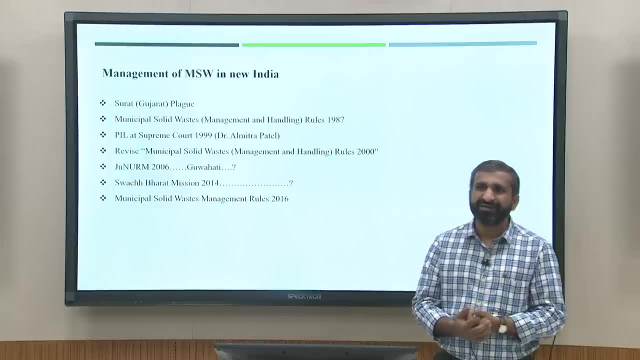 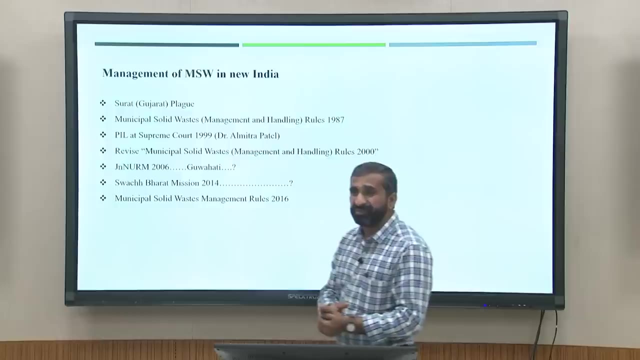 The major sources of hazardous waste management. hazardous waste those are the hospitals or most of the industries are the hazardous waste. So normally ULBs would not manage the hazardous waste management ULB would not do. That is based on the company wise, based on the industry wise. they have to manage their 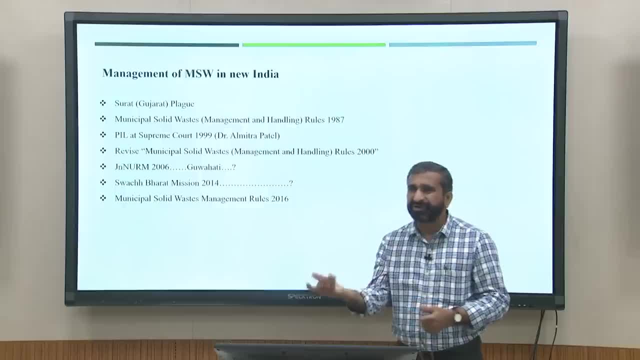 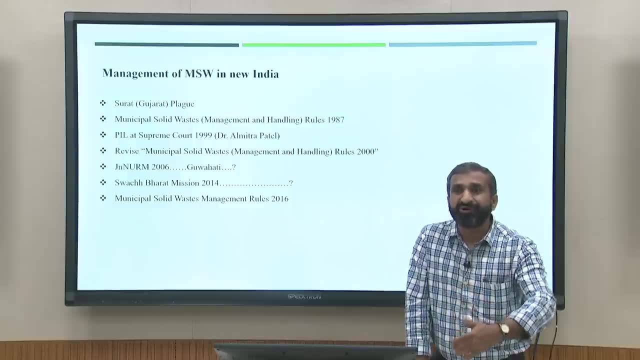 own waste into industry wise, So that is a separate course. hazardous waste management. So, similarly with hazardous waste management, we have rule on plastic waste management. we have rule on e-waste management. India was the first country in 2011,. we had a first. 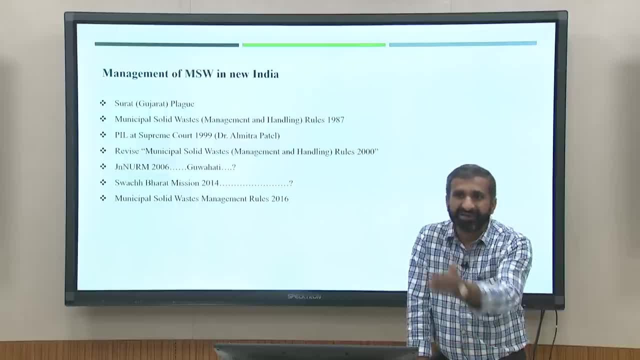 rule, e-waste management rule in 2011,, which got, which got again modified in 2016.. Similarly, we have battery disposal rules, Okay, Okay, So that is a separate rule that is also modified, and even that, that these rules I am talking. 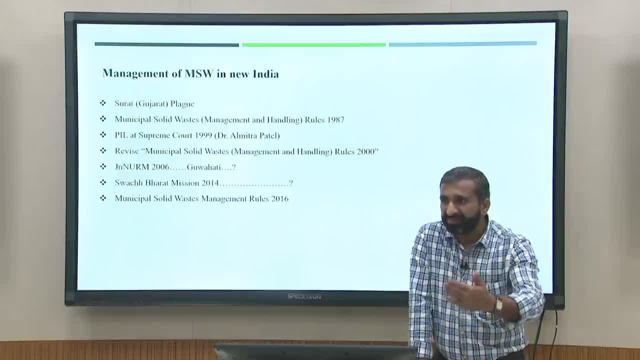 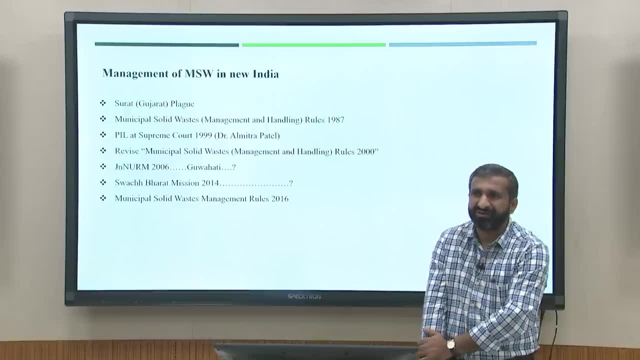 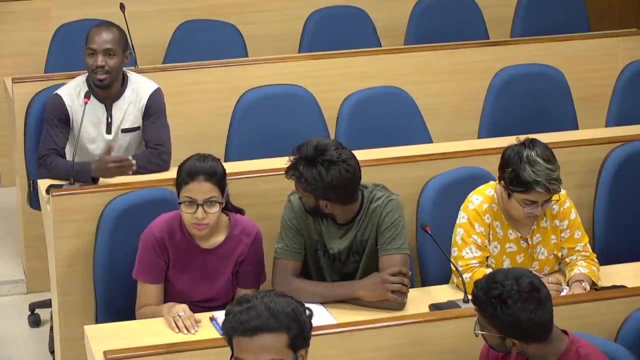 about the country wise, But there are some states. they have also their own rule. So these are the different. different rules are available with us In 2005,. in Mumbai there is a flare was happened. That is not the main problem. 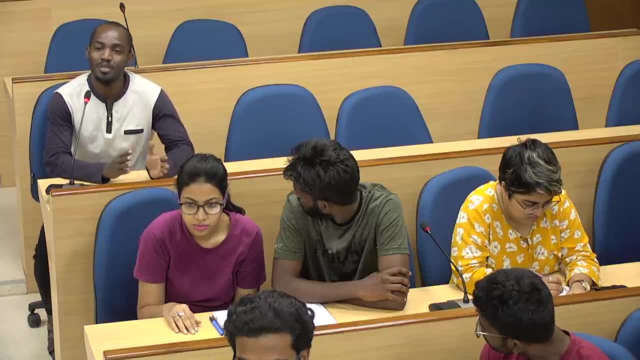 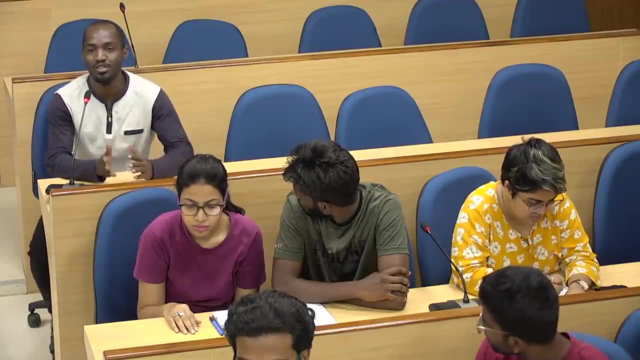 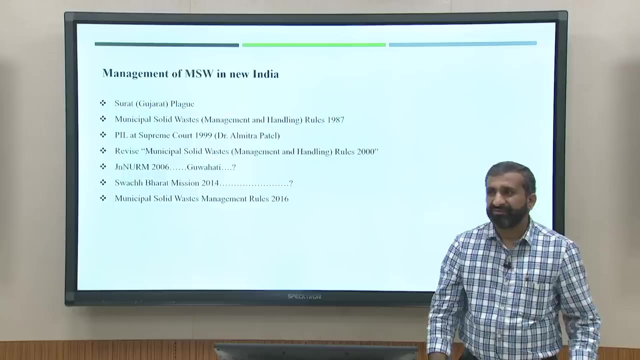 That means it is created with the solid waste. Okay, So the problem is maybe from the awareness of the society. So what can we do on these areas regarding to the authorities, the responsible bodies in the country? wise, what can we do? what can you suggest? 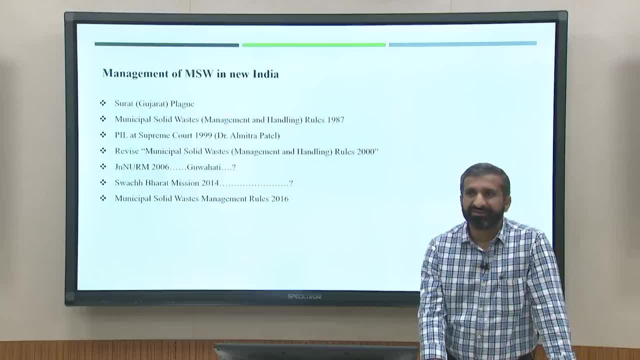 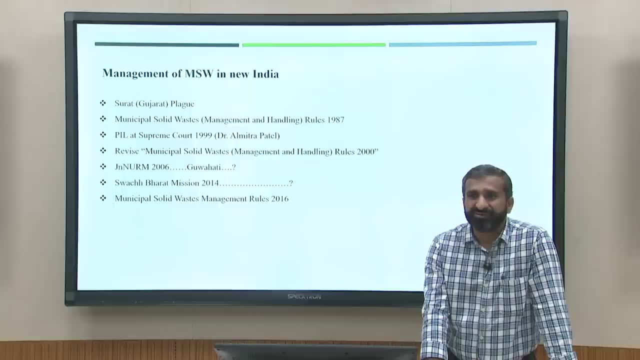 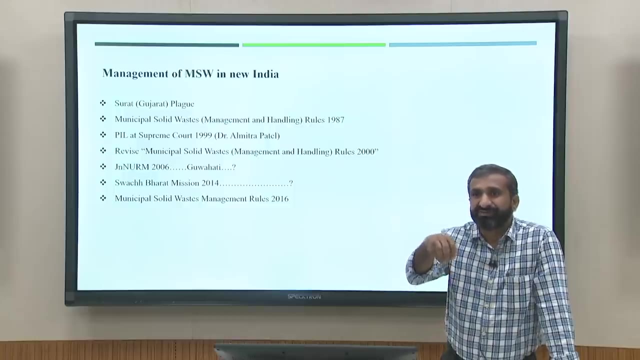 Yeah, So as I talked about that, the flooding in Mumbai was very surprising because the way we are disposing the waste is not only the disposal at dump site, But the way we have the located the dustbin. those dustbins is became a dump site and large. 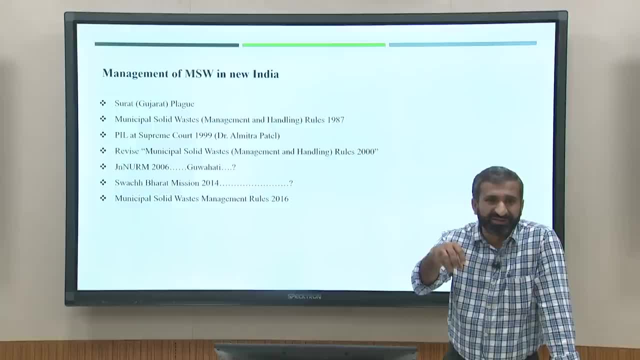 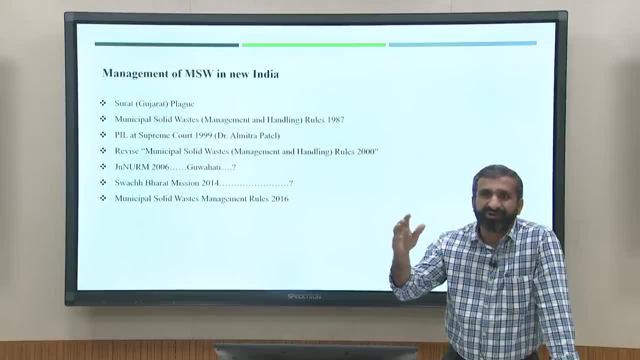 amount of waste is getting accumulated into the, onto the dustbin area, And when in, especially in India, when the rain started, that get continued for four days, five days, for a week And because of that, this plastic, because it is a very light material, that became added. 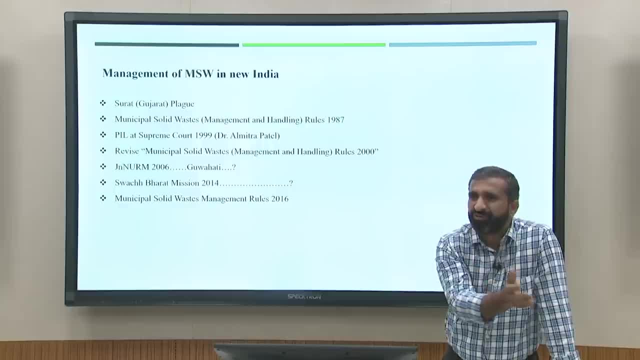 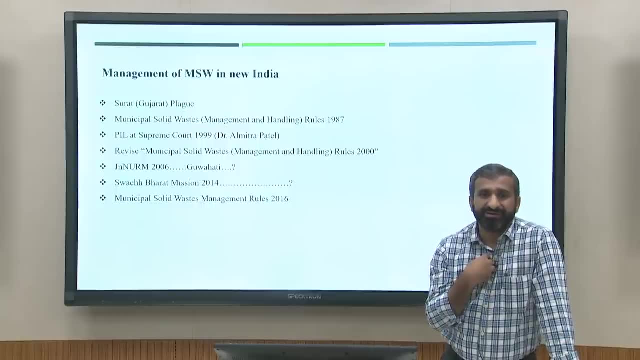 into the that became soluble in the water, Okay, And get flowed with the water and enter into the drain. So what was the problem? Because, see, until before, Swachh Bharat Mission was very difficult to understand by the local people. 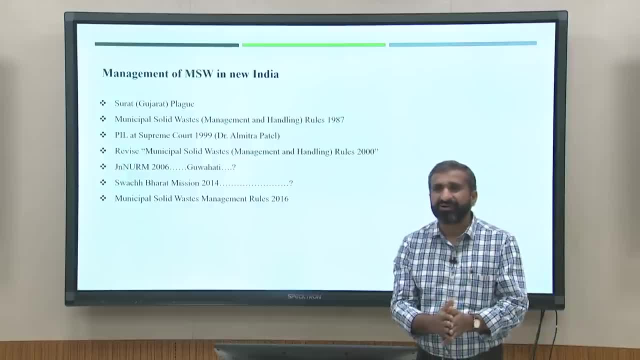 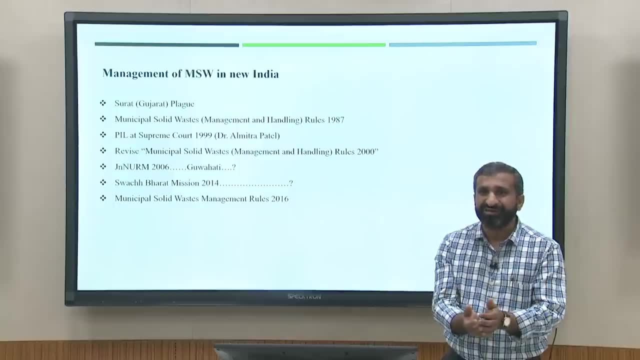 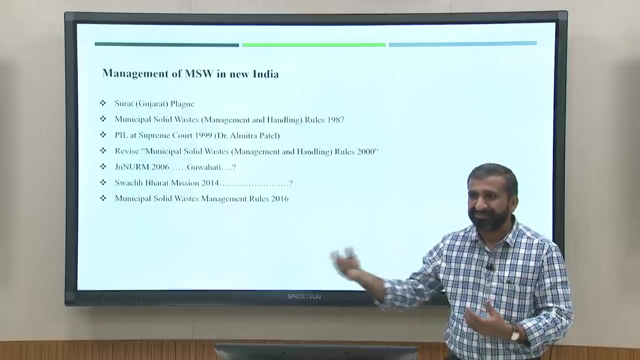 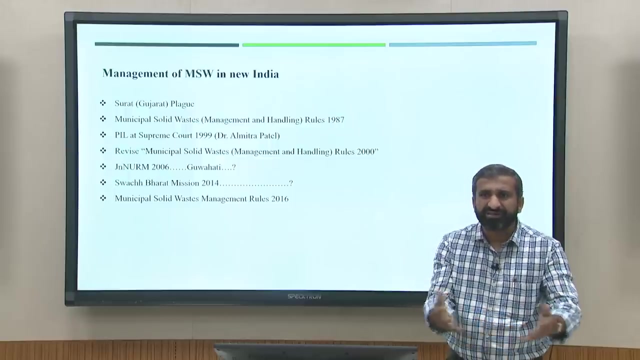 They never thought of. under see in India people were talking about about one NIMBY. we called it NIMBY in my backyard. They were worried about that. I am disposing the waste anywhere. This is not my problem. Swachh Bharat Mission also that that has been proposed. that awareness is very important. 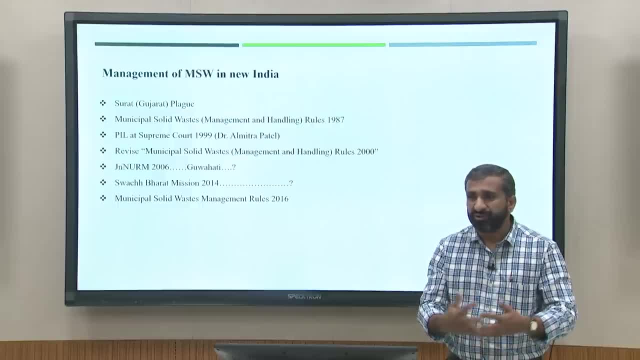 issue now. People has to understand whenever you go for the, any purchase or whatever activity you are organizing, your house has to be understand what kind of waste is getting generated and you need proper collection facility for the waste. That is why I talked about this. 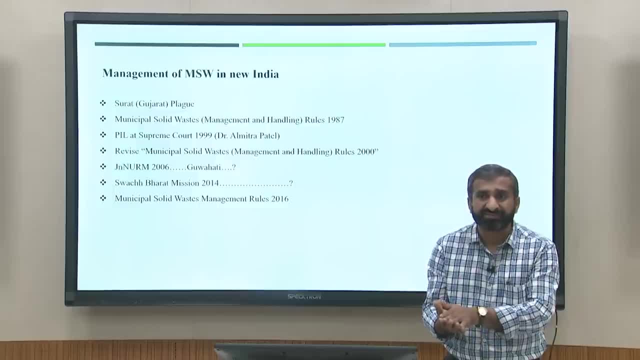 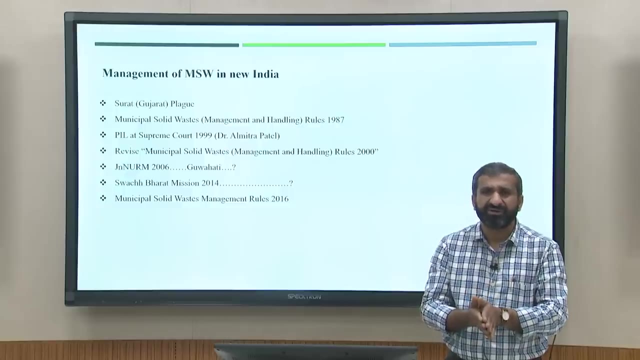 Okay, I talked about that- when you need to have proper waste collection facility- Not only waste collection facility, but also waste treatment facility in nearby area. So lot of awareness, because and was very difficult in India when, when household had been asked to segregated the waste, was highly opposed when this, even in 2006, when JNRM said that. 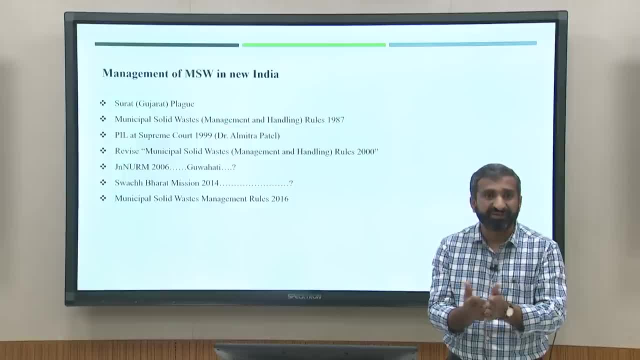 you know you have to have proper waste collection facility. So it is not only waste collection facility but also waste treatment facility in nearby area. So when JNRM scheme has scheme has been proposed of, in during this scheme itself, the house to house collection has been proposed. 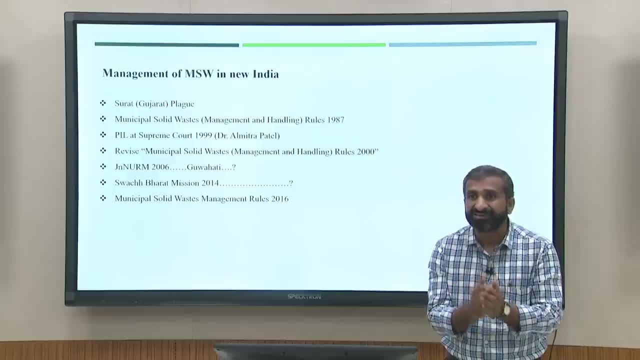 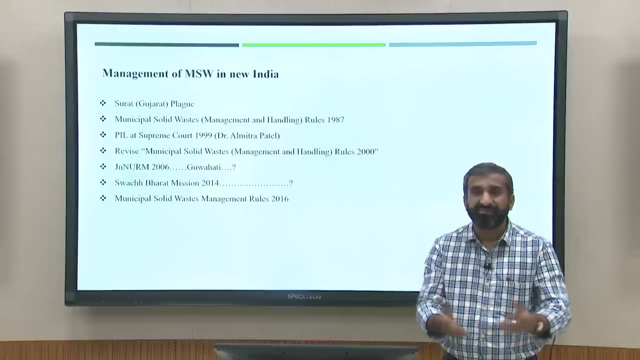 But people were not ready to give the waste. That was very difficult. and forget about the segregated waste. But it is good that under Swachh Bharat Mission most of the city started the segregated waste collection. But again, when you are segregated in the household level, 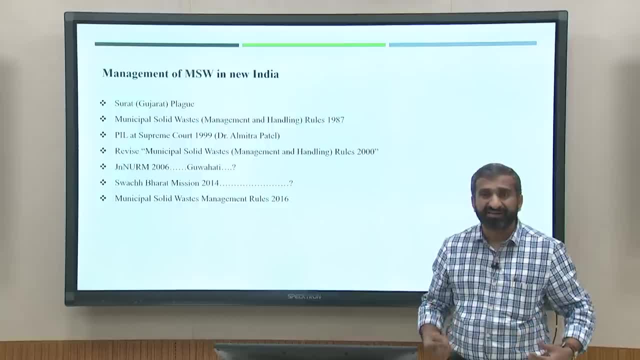 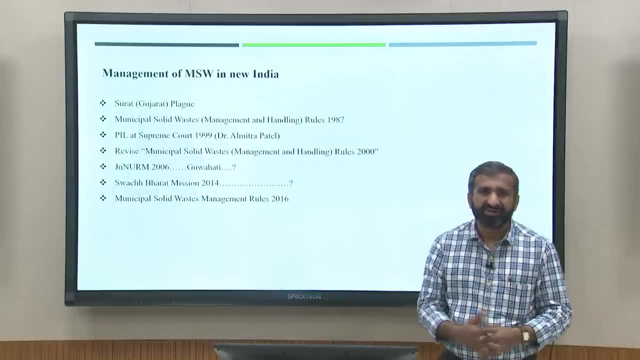 You need to have proper waste collection facility. Okay, You need to have proper segregation: segregated collection facility and segregated treatment facility. That is also one very important issue. that So there is a lot of awareness, but under Swachh Bharat Mission, lot of our Bollywood. 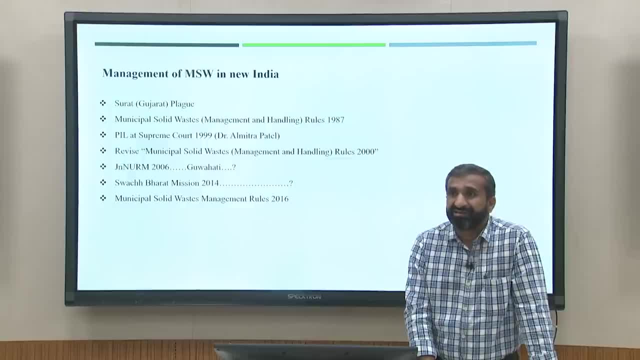 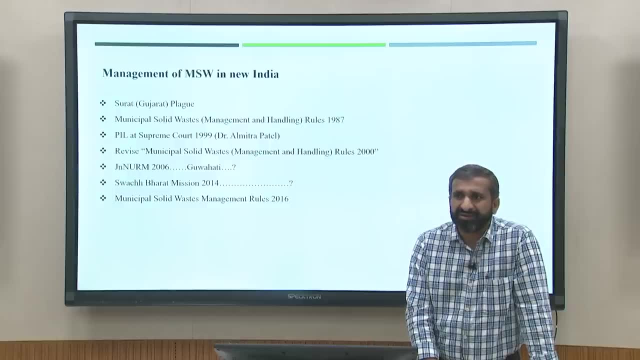 actors also came in, came front and they in lot of media also covered the solid waste management. So people are getting aware now. but again the corporation has to, has to organize lot of awareness program, Specially into the schools, colleges. So obviously I think this course is became very important now and now this is very important. 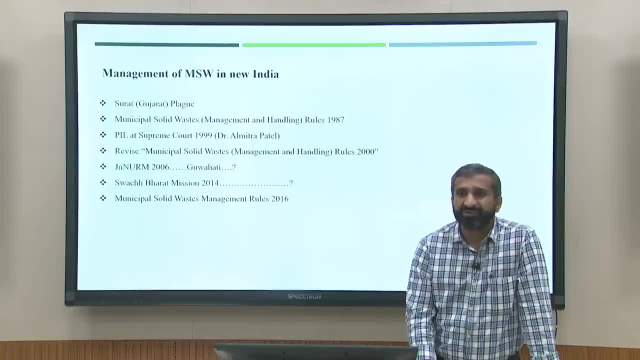 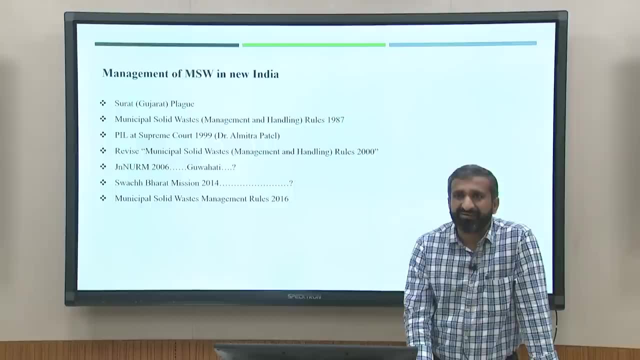 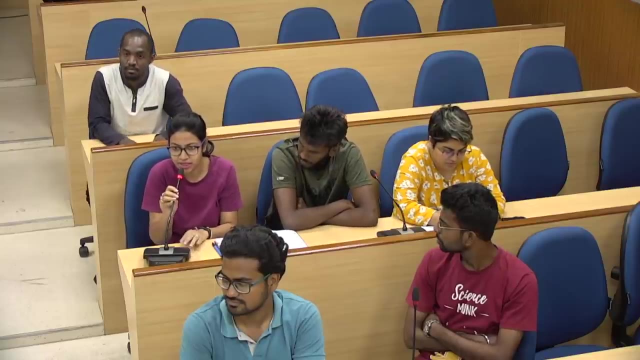 time to understand solid waste management. otherwise, after 20 years, when the waste generation will increase in large quantity, will be very difficult to manage. Hello, sir, sir, there is one question: When we talk about a smart city and a clean city, Yes, Yes, 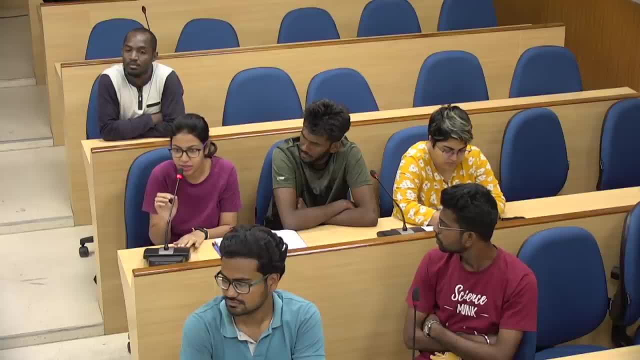 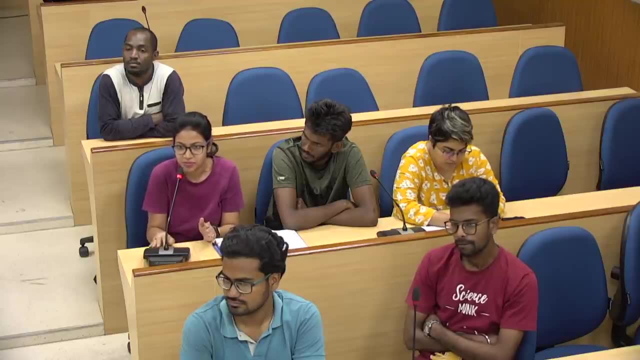 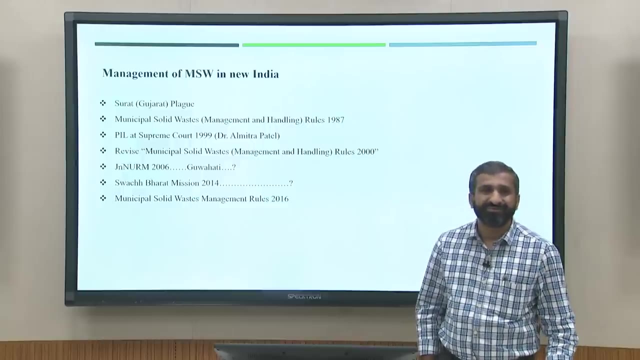 So, in terms of solid waste management, what are the basic characteristics or parameters that we can say which can differentiate a smart city from a clean city? That is also very important one: The clean city and smart city. see, when you say the clean city, that mostly we talked about. 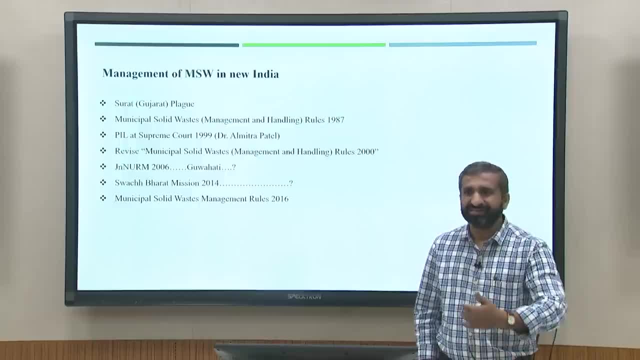 the waste related issue. Waste related issue: waste is getting collect up, but when you call as a smart city, waste is also including into that. Yes, So you need to have proper communication facility, proper transportation facility. that became the smart city. 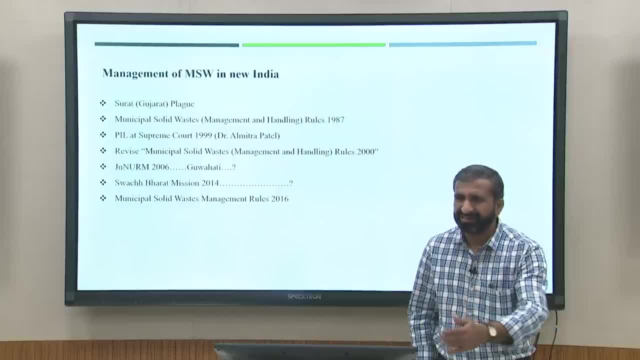 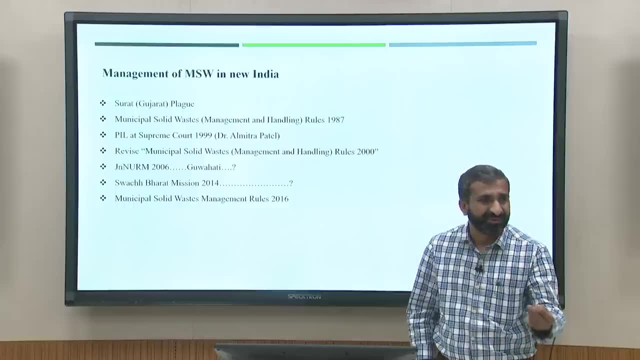 But now I think need not to say the clean city. There is no importance of clean city. now You will be a very clean city, but if you do not have proper communication facility, proper transportation facility, there will not be any benefit of such cities. 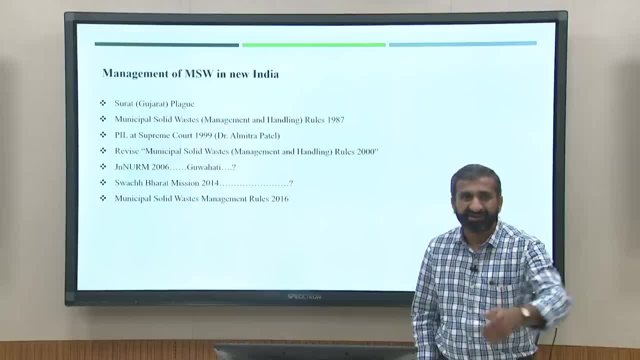 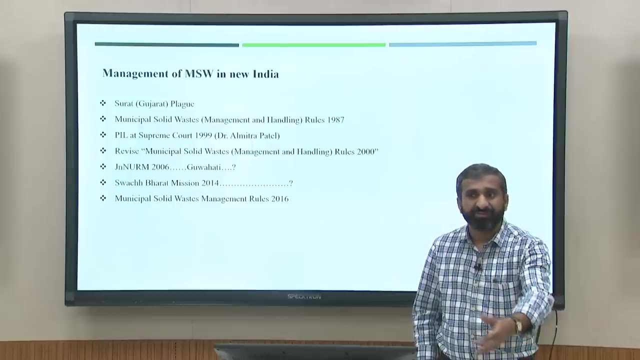 So you need to have- you need to be a become a smart person- or smart city which will have the proper communication, transportation facility- Yes, But also need to have the clean city. So when you say the clean city or the smart city, you need to have proper segregation.